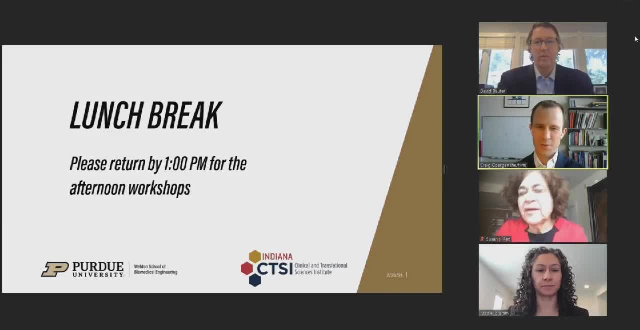 as is. My name is Craig Gorgian. I'm the Leslie A Geddes Associate Professor of Biomedical Engineering here at the Weldon School of Biomedical Engineering at Purdue University. I'm thrilled to co-lead the breakout session today for pediatric regulatory medical devices. 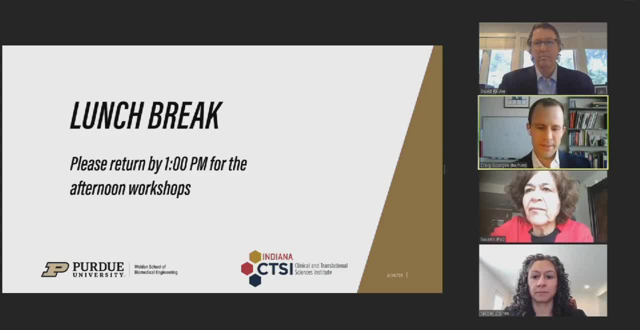 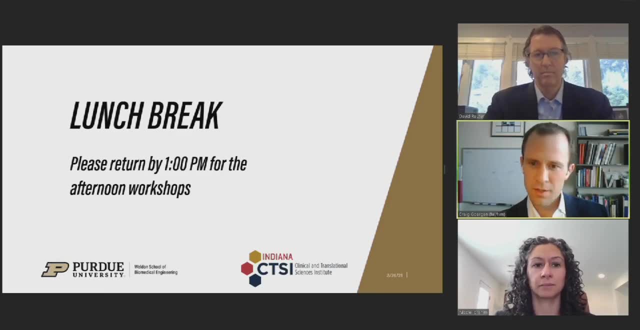 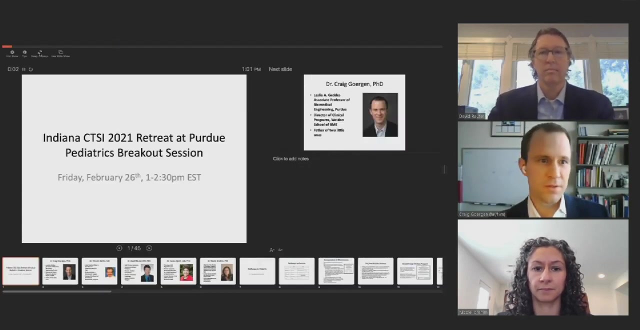 and other issues in relation to pediatric disease. We have a great list of panelists that are going to be participating with us today. I'm going to go ahead and share my screen, and hopefully we can do that quickly. Okay, Let's go ahead and swap displays too. David Reuter, can you see the slide? okay, Does that? 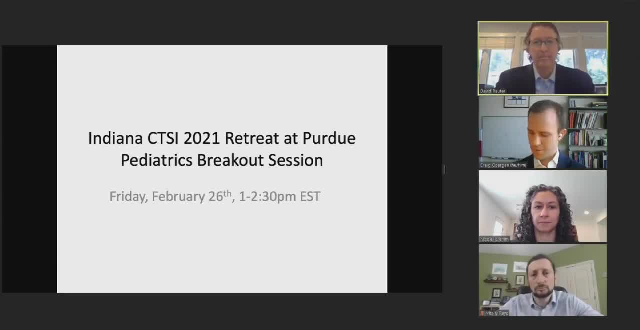 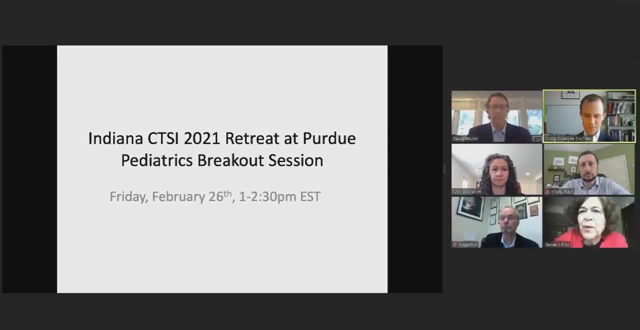 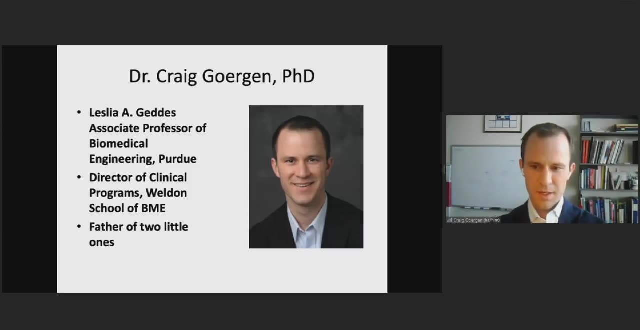 look good to you. It looks great, yes, Fantastic. Thank you, So right. this is the breakout session on pediatric devices. All four of our panelists have experience in pediatrics, either from a device development or regulatory standpoint, or both, And with that I'm thrilled to lead this. I lead a panel of panelists who are going to be 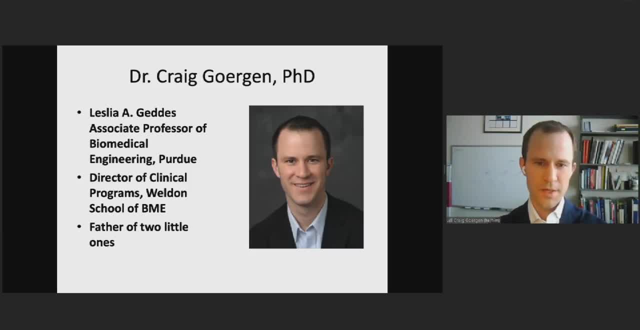 participating in a group of panelists who are going to be attending this webinar, And I'm going to have David Reuter work with me today. David, you have your hand up. Hi, thanks for having me. I'm David Reuter. I'm the Director of the Research Group at Purdue in the 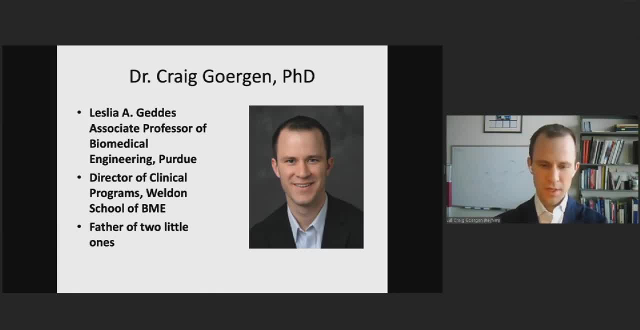 Weldon School. Primarily, I focus on cardiovascular disease. My research interests primarily lie around imaging with high-frequency ultrasound or high-field MRI. We've got a lot of different projects on heart disease and vascular defects, aneurisms and atherosclerosis, But we've also gotten into an interesting project related to reproductive health, vascular health and pediatrics- Developing and trying to develop devices for pediatric populations as well as in prevention. So I'm going to share with you a little bit of that as well. 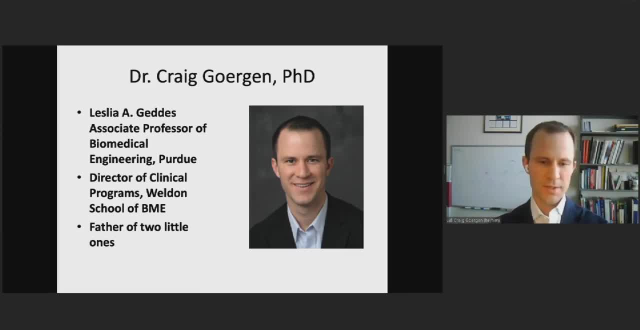 improving our imaging technologies for pediatric patients. Beyond the research efforts, I run the and director of the clinical programs in the Weldon schools. We partner with IU School of Medicine West Lafayette, IU School of Medicine Indianapolis and the other regional campuses around the state. 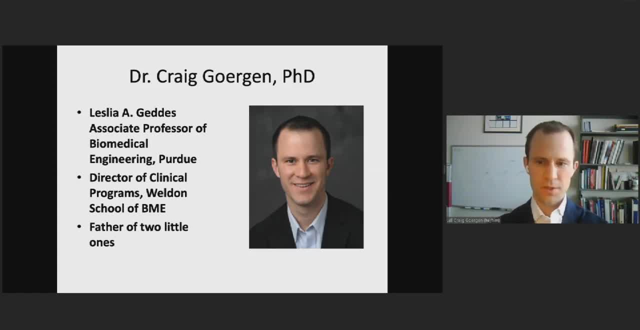 including a scholarly concentrations program for our medical students interested in biomedical engineering. And with that right, pediatrics has become a passion of ours as we're trying to build a consortium. I've got a six and a three-year-old at home that keep us on our toes in the house. 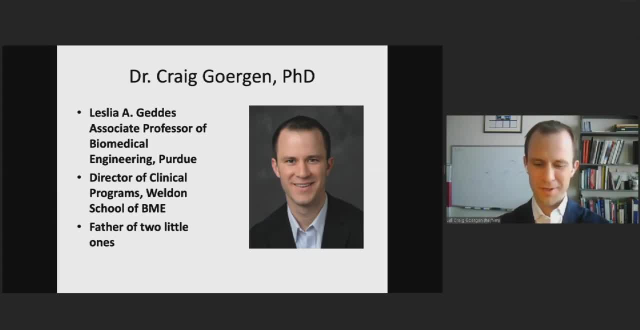 and is really open to my eyes to healthcare not only for mothers that are expecting but for little ones as we try to get them up to the healthy adults. With that, I wanna introduce the panelists, First Dr Vincent Devlin. 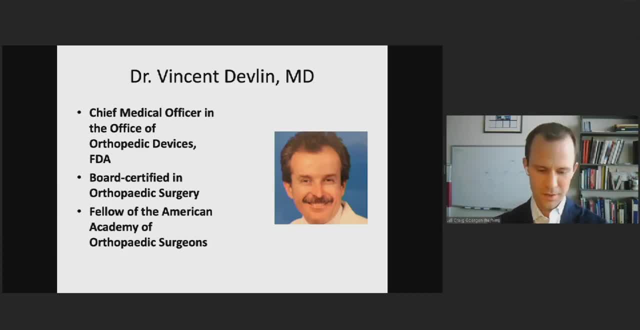 MD is a chief medical officer in the Office of Orthopedics at FDA. Currently serves in the Office of Health and Technology, a six Office of Orthopedic Devices and FDA Center for Devices and Radiological Health. Dr Devlin obtained his undergraduate degree. 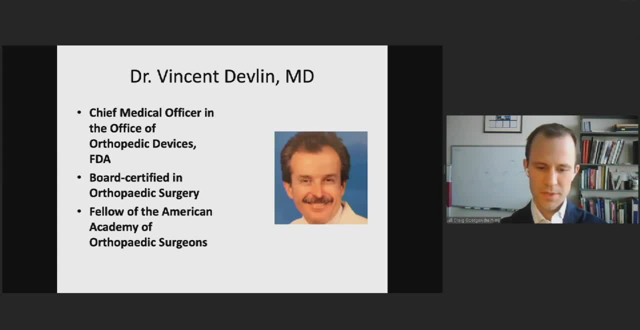 in pre-medical studies from Columbia University and doctor of medicine degree from the State University of New York Downstate Medical Center. Subsequent medical training include an orthopedic residency at the State University of New York Downstate Kings County Medical Center and spine fellowship training. 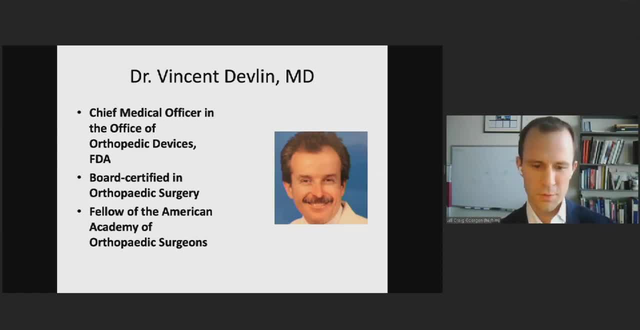 at the University of Minnesota. Dr Devlin is certified by the American Board of Orthopedic Surgery and is a fellow of the American Academy of Orthopedic Surgeons. His clinical practice focused on the diagnosis and treatment of pediatric and adult disorders. 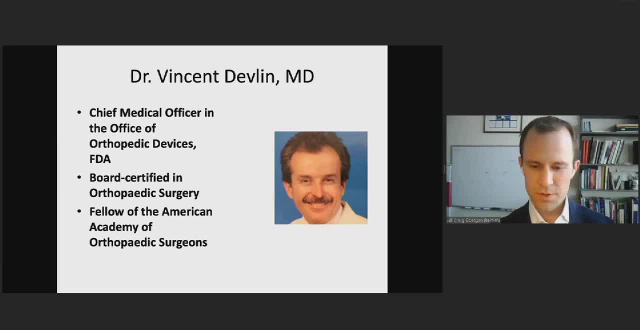 involving the cervical, thoracic and lumbar spine. His research interests include sacropelvic fixation, intraoperative neurophysiological monitoring and orthopedic device registry development. In 2010,, Dr Devlin joined FDA as medical officer, where he's involved in reviews and programs related. 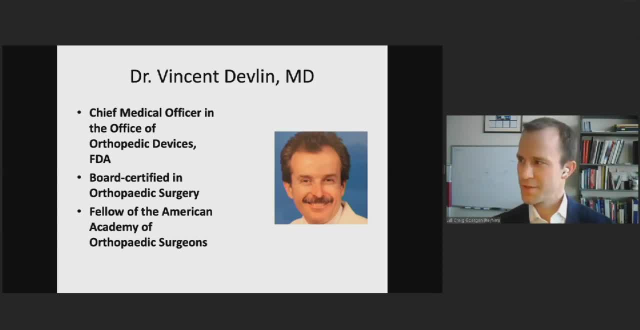 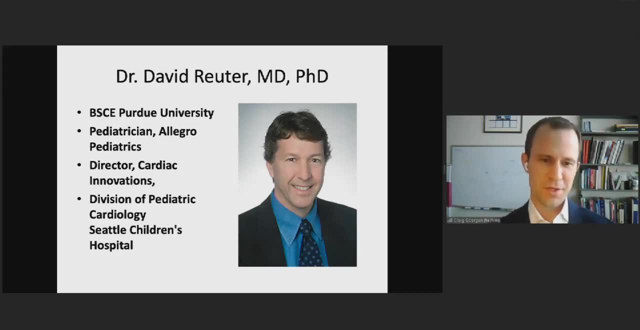 to a wide range of orthopedic devices. Thank you, Dr Devlin, for joining us today. Dr David Reuter is an alum of our program, at least in engineering school, and is a pediatrician out in Seattle. Dr Reuter studied liberal arts. 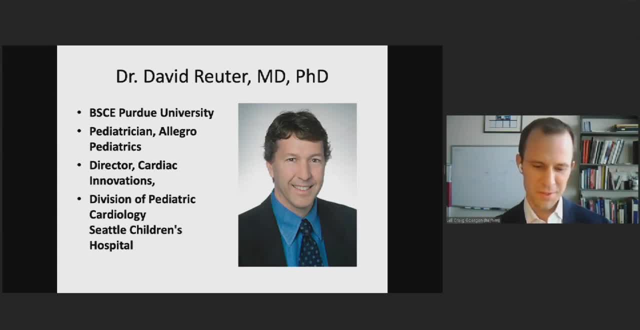 at St Andrew University in Scotland, engineering at Purdue University and received his PhD in bioengineering, also from Purdue. before attending medical school at Indiana University, He completed his pediatric residency at Pittsburgh Children's Hospital. Dr Reuter worked at Seattle Children's Hospital. 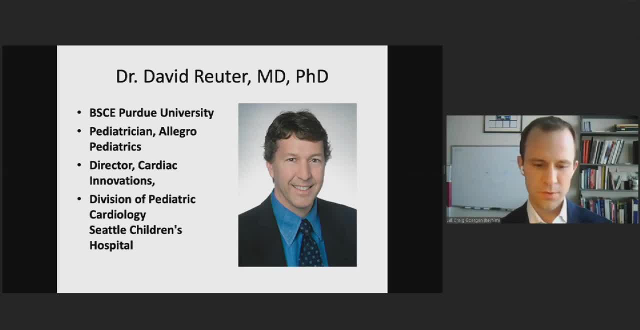 in the emergency department for 15 years before joining Allegra Pediatrics in the fall of 2014.. Dr Reuter is an advocate for improving the lives of children. When he lost a patient to heart disease, he worked for decades to develop a cardiac implant. 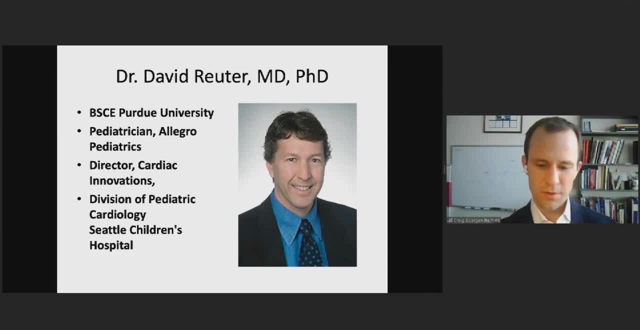 for patients with heart failure. Dr Reuter is currently spearheading a clinical trial in collaboration with Purdue and IU School of Medicine to solve preeclampsia, which is pregnancy associated hypertension. My lab is collaborating with Dr Reuter on that project. 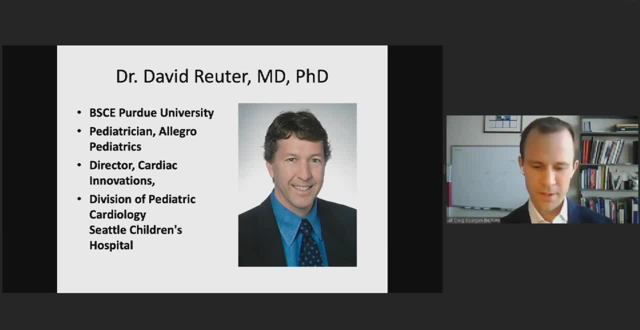 It's been a great success so far and something we've really enjoyed. He also loves caring for kids and feels that partnering with families to help children reach their full potential is a tremendous and rewarding privilege. Dr Reuter, thank you for joining today. 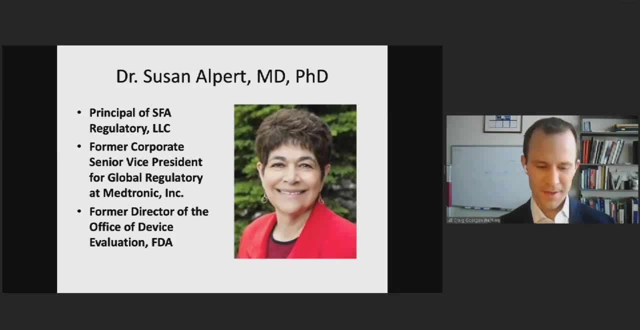 Yep Dr Susan Alpert. She is the Principal Consultant at SFA Regulatory. former Corporate VP at Medtronic Is working currently now at a one-person firm focused on strategies needed to place medical devices and other medical products into the global market. 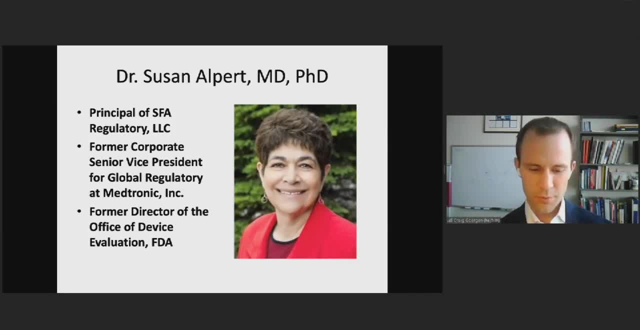 She was a Corporate Senior VP for Global Regulatory at Medtronic Incorporated and, prior to that, the VP of Regulatory Sciences at CR Barr Incorporated. She previously worked at the US FDA, where she held a variety of management positions in the centers for centers dealing. 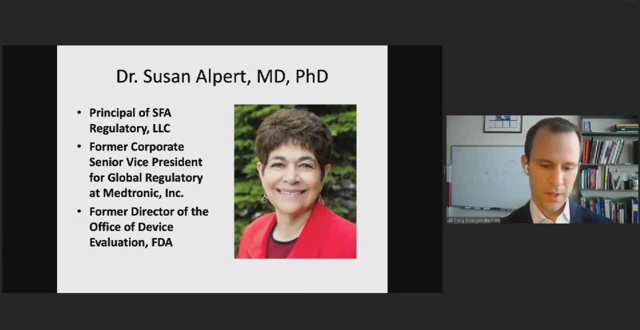 with drug devices and radiological health and foods. She was Director of the Office of Device Evaluation from 1993 to 1999.. Dr Alpert is a microbiologist and pediatrician with a specialty in infectious disease. She completed her undergraduate degree. 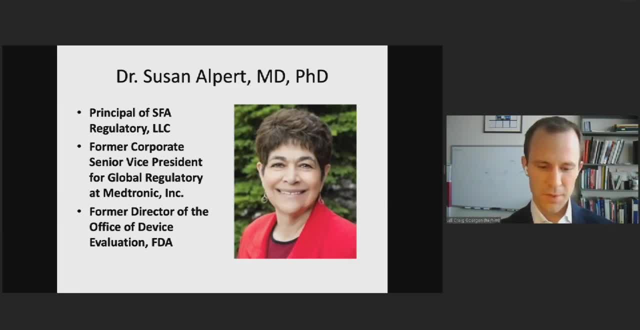 at Barnard College, Columbia University in New York City, holds a Master's degree and PhD in Biomedical Sciences from NYU and a medical degree from the University of Miami, Florida. She's a member of several nonprofit and for-profit boards. So, Dr Alpert, thank you very much for joining. 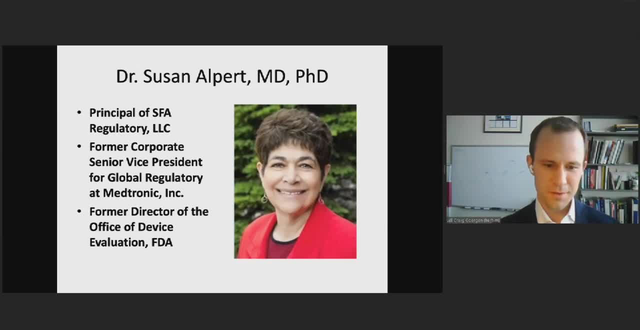 Then finally, Dr Nicole Ibrahim. you can see from the slide here she's the Director of the Division of Circulatory Support, Structural and Vascular Devices in the Office of Cardiovascular Devices at the FDA, where she provides regulatory oversight for pre and post-market activities. 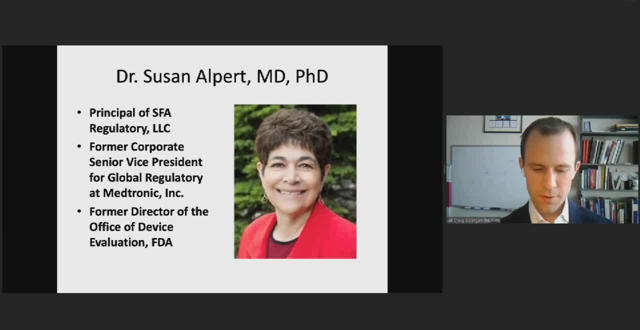 for medical devices in her division, She's involved in several internal and external efforts to promote pediatric device development for cardiovascular applications. She joined the FDA in 2009 as a pre-market reviewer in the Division of Cardiovascular Devices and served as the Branch Chief. 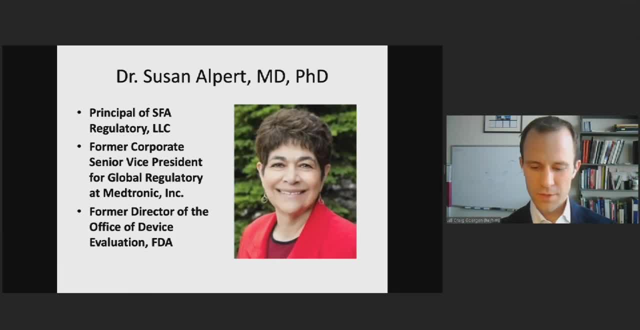 for the Structural Heart Devices Branch, where her work as Branch Chief included oversight of products such as heart valve repair and replacement devices, occluders and pediatric structural heart devices. Prior to FDA, she received her BS in Bioengineering from Rice University in Texas. 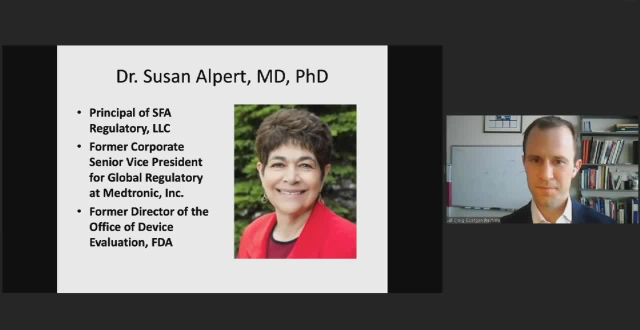 and her PhD in Bioengineering from the University of Pennsylvania in Philadelphia. Dr Ibrahim, thank you for joining as well. So with that, instead of just jumping right into discussion, we actually I asked all the panelists to put together a few example case studies. 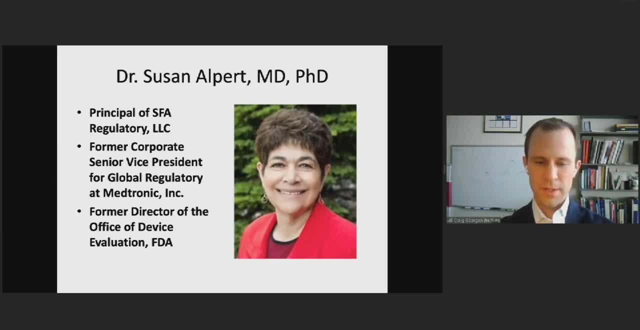 and main takeaway points from their experience that they wanted to cover first. So Dr Ibrahim is gonna go first. I'm gonna try to advance the slides when she tells me to All four of our panelists have prepared about 10 minutes worth of content. 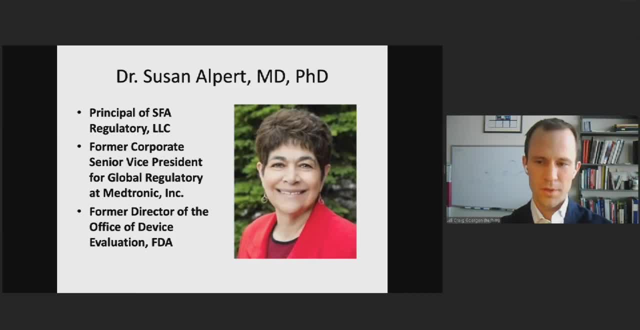 And then the rest of the time. we really wanna make this as interactive as possible, So if we could work with everybody that's participating today. please put your questions in the chat and then ask as well if you'd like to have your line unmuted and your video on. 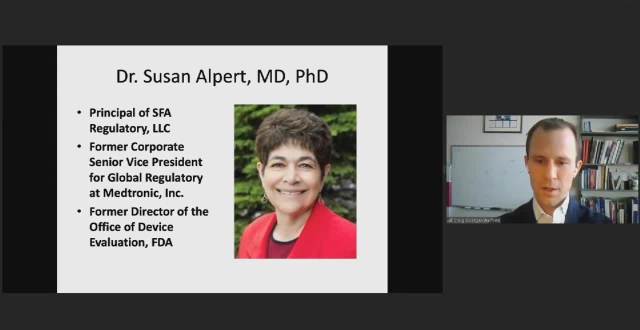 you can ask questions that make a real discussion of this, so that we can delve into what regulatory consideration should be made for pediatric devices that are different from adults. So with that, Dr Ibrahim, I'll go to your first slide and you can take it from here. 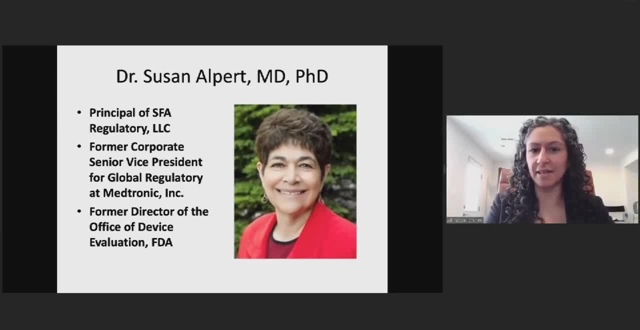 Great, thank you. I don't see the first slide. The slide that I see still says Dr Susan Alpert, Dr Susan Alpert, Dr Susan Alpert. So that's the one I'm gonna go to. We already have a little bit of time. 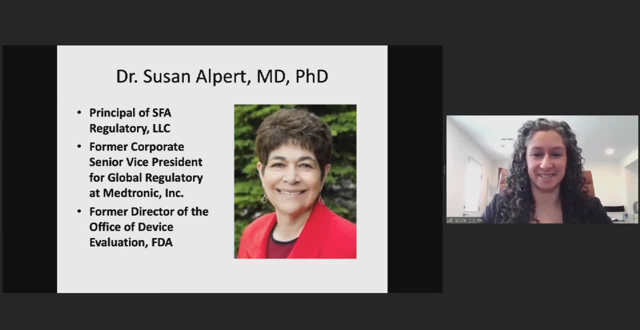 but I'm gonna go back to the floor. So, if you just wanna talk a little bit about what you just talked about and what you'd like to share about the support that you use, in terms of the support that you're getting from each of the organizations that are here today, 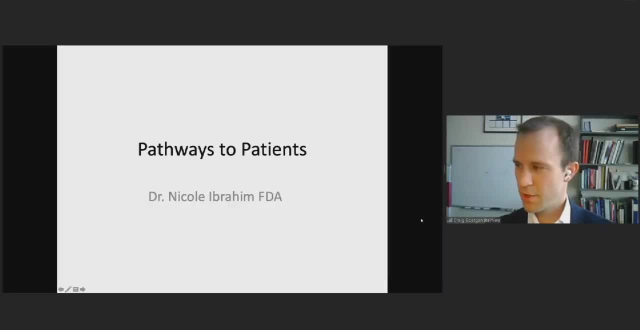 and how you react to some of this. Dr Susan Alpert, I'm not sure if I got the first slide. Even this is probably one. I'm not sure. if I'm not sure if I'm not trying to help you right now. 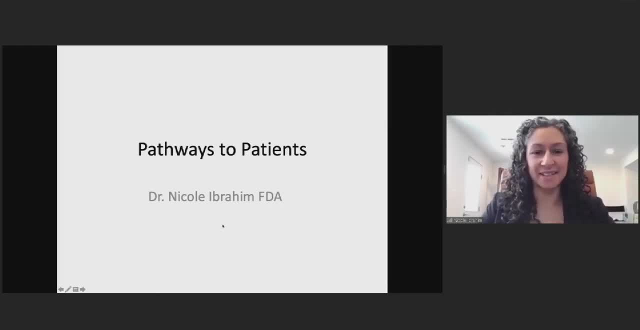 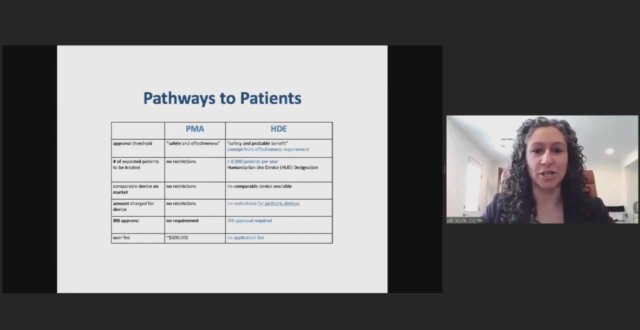 Dr Susan Alpert. That's, I think, the first slide, Dr Susan Alpert. Okay, sorry, Dr Susan Alpert. Last question I was gonna say to our panelists workshop for inviting me. The content that I've prepared here is not necessarily intended to be. 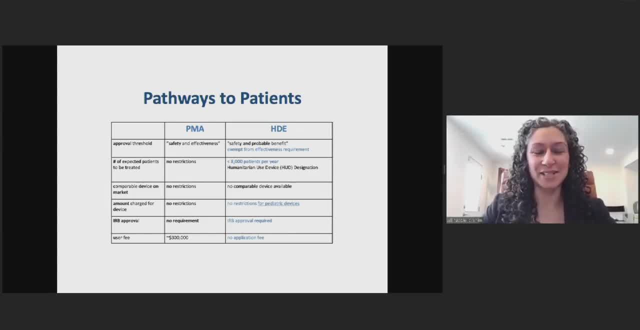 a cohesive presentation per se, but in our prior discussions, as the members of the panel, we discussed, maybe highlighting some areas in the regulatory framework that have been either established or are intended to really promote and help encourage pediatric device development. So the slides I have here kind of describe a couple of different regulatory programs and aspects. 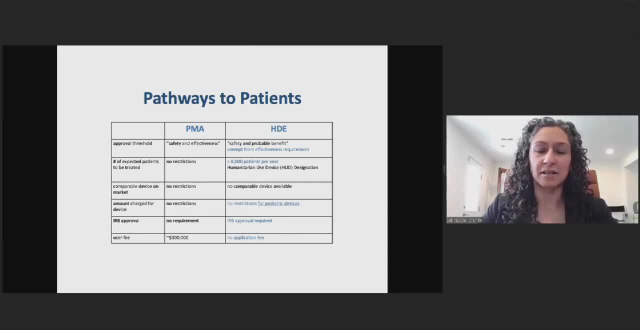 that are currently in play that the FDA is using to try to help get some of these devices to market for pediatric patients. So the first one that I wanted to highlight is the HDE program, which is the Humanitarian Device Exemption Program, And it's a little bit different from the traditional 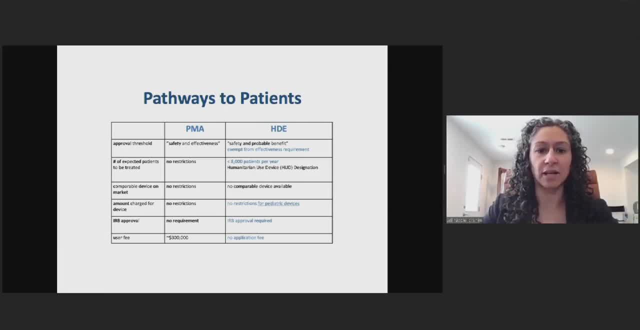 pre-market approval pathway, And so I've provided a table here that kind of shows a comparison between those two programs. So the statutory bar for approval for a PMA device, or Class III PMA, is to establish safety and effectiveness of the device, whereas for HDE the bar is really safety and probable benefit, And that's to say that the 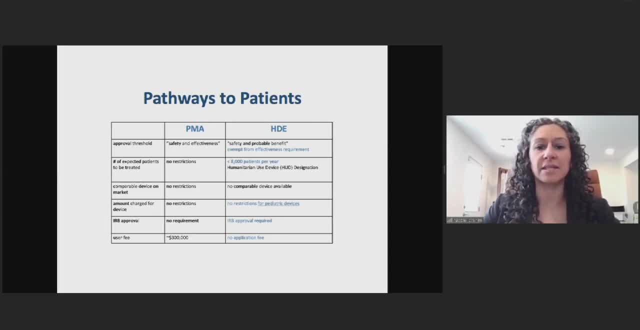 device is exempt from the effectiveness requirement but still has to demonstrate some degree of benefit in order to reach the market. There are also restrictions related to the number of patients that can be treated under an HDE. So for a PMA there are no restrictions, But humanitarian device exemption is really limited to. 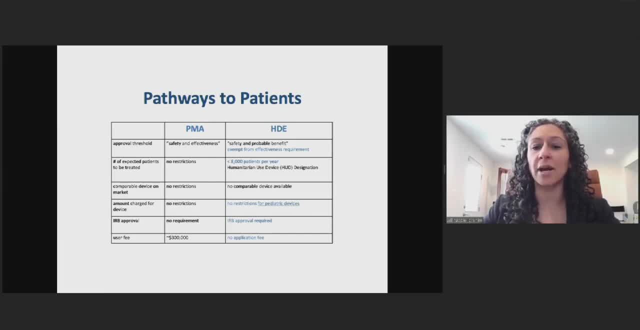 devices that are going to treat less than 8,000 patients per year, And prior to pursuing an HDE as a marketing application or marketing submission, a company would need to apply for what's called a humanitarian use device designation or a HUD designation. 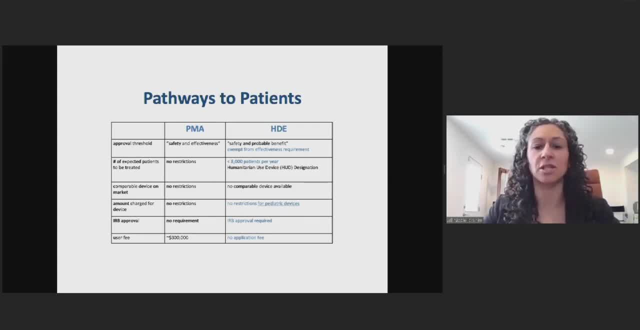 And they have to submit documentation and analysis and evaluation that shows, based on either epidemiology or literature, that the disease or condition that they're going to treat with the device affects less than 8,000 patients per year. For a PMA there are no. 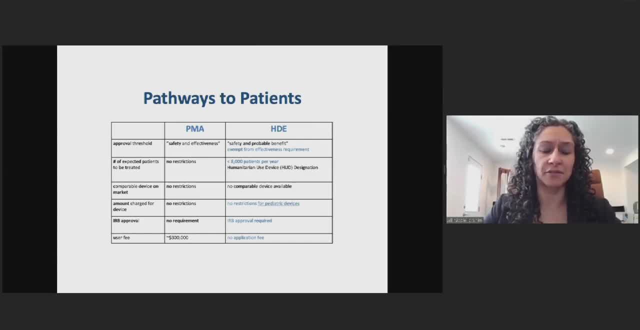 restrictions in terms of comparability of devices on the market. So we might have 10 PMAs for drug-eluting stents, And so a drug-eluting stent would not qualify for an HDE, because the HDE program is really centered on devices for which there's no comparable or available alternative. 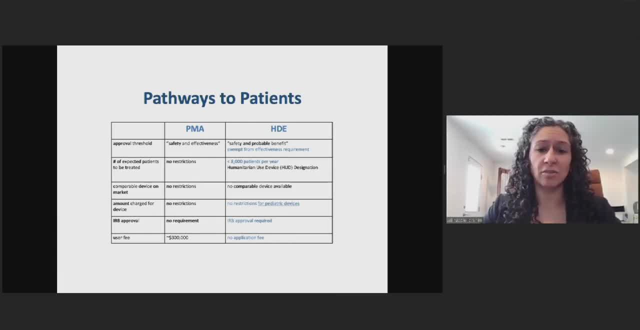 The restrictions. there are restrictions that are placed on HDE devices for the amount that a company can charge. Under the PMA program there's no restriction, but for HDEs in general there were restrictions on the amount that the company or the profit that could consume. 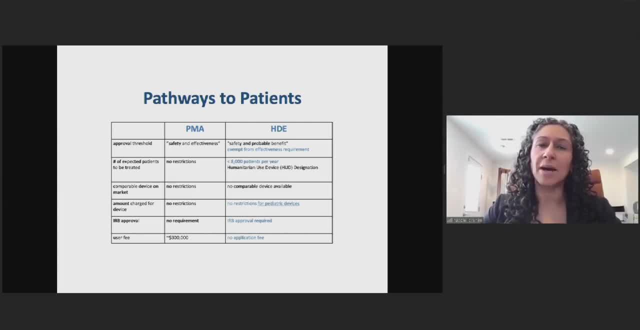 be made for a particular device. about 10 plus years ago- more than 10 years ago now- they listed the restrictions for pediatric devices, and so now there are currently no restrictions under the hte pathway for pediatric devices. another requirement for hte devices is that, in order to use them, a 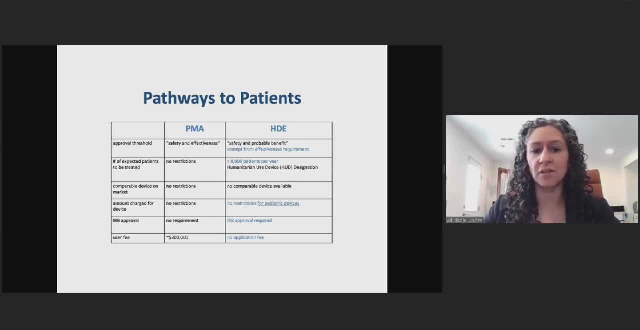 physician needs to obtain irb approval from their institution. this is a fairly unique requirement because i think it can sometimes create some degree of hurdle in gaining access to a device, but because the the requirement for effectiveness has been lifted, input from the irb and approval from the irb was sort of established as a way to mitigate that particular issue. and then the last: 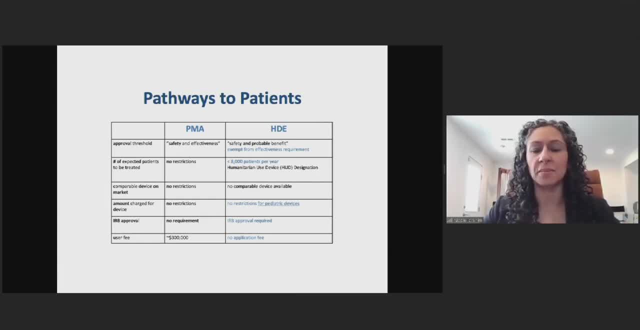 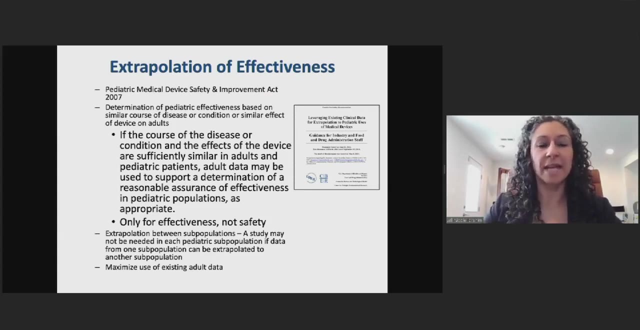 thing is the user fees. so pmas have a user fee associated with them, but hdes are a free application- next slide. so that's kind of a basic framework of application types that could apply for pediatric devices, at least in the class 3 realm. there have been a number of guidance documents that have been 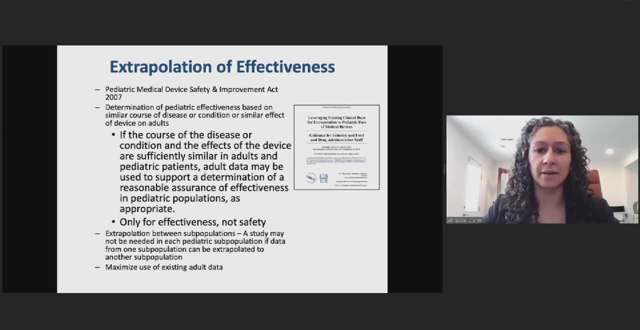 put out by the fda to try to promote again pediatric device development and on-label use of pediatric devices, and so one of the areas back in 2000, 2015 or 16 that was established was this concept of extrapolation of effectiveness, and so it's. 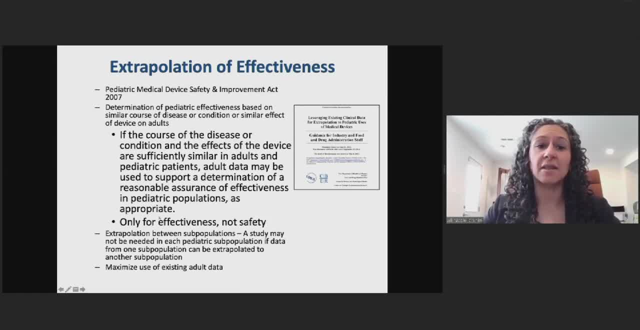 basically a determination of pediatric effectiveness that's based on a similar course of disease or condition that exists for the device in adults. so you can imagine that if there's a device on the market that was developed and approved for for adults, there may be a- you know, a cohort of data. 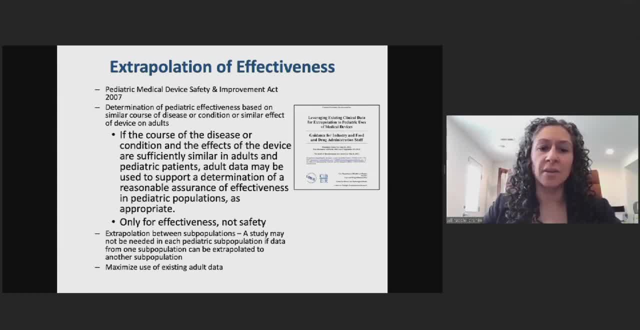 or volume of data that supports the use in adults, if that device were one, were to be sought for a pediatric indication, that the concept of extrapolation of effectiveness is essentially to utilize some of the adult data to support a pediatric indication. and so, if the disease course is really similar between adults and pediatrics and we think that the effectiveness 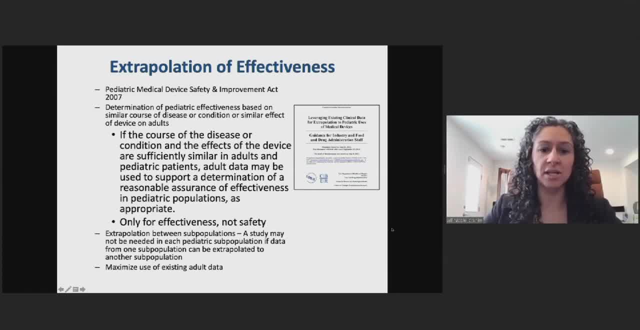 is leverageable and is applicable to the pediatric use, then we can use it to as a means of establishing effectiveness for pediatrics. I will note that this doesn't apply necessarily to safety, So if FDA feels that there are different risks or different adverse events that might be observed in a pediatric population, 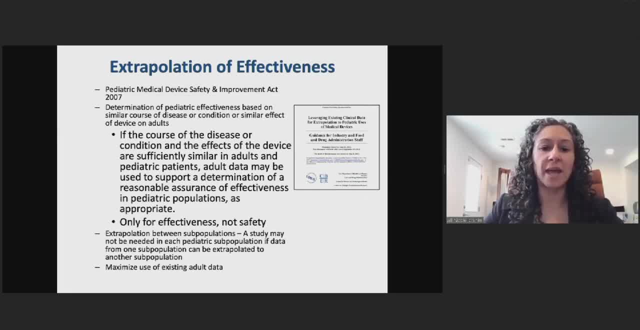 that we might not expect in an adult population. we may ask for an additional supplemental cohort of data that establishes the safety element in pediatrics, And so this, I think, is something that I've seen used over the last few years in order to support a few applications. 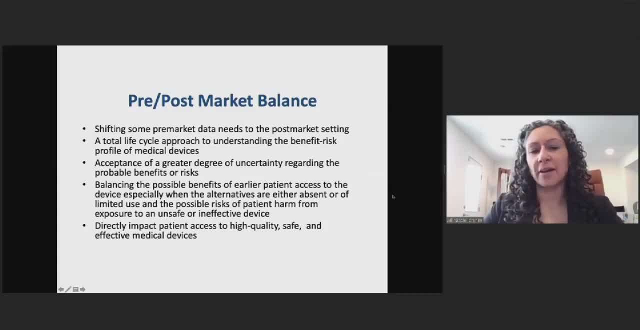 Next slide. The other program area that I think has really, I think, become more robust and stronger over the years is this concept of pre- and post-market balance, where we've established this paradigm of the potential for shifting some pre-market data needs into the post-market. 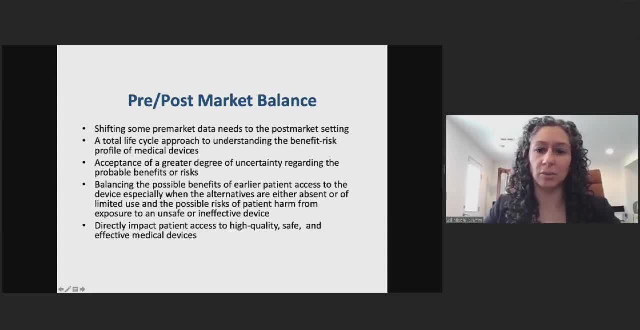 And it's really aimed at looking at a total lifecycle approach to understanding the benefit-risk profile of devices, And so it essentially relies on this concept that we might be able to accept a greater degree of uncertainty for probable benefits or risks, And that's really balanced by the benefit of having earlier access to a particular device. 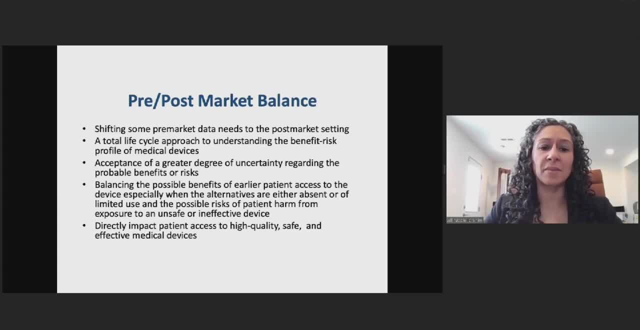 because either there are no alternatives available or maybe there's limited use, And so this shift in the balance between pre- and post-market, I think, is a really important concept, particularly for pediatrics, And it has in recent years resulted in pediatric patients, I think. 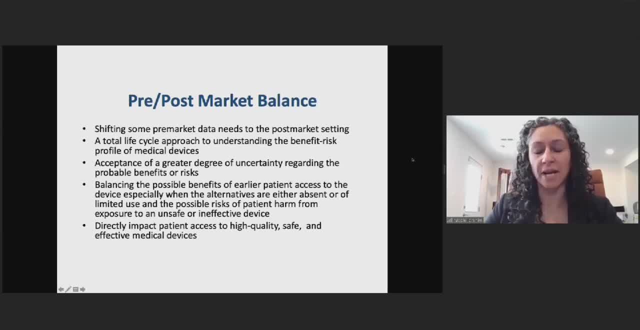 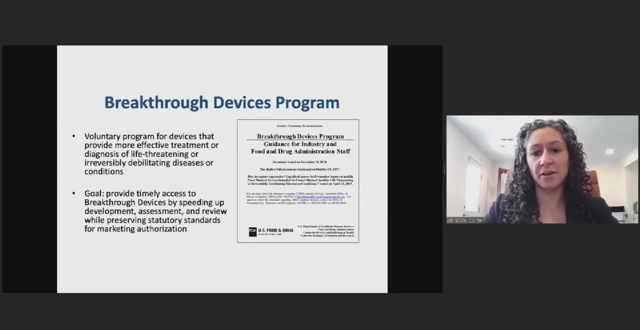 gaining access to devices that might otherwise not have reached the market if it hadn't been for careful thinking through that pre-post-market balance. Next slide, The Breakthrough Devices Program, is another one that I think FDA has increasingly utilized over the last few years to help encourage pediatric device development. 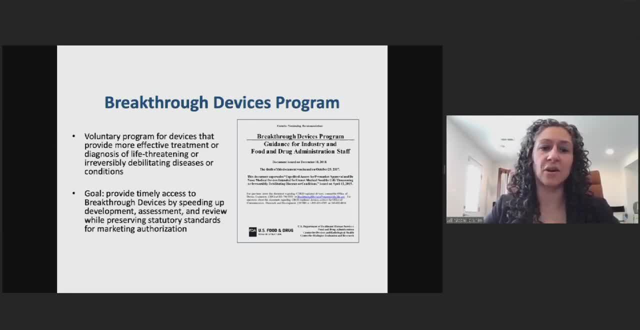 So the Breakthrough Devices Program, if you aren't familiar with it, it's a voluntary program for devices that allows for a designation of a device when it provides for more effective treatment or diagnosis of a life-threatening disease, And it also helps toη¿ fee group units that might not have access to it to as well. 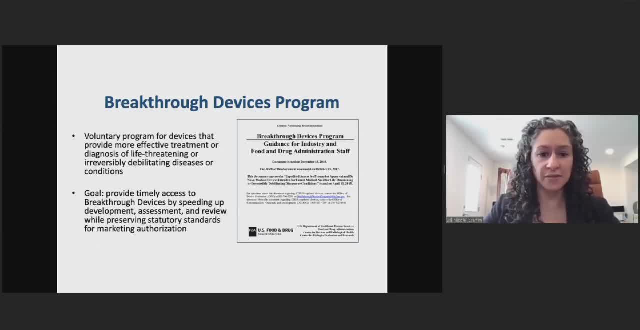 And then there's the same programs that we've decided to follow when we help Yarblo organizing Artemid. So that would be, I think, a waste of what we it has a major role in what's happening with digital companies and reaching settlement for events. 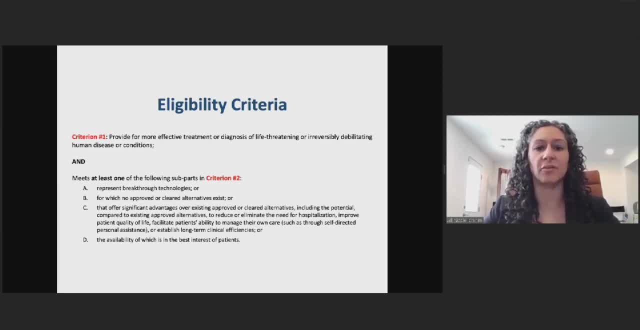 that we should be able to participate in. But our goal is to be able to continue knowing some things that may образ or irreversibly debilitating disease or condition And, like I said, the goal is guy to try to increase access and timely ackess. 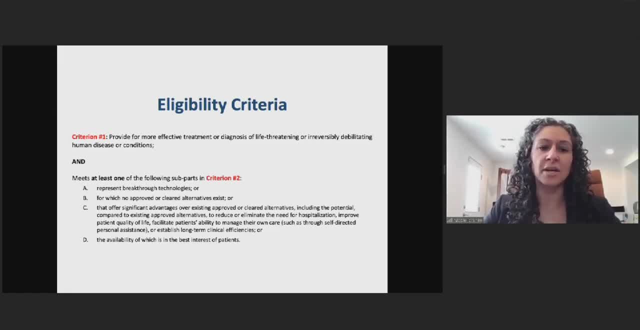 is around this concept of a novel technology. So does it represent a breakthrough in technology for that particular patient population or indication? Are there no approved alternatives that exist? It might offer significant advantages over existing alternatives, or it might just be in the best interest of patients. 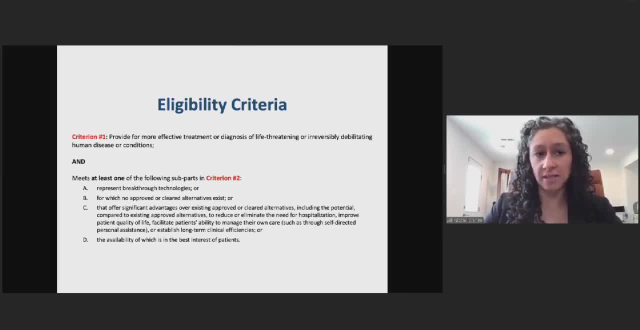 And I would say there are a number of pediatric devices that are in development, at least in the cardiovascular space, that have received a breakthrough designation in the last few years. I will note that the breakthrough program applies to PMA devices, 510K devices and de novo devices. 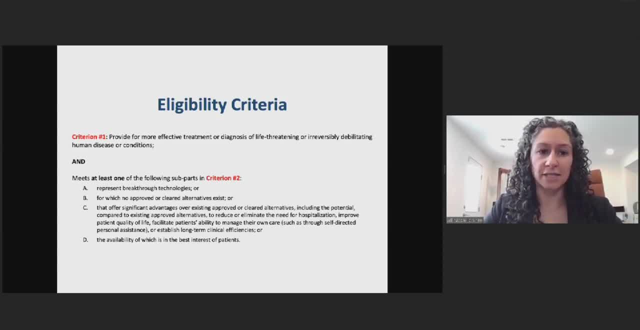 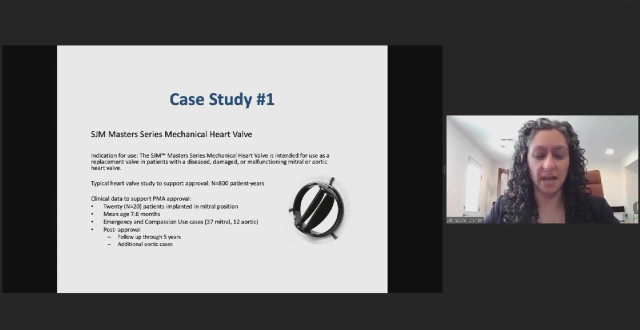 But right now the program doesn't allow for designation for HDE devices, So that's a distinction that I think is relevant to this particular area. Next slide. So I I put on here a couple of case studies that I thought were illustrative of devices. 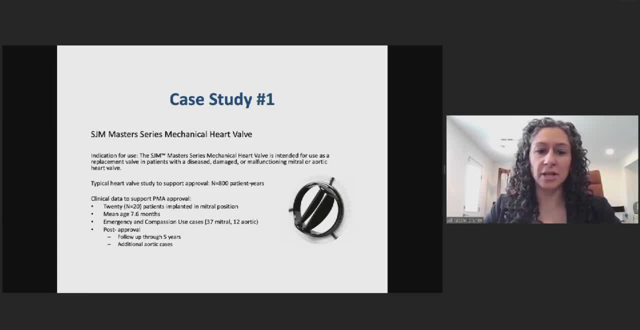 pediatric devices that were commercialized, based on data that incorporated some of the concepts and some of the programs that I just spoke about. So and I'm from the Division of Circulatory Support, Structural and Vascular Devices in Cardiovascular, And so all of my examples are cardiovascular. 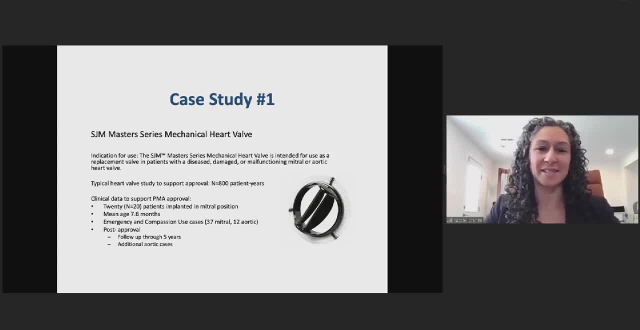 So I'll apologize in advance, but I think there are some lessons learned that are significant And I think they're still applicable across the spectrum. So the first case study is the St Jude, or now Abbott, Master Series Mechanical Heart Valve, And this valve has been around for decades and is sort of the staple in mechanical heart valves. 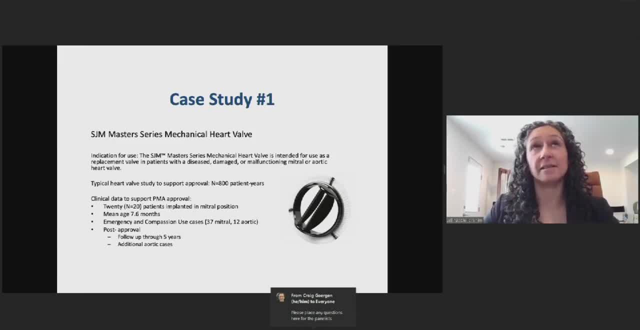 But it was largely developed for and developed and studied in adults because of the larger sizes that were available, And it wasn't until about a decade ago that development of a smaller device that could be implanted in neonates was developed. And so the question that kind of came up is: well, how do we gather the data? 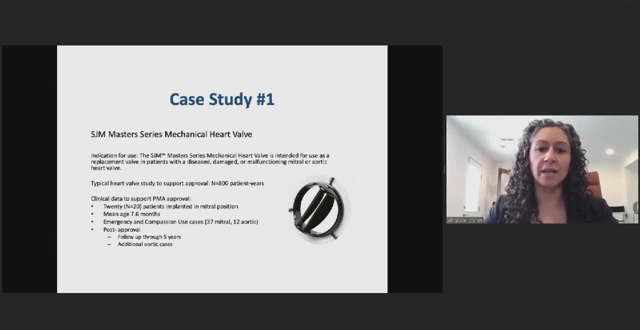 And what type of data do theydo we need to support approval in whatwhat is? one, a very small patient population, but two is a verya very difficult population to enroll in trials and toto follow and to gather data. 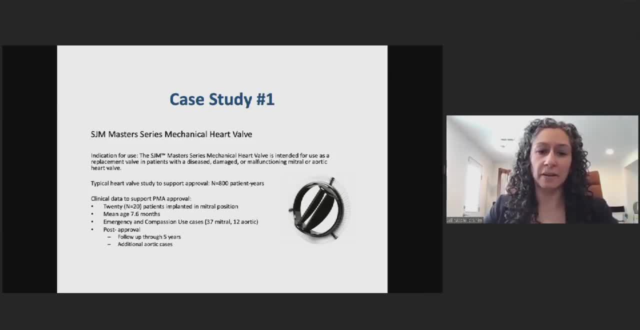 Because it'sfor folks that aren't aware in the audience. the typical heart valve study that we would require for a mechanical heart valve like this isrequires on the order of 800 patient years. It includes patients that arethat have implants both in the mitral valve position. 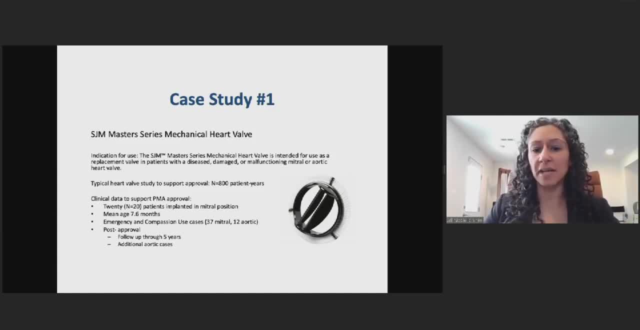 as well as in the aortic valve position, And for a pediatric population. to gather this volume of data isis quite onerous, if even possible based on the numbers thatthat we know about, So we had to develop a creative approach. 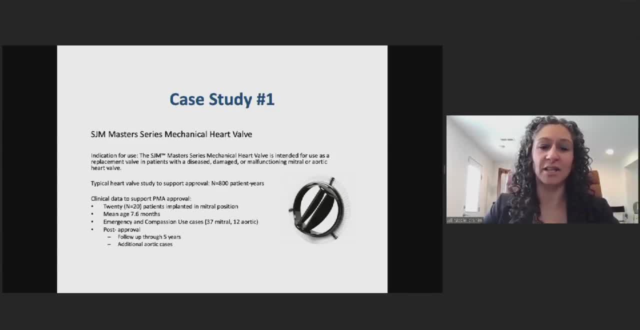 Otherwise there wasthis device probably wouldn't have made it to the market, And so what wewhat we determined, based on the population, is that we required a total of 20 implants in the mitral position, because that's the more common implantation site for this particular valve in this population. The mean age of the patients was sevenabout seven and a half years, Okay, About seven months, And so these were very delicate patients that were difficult to follow, difficult toto kind of carry out through your typical follow-up in ain a heart valve study. 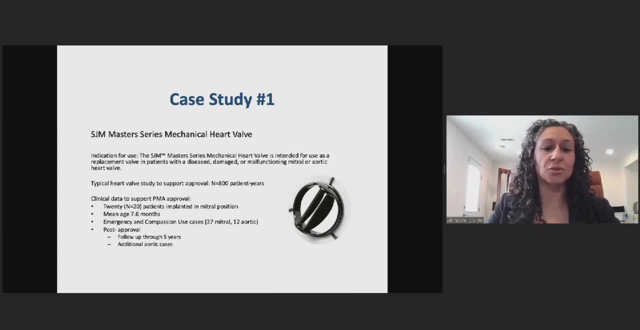 And so, in addition to that, we alsoin addition to the 20 patients that supported the approval, we also relied on some supplemental data from emergency and compassionate use cases, And you can see the numbers here. So quite a reduced set fromfrom thefrom the mitral valve. 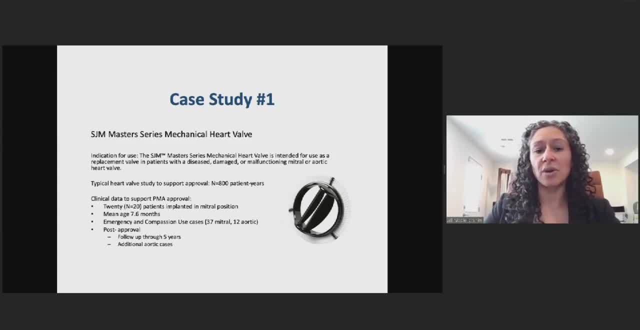 And really this is a little bit of a graphic explanation of what wewhat we expected fromfrom what we would expect for adults, But the idea was that we had learnings from the adult data, from the studies that had been done in prior decades, from the adult sizes that we felt were leverageable in terms 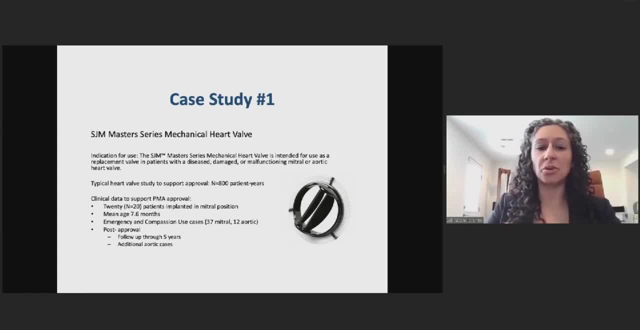 of performance for the valve, And what wewhat we were really interested in is understanding the safety profile and, But also in the post-approval space, we also required five-year follow-up of all the patients, as well as some additional aortic valve cases. 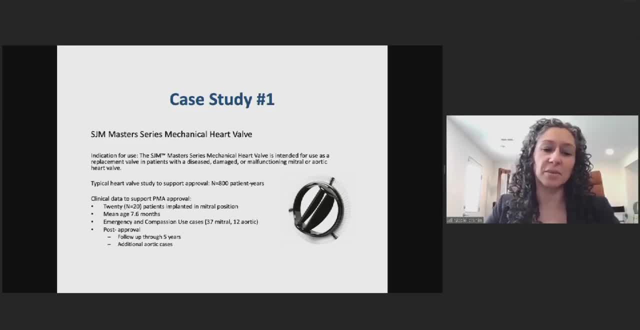 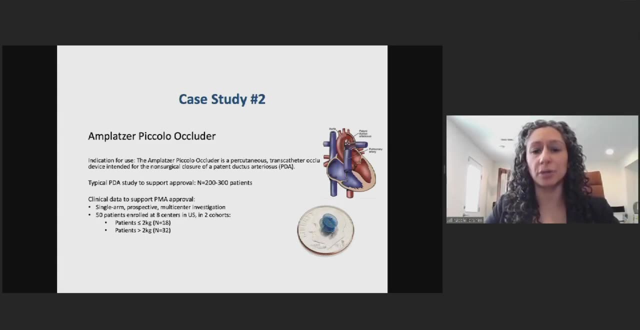 And so I think this is also an example of an area where we use the concept of pre-post-market balance to be able to obtain data in the aortic cases. So that's one case study. The second one that I put together is for a device called the M-plaster piccolo occluder. 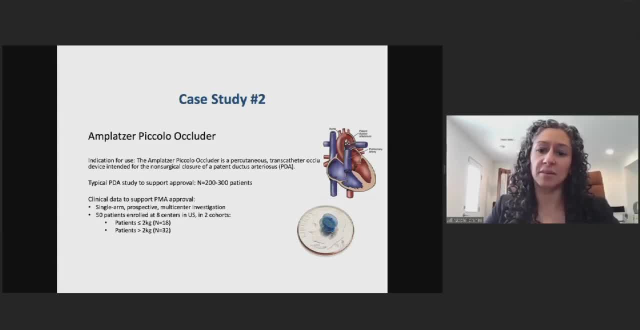 And so this is a very small device. You can see the aspect ratio here when it's put on top of a dime. So it's a very small device And it's intended for percutaneous closure of PDA in pediatric- well, in not just pediatric patients, but this is predominantly a phenomenon seen in pediatrics. 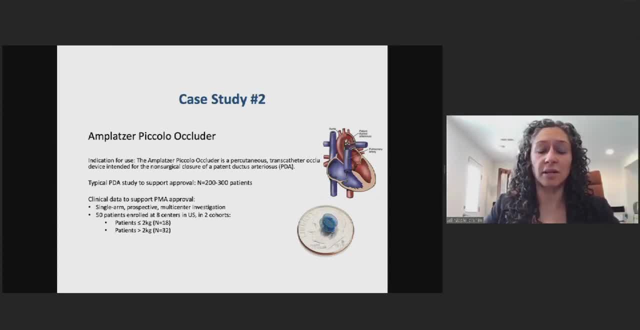 Typically, what we would require for a post-market study was on the order of 200 to 300 patients for the larger sizes of this device. But because of how small this device was, it really was intended to be used in premature babies or very young babies. 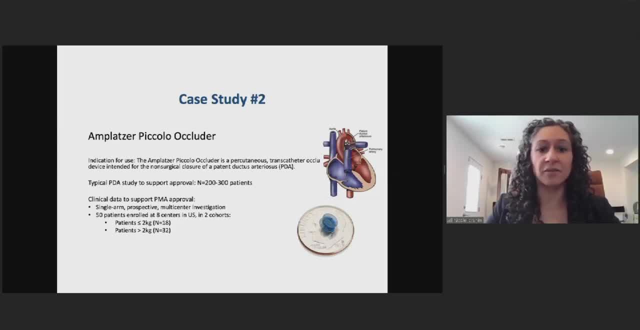 And so the data collection in that population was again going to be very challenging. So essentially, the way that we kind of came up with a creative plan was to collect data in a single-arm prospective study, And the study essentially enrolled about 50 patients at eight centers. 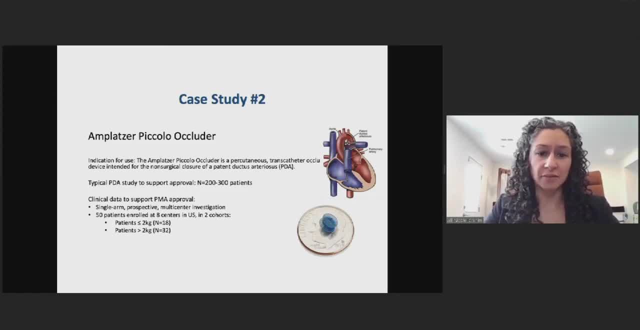 There were 18 patients that were in the very low birth weight infants And another 32 patients that were above two kilograms, And so, again, I think we drew from some of the experience of the larger sizes of this device in older pediatric patients to be able to draw from some of the effectiveness that we had seen. 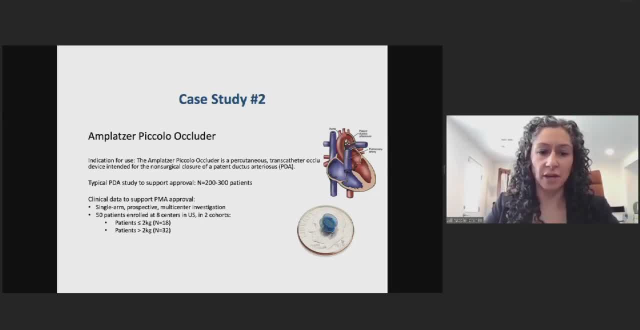 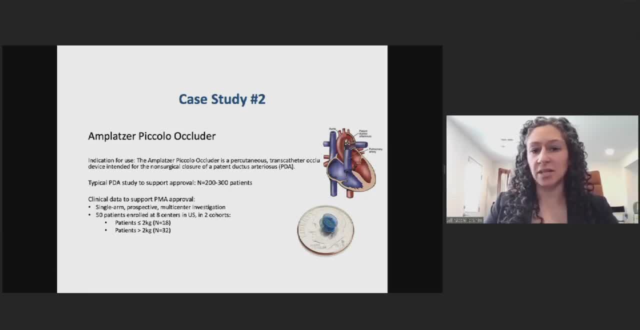 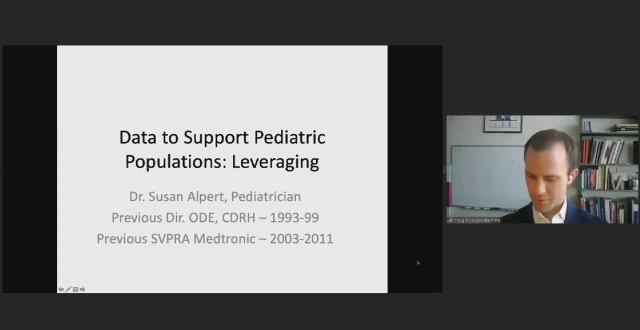 get a pediatric device to market. So I'm happy to answer any questions now or postpone until later, but that's all I have for now. MR, You know that's wonderful. Thank you, Dr Ibrahim. I appreciate both case studies. 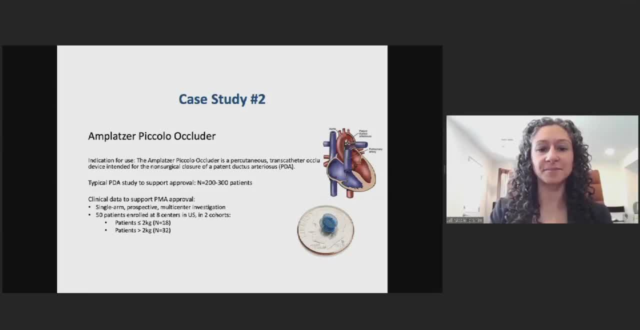 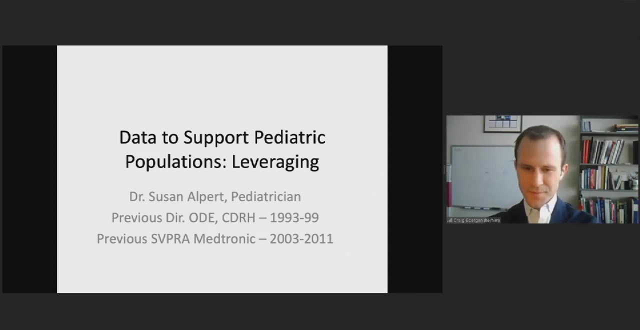 It's really interesting just to think about the numbers and the logistics for some of these smaller patient populations. There are questions coming in, but I'm going to hold off on the discussion portion until the end, once all the panelists go. So with that, Dr Elpert, are you wanting to go through your slides now, please? 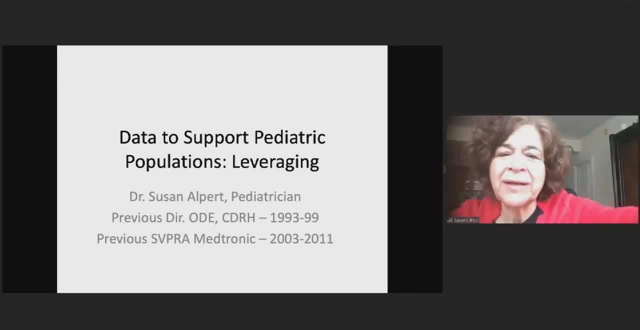 DR, I'd be happy to. Can you hear me, MR? Yes, thank you, DR. Great, I want to actually – it'll tag right off of what Nicole already spoke about, and it's talking about how to leverage data. 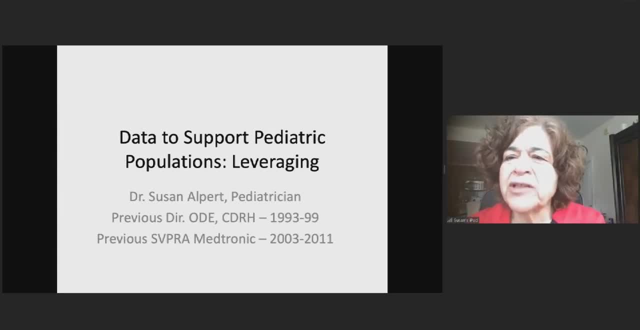 And I think it's important to read, It's important to remember that pediatric populations are not one population, They're multiple populations. So we have the neonates which she spoke about, But young children are not like middle-aged children, if you will: the eight to teenage. 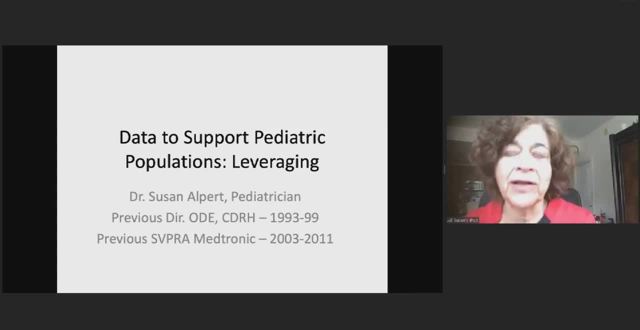 years. Teenagers are not like younger children, and yet they're not like adults, And so we actually are dealing with multiple populations. So leveraging isn't always just one direct thing and the leveraging that FDA allows, which is exceedingly helpful – wanted to enforce that – exceedingly helpful and 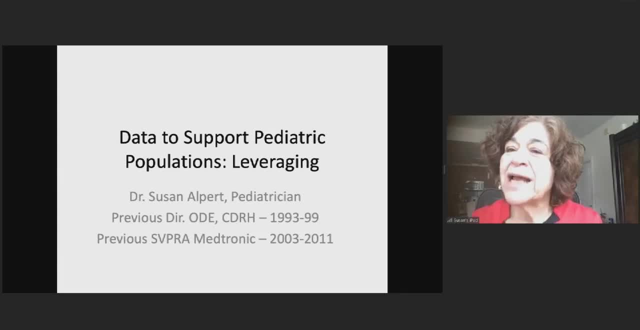 useful for companies is that you can leverage from adults, particularly into teenagers – remember, pediatrics goes to age 22 – but even teenagers. But for younger children, sometimes what we're leveraging is data from the older children and trying to leverage that. 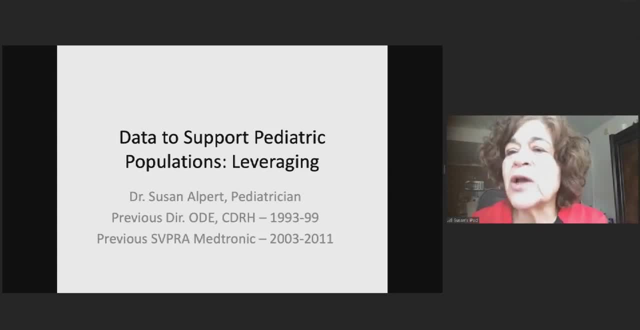 MR, There are diseases in many cases, where the presentation, the severity, the way in which the disease impacts the child's life is totally different depending on the age of that child. So leveraging isn't always easy, and I wanted – and the next slide, my example is one. 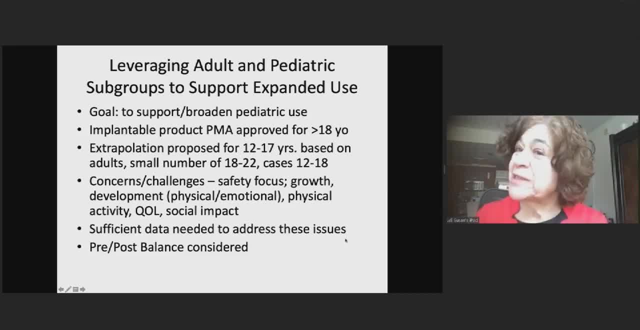 where it wasn't easy, This was – I can't tell you exactly the name of the product or specifically what it did, because it's not mine. It belongs to one of my clients, But I can in fact talk about the issue. 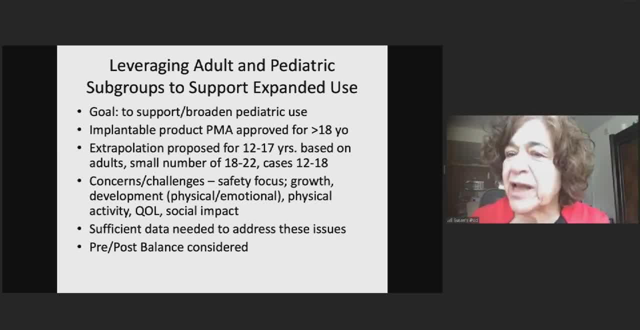 So the idea was to move from adults to broad use in pediatrics. It's an implantable device. Happens to be in neurology, but it's an implantable device, And the questions that came up were: how much leveraging? How much can you leverage? 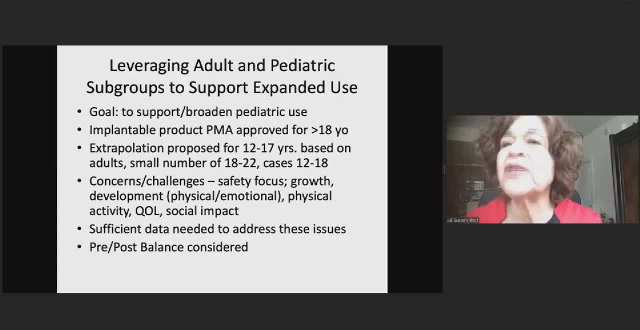 Clearly, as Nicole pointed out, safety sometimes needs to be directly evaluated by age group, because young children are much more active than adults. Size is different. They're growing. Shocking, I know, but they're growing, And so you – when you have an implantable device, how do you account for that? 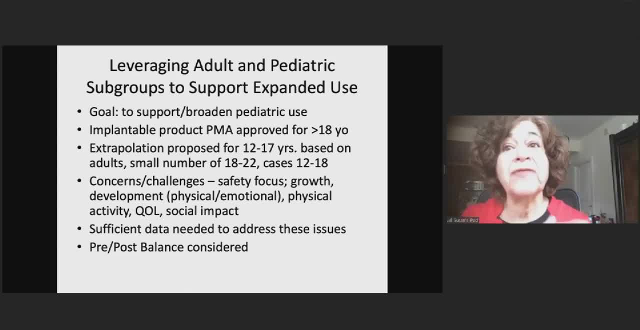 How do you make sure that it remains safe over the growth of a child? How do you design it to do that? So there are different questions Here. the issue was broad support across pediatrics, Implantable already approved for greater than 18.. 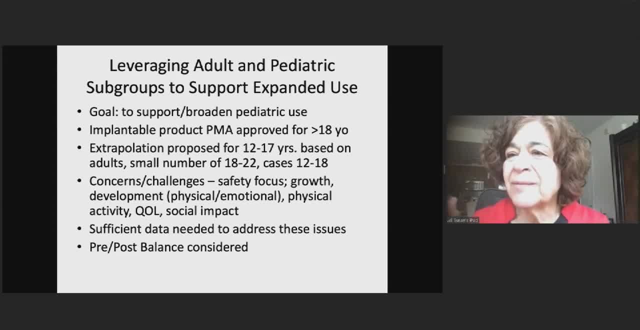 So the older children, Pediatric population, the adolescent population was covered, But the company really wanted to go down quite young but would start with 12 to 17,. again, in leveraging going down by group, because the disease presents differently and because growth is different and sizing is different and the amount – the way in which the device 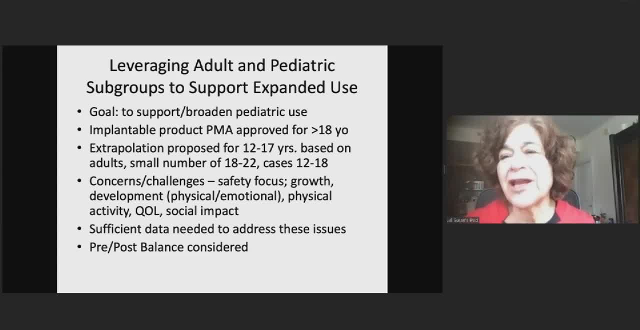 works has to be geared for the age group. Okay, There were challenges. We already spoke about safety, but growth and development, physical activity, quality of life and social impact- two things we don't always think about when we think about pediatrics. 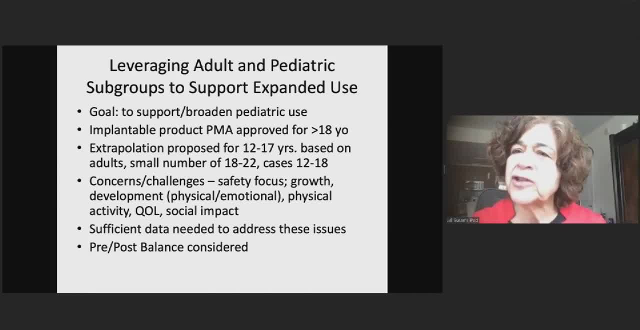 but we need to. So the quality of life of a child who's eight is a very different issue than the quality of life of a child who is 16.. We need to think about the impact that our devices have on their quality of life. on. 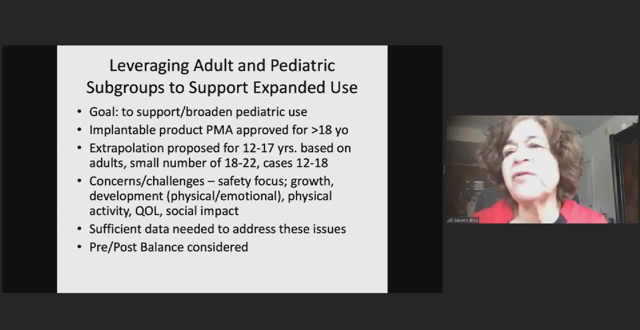 their social life? What are the limitations? What are the limitations of social development? Will they be able to participate with their peers? What are the limitations And will they need assistance? So in leveraging we need to think about age group, the disease, the product itself by 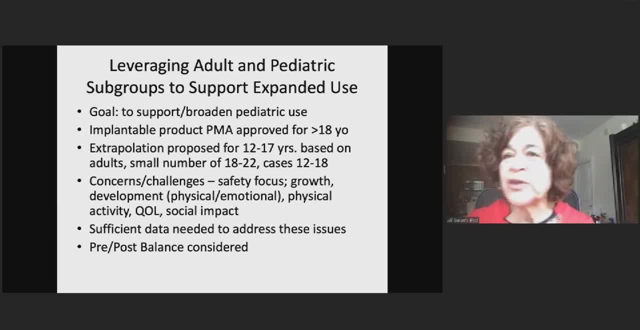 size or by activity. Sometimes you can – you can program devices for different rates of delivery. What's the rate of delivery of therapy? Well, what rate of delivery of therapy is appropriate for that specific age group? Again, very different: in young children, in midgroup children or in adolescents? 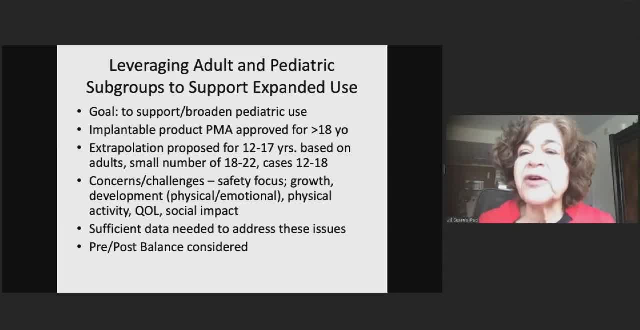 And how much data is enough. This company's experience was that they needed to do an actual study. A study needed to be done because, although there was evidence in 18 to 22, there were off-labeled tests cases for patients between 12 and 18, which they had, but it wasn't broad enough safety data. 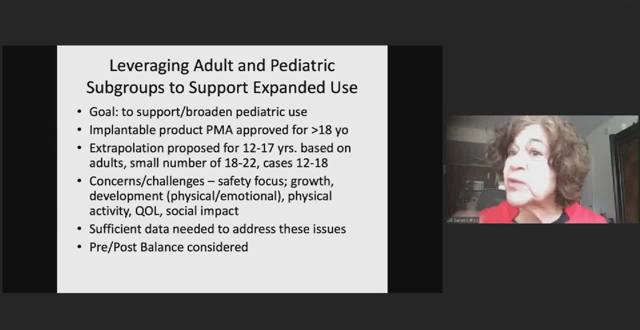 And therefore FDA did require safety information as well as some efficacy to be developed, even for those 12 to 17.. My point here is: when you're developing a novel device for pediatrics, you have to think about the different age groups. You have to think about how much 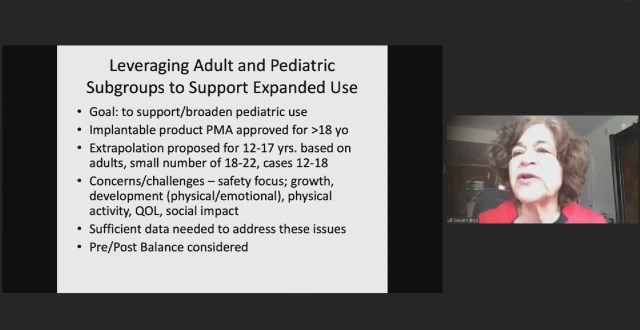 leveraging you can do, what kind of leveraging you can do and what types of data you will need to support either safety or safety and efficacy, in order to do leveraging in general and in order to have small enough studies that they're doable but impactful enough that they provide the 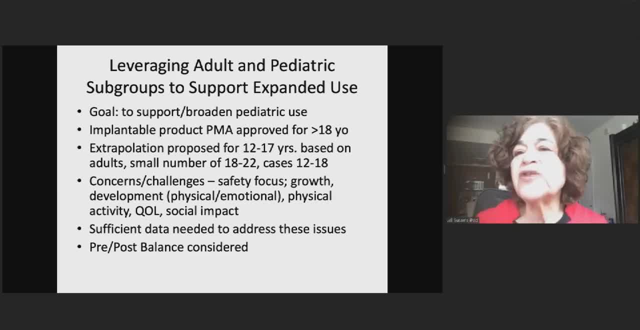 information to FDA. And then, of course, the plan to continue to develop data in the post-market market. And with that I'm going to stop and wait for questions on the practicalities of implementing some of these wonderful programs. but the practicality for the innovator, especially when 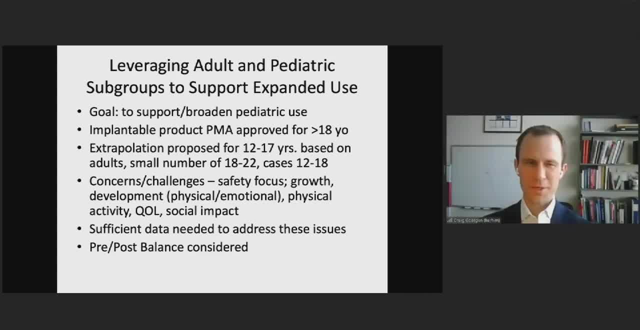 it's a small company. Thank you, Great Thank you, Dr Alpert. I'd be interested to hear more in the open portion about your experiences at the FDA and with companies and how the two should work together and best leverage the strength of each, and then thinking too about 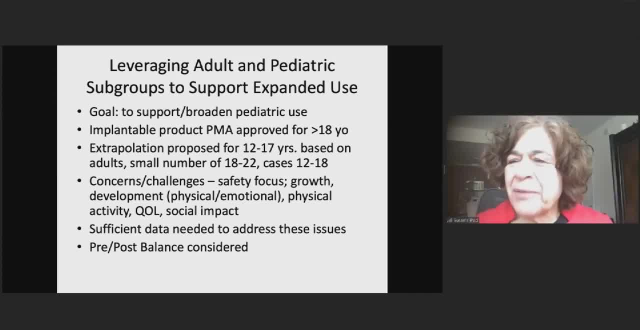 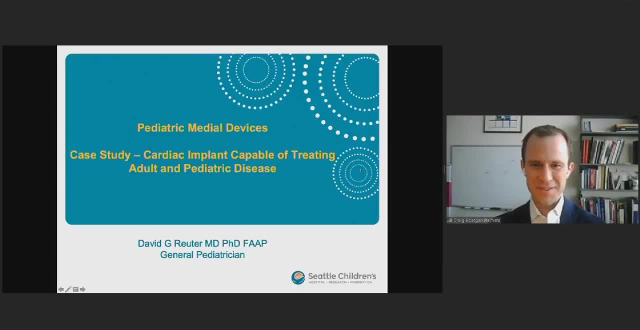 small companies, as you're in your consulting role now too Happy to do that. Yeah, I've worn all the hats. Wonderful, All right. Now we're on to Dr Reuter- Awesome, Well, thank you for the invitation. 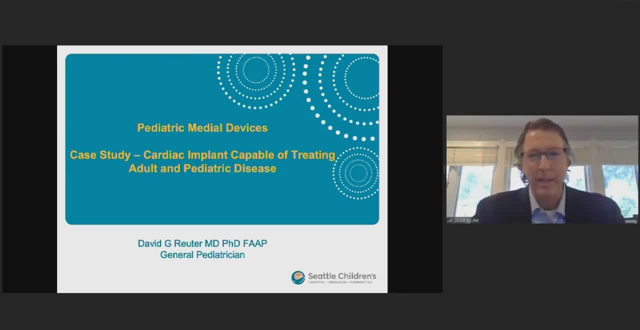 It's a privilege to join this distinguished panel and to add to the case studies. I also very much enjoyed the discussion and presentations this morning. If there was a bit of a theoretical premise to the entire product, I'd be happy to answer that, Thank you. Thank you, Dr Alpert. 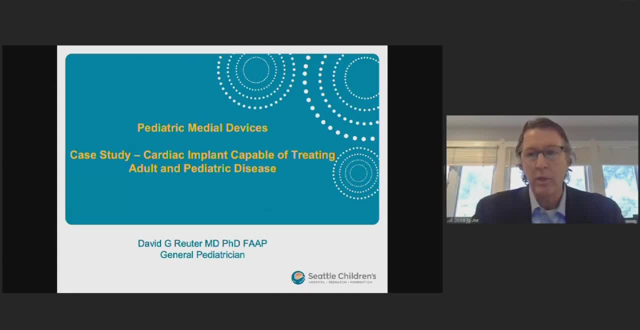 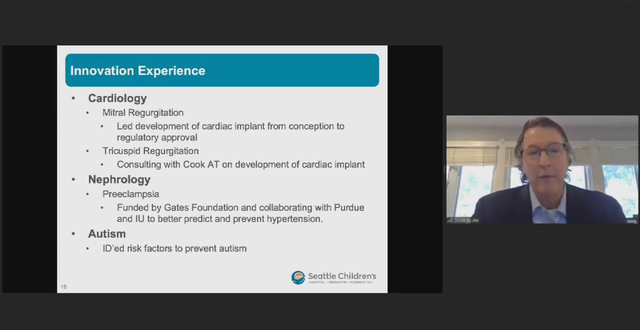 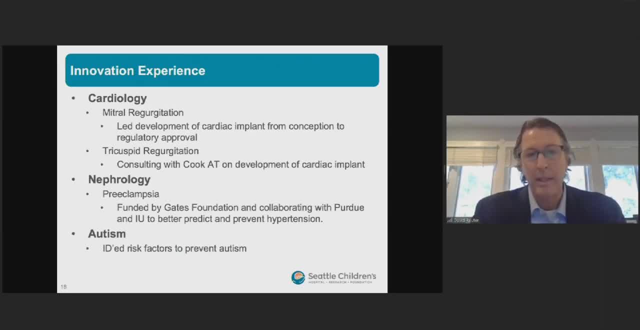 of mitral regurgitation. And again, my experience is that back in 2000, I started a company and I led the development of a cardiac implant from conception through regulatory approval. I'm going to share some details of that effort, but what I want for the audience to be aware 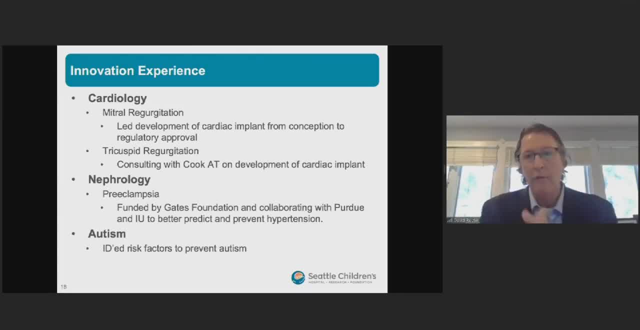 of is, there are certain fundamental principles that we use at each phase of development And so, independent of the specific technology, my hope is that this example, this case that is going to highlight the path that any of us have either gone through or we have the 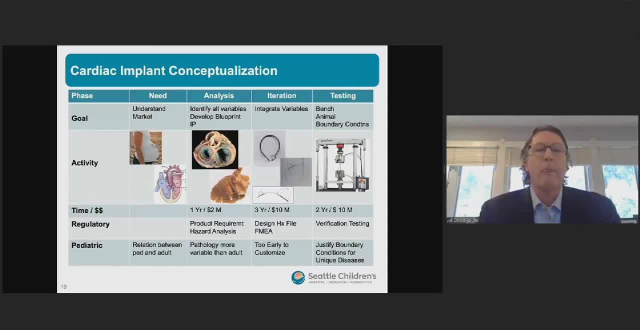 opportunity to Next slide, please. So this slide lists the first four phases of development as I see them. We've heard people say before that step number one, phase number one is to identify the unmet needs. For me, if I make it personal, back in 1995, there was 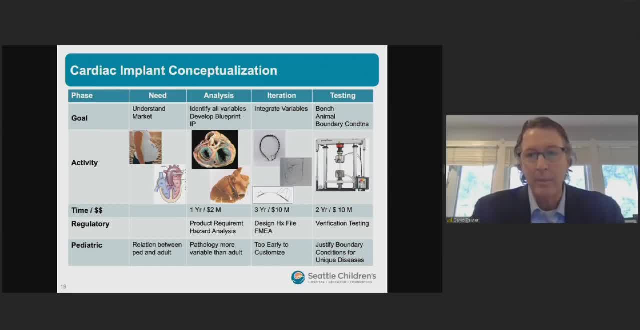 an unmet need for a cardiac implant, And so I'm going to share that with you. I had an 18-year-old single mom that walked into the emergency room at Pittsburgh Children's Hospital complaining of shortness of breath And she says: maybe I'm tired because I haven't slept. 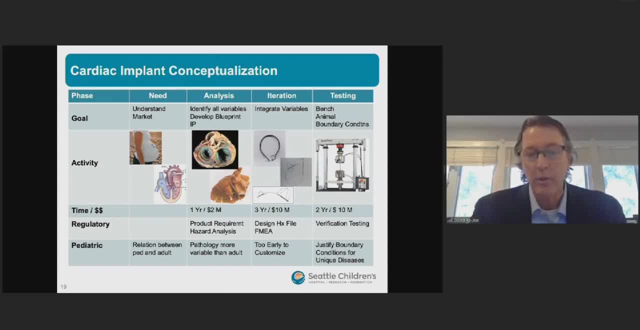 for three months, but I got a chest x-ray and her heart was huge. She had heart failure caused by her pregnancy. We took care of her for about two and a half years, And in the final year of my training we learned that Danielle had died, leaving behind her three-year-old son, And so this was. 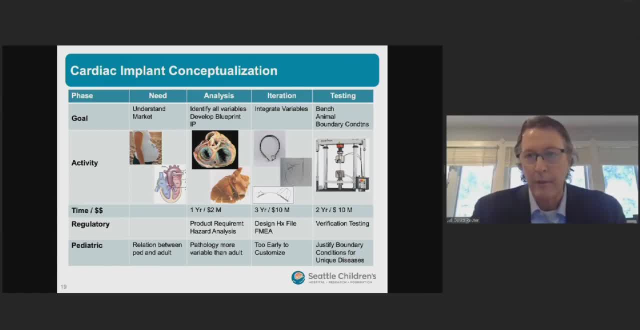 the first experience for me that says that this effort to innovate and to make medicine better for those patients that depend on us is a critically important thing. Danielle's disease was interesting because it was heart failure, but it has a close enough variant in the adult world that I knew we could develop a device for adults take advantage. 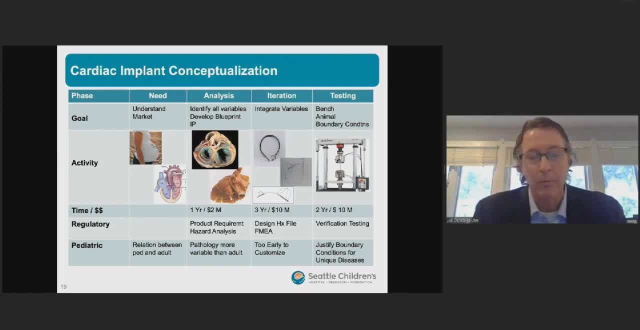 of the $70 million in venture capital money that we had to raise and that would eventually be able to bring it into the pediatric population. At least, as Dr Alpert said, we were able to bring it into the pediatric population. But, as a pediatrician, there are a variety of 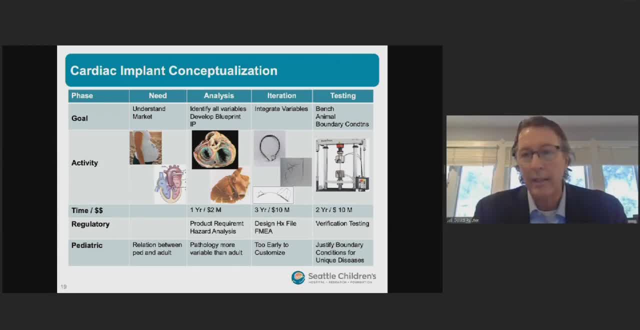 different, very specific, rare, unique cardiac conditions And the image on the bottom right there's a patient with truncus arteriosus. There's four chambers to the heart, There's an aorta, but there is no pulmonary artery, And so it's an example of one of the cyanotic diseases. 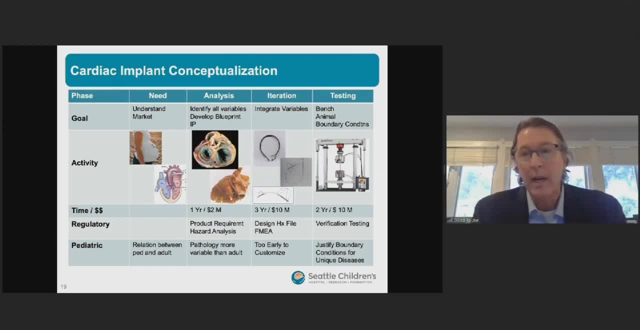 So step number one, I think from a pediatric advocacy standpoint, is to understand the relationship between pediatric and adult pathology. Phase two of innovation is the analysis phase And having now done this three or four times, my personal opinion is that this is the most important part of innovating a novel technology. 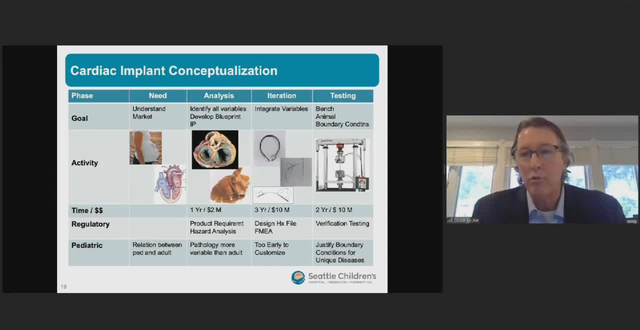 And Purdue taught me this- You have to study the problem in extraordinary detail, right, You have to identify every single variable that's contributing to the pathology, because what you need to do is to align those different variables in such a way that you can come up with a blueprint. 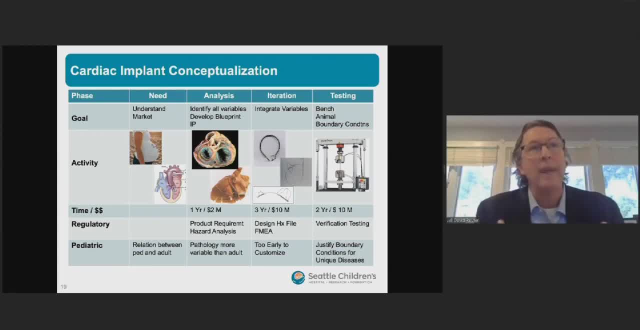 a design of what that device is going to look like. There's a lot of value in that creative process, Specifically for the innovator. we can see in our minds- before I've ever made anything, what that device is going to look like. 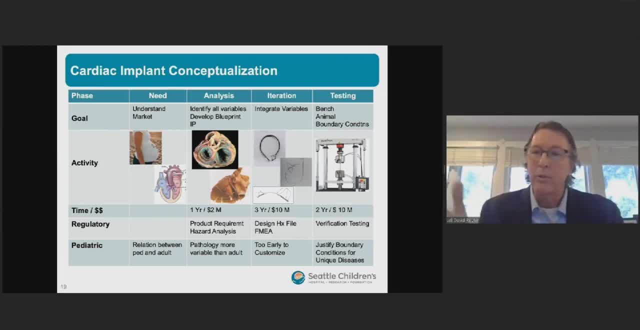 And you capture that in the intellectual property And down the road when somebody needs a return on the investment, that IP happens at this early critical phase From a regulatory standpoint you can see that the device is going to look like a blueprint. 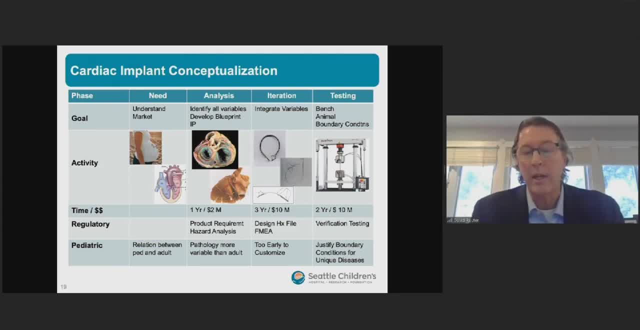 And from a regulatory standpoint that device blueprint is called a product requirement document And all the different variables that can cause different issues. clinically we would call it a hazard analysis. So this is starting to assemble the material that's going to be submitted to the agency eventually. 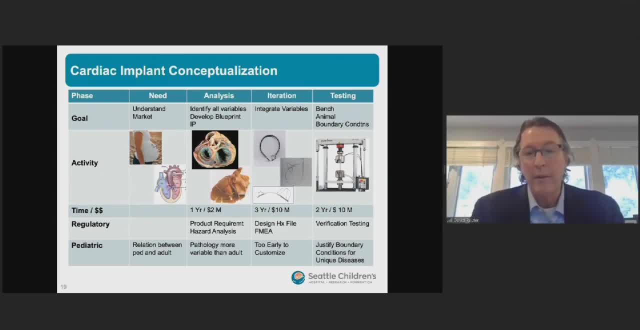 Again, if we take the pediatric angle to this, we're all aware, as I've already said, that the pathology in kids is a lot more variable than adults. I looked at 100 different ways that we could do this. I looked at 100 different parts, half at the University of Washington, half in Minneapolis. Jesse Edwards collection of hearts. 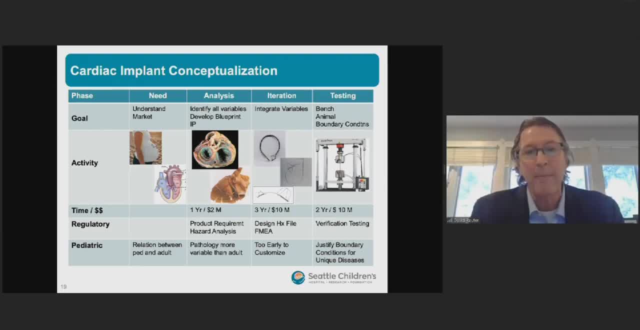 just to look at adult disease, which is less variable than kids, And I think that's one of the challenges. Phase three is the iteration phase. Once you know what the device needs to do, then you need to come up with something that does it. 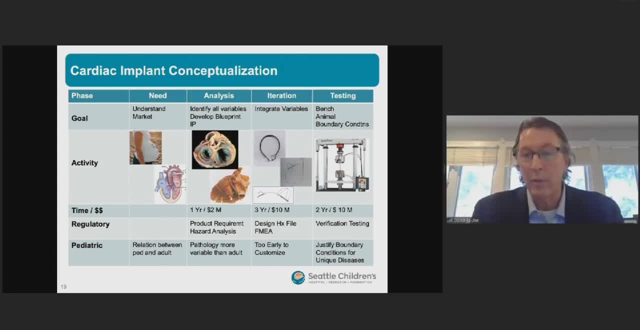 You don't have to be creative or brilliant to start, You just need to start with anything. Top left is the first device that I came up with And when we put it into an animal it was an 80% failure. It rubbed against the tissue, It eroded the tissue. There's blood in the pericardium. The animal is going to die anyway two days later, and it did. 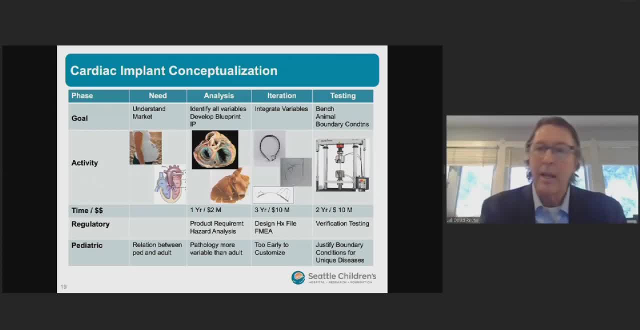 You study that failure mode and you come up with the next iteration. That second device was about a 50% failure. But again, this idea of analytical thinking and let me understand the failures and iterate the design so that you can prevent all of those different failure modes. 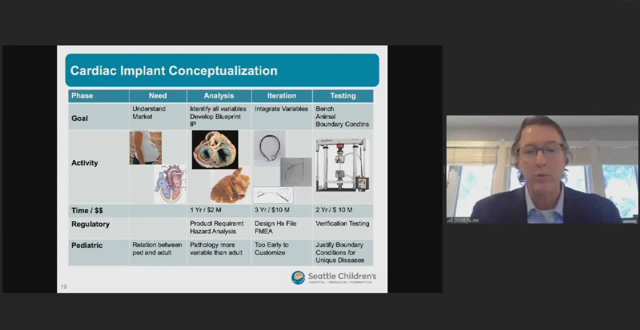 Again from a regulatory standpoint. Not only are you going to submit some sort of design history file that says this is what we did and why, but in my mind More importantly is, you can present to the FDA that failure mode and effects analysis. 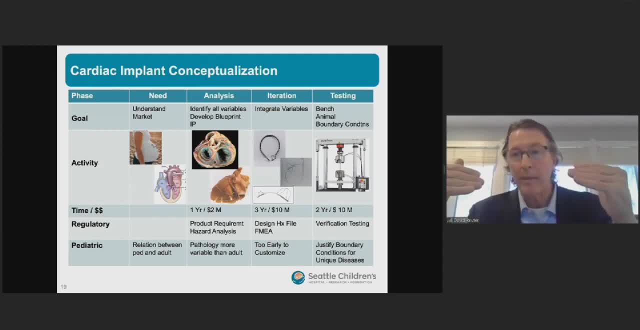 I've seen all these problems, Some of them I created on my own, just to see what's going to happen in the clinical setting. And here's the design of the device we've Generated in an effort to prevent those failure modes. So I put. 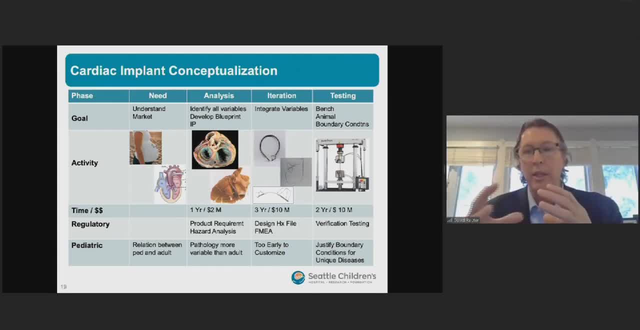 A lot of effort into the design of the device And I personally think that really clear communication with the, with the agency- not only what have we done, but why have we done it- And let's make sure that we Take our expertise and share it in a way that that some sort of a unique device can be thoughtfully evaluated is important. 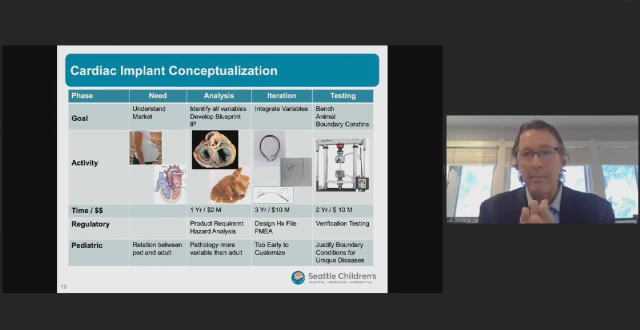 The fourth phase is the testing phase. It's a it's a Critically important decision step to say when do I freeze the design of a device, Testing and eventually, clinical testing. Testing is going to involve both bench testing, animal testing And again, this is where that analysis phase was so important. You need to set the boundary conditions. 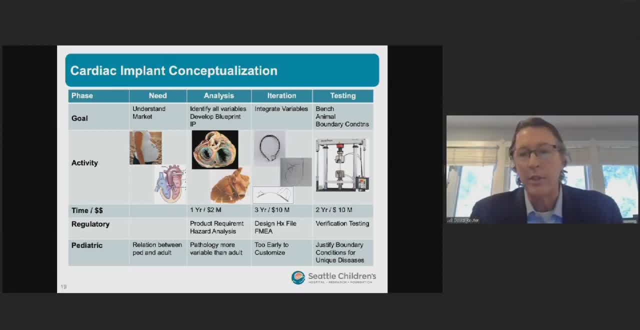 And what are the forces that the device is going to experience? What's the range of motion? You see a picture there of a fatigue tester That might be two years, $10 million. This is some of the verification testing that you do on a device to say that design, that we told you about it. Step one: 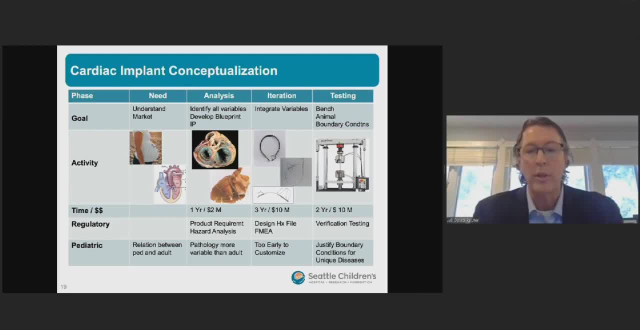 Now we've tested the device And we're proving that it does What we told you it's going to do Again: the challenges for pediatrics. It is extraordinarily difficult. you know I did 100 different animal studies in three different animal models. 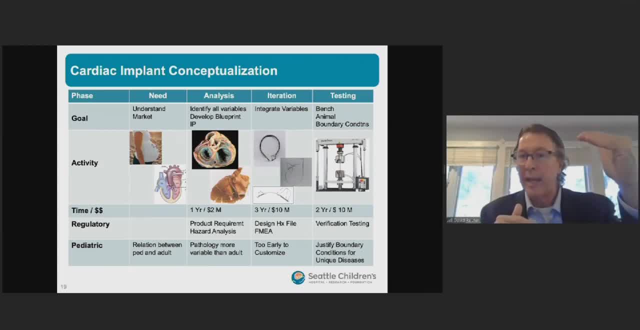 Trying to take a specific anatomy or physiology of an animal that I was trying to extrapolate to a person And that's just trying to mimic an adult disease which is more homogeneous. So how do we justify different boundary conditions For some sort of pediatric pathology like a truncus arteriosus? Next slide, please. 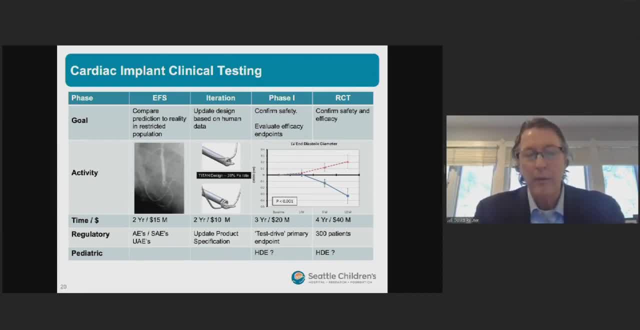 As Andy farb said, there's only so much that you can do a theoretically and on the bench top. at some point you have to get into the clinic. I so appreciate. the FDA is dynamic in evolving Program. When we started in 2000 that EFS program did not exist. 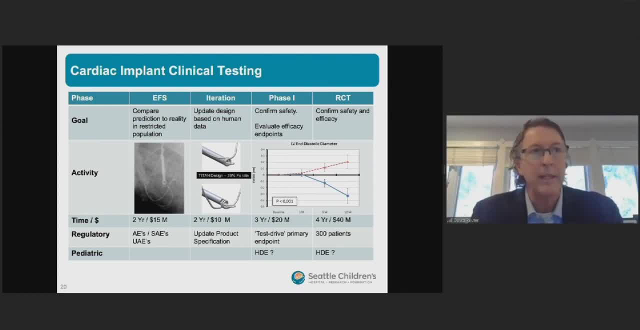 There was a lot of Discussion between industry and the FDA and huge credit to them for generating this EFS. that really allows us to compare what we predicted, what we, what we saw in an animal setting. Did we make the device robust enough that it can withstand human physiology? and you see, in that picture of the device that we generated, 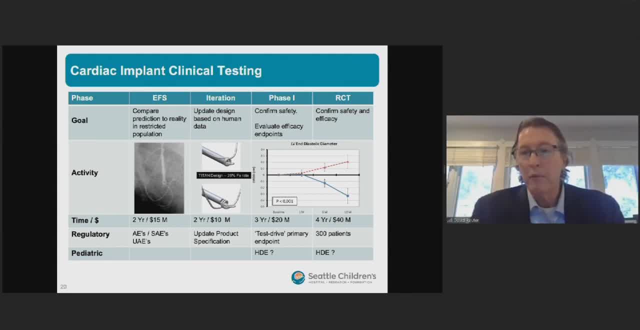 That there's a fracture of the device, And so this is proof that you Learn some important lessons, sometimes in the first five or 10 patients of a clinical study. So we do not want to subject 30 different patients in a phase one study to a risk. if we can put a device in, learn some critical. 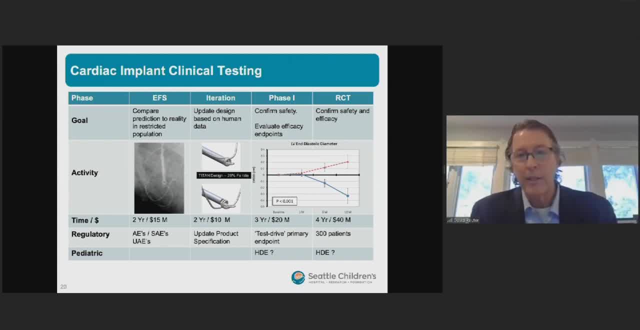 Insights as it relates to the safety, the adverse events, serious adverse events- and iterate again that EFS study is a is a really thoughtful and valuable Manner to do that. You'll notice the phase six, I believe. we're iterating again and you'll notice how this time, that iteration is incredibly subtle. We simply twisted the wire forms from the top of the device to the to the bottom, but there was a stress point, is some very there was some fatigue analysis that we did. 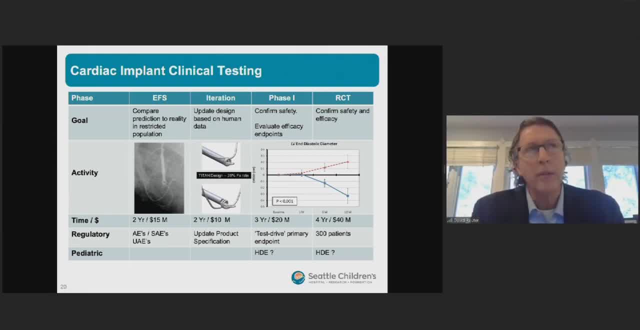 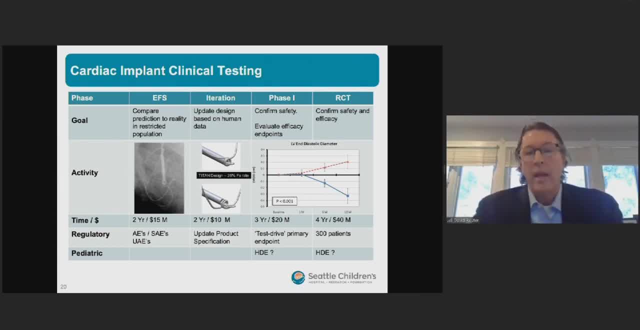 So we're going to go ahead and get started. So we're going to go ahead and get started. And then, once you have a device that's going to withstand the environment of of clinical physiology, you then embark on the more robust clinical studies, phase one in the randomized study. 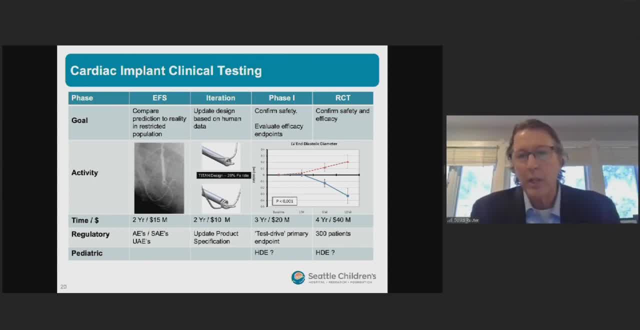 In my mind the purpose of a phase one study. you've already shown this going to be safe in the EFS, So for me the biggest thing we can do in a phase one study is Only confirmed safety. but you want to test drive different primary endpoints for a pivotal study, um part. 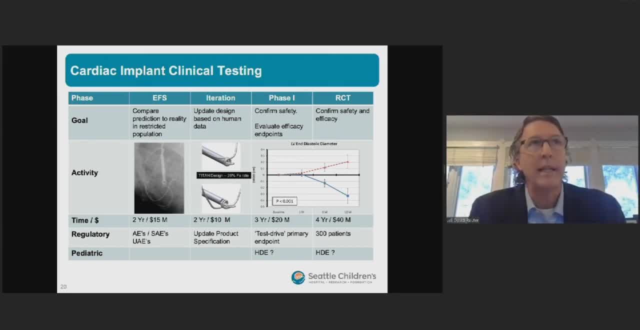 of the dialogue earlier was: how do we get venture capital to support any given idea? and i can just tell you that: um, if you're going to innovate, failure is not an option. um, if an, if a, if a funder doesn't see that, you're going from point a to point b, to point c, d, e in a very systematic. 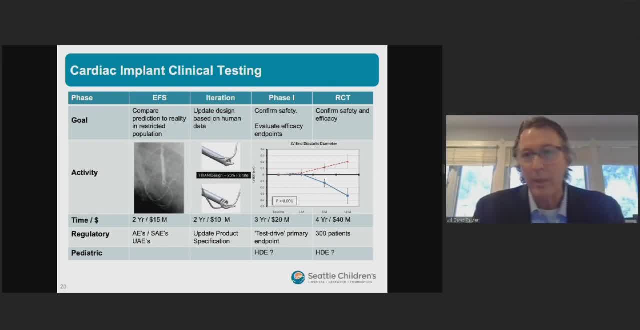 thoughtful, efficient manner. you're not going to get that 40 million to do the pivotal study. um. one last personal um anecdote: having um proctored many of these um phase one studies all around the world. um we had a very productive site in riyadh, saudi arabia, and like once a month, 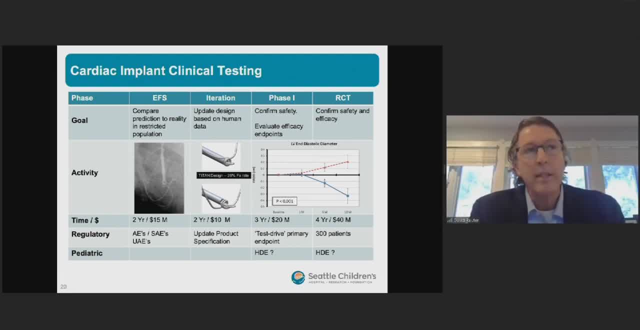 i would travel there to proctor one or two patients and we've done maybe eight or ten. we're getting really good results. we had a great um interventionist that we were working with and about my eighth trip there. there was some gentleman standing in the back of the. 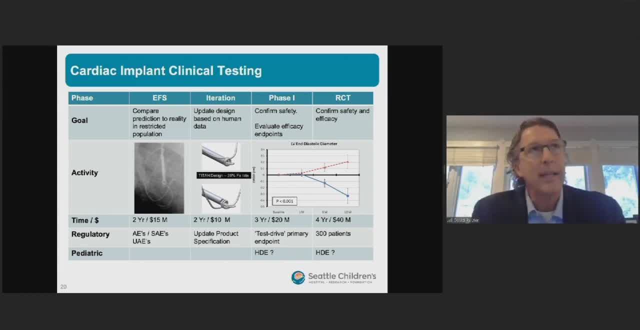 lab. we finished deploying the device and he comes up to me and say: hey, david, i'm um, i'm head of pediatric cardiology. we've been watching your implant, we've been talking about it in the institution. i've got a 10 year old patient with truncus arteriosis and i think your device would. 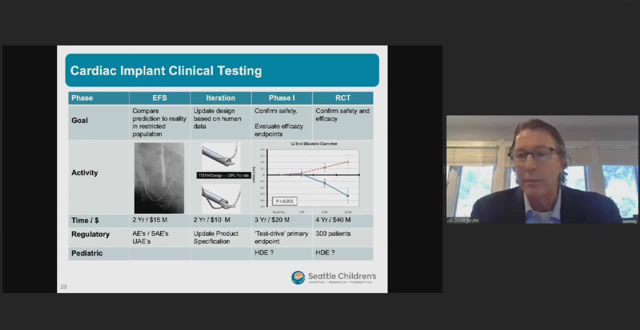 work well for them. would you be open-minded to making it available? in a capacity similar to this hte and having taken 10 years of my life devoted just to innovating something, as a person who's going to be able to do that, and i think that's a very important part of the process- 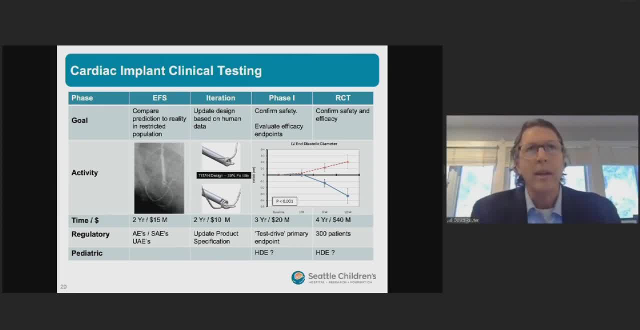 and i think that's a very important part of the process, and i think that's a very important part of the process. it was an interesting decision point for me to say no, i'm not interested in that right. as a physician, you take care of one patient and you do. 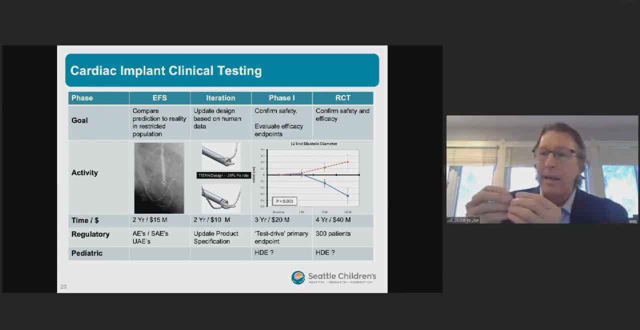 anything you can to make that patient better. but as an innovator, i was developing a therapy- a therapy and i need. i knew that our therapy was still in a vulnerable position because we just had a fracture. we're just starting to get some new clinical data. we hadn't 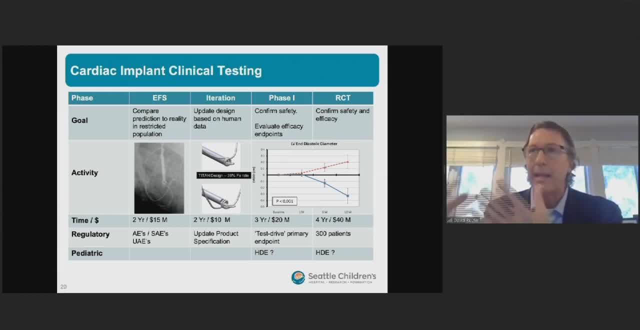 created momentum enough and respect and data etc. for the therapy to go the distance right, and so it's a very interesting dichotomy of what are you advocating for a patient or a therapy, and it really begs the question: what is the right time to take that risk? 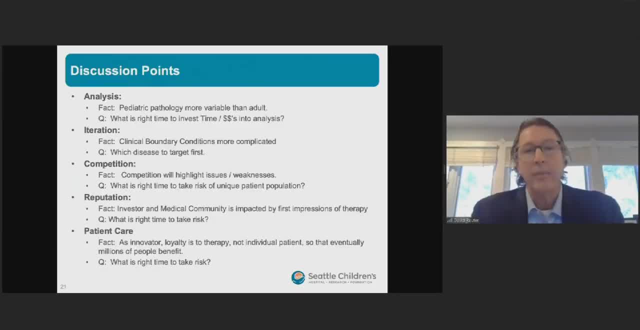 so my final slide in less than a minute is: um, you know discussion points as needed when you're in that analysis phase. it's just the fact that pediatric pathology is a lot more variable than adults. what's the right time to invest the dollars and time to do? 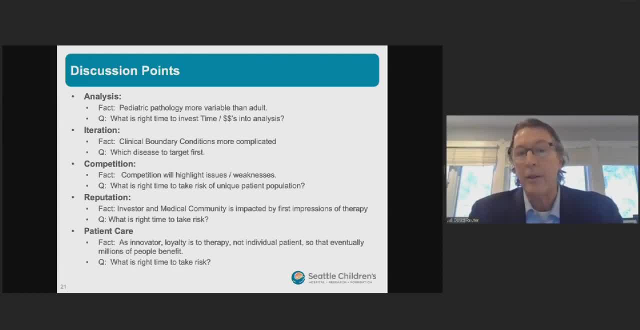 that the iteration phase, as i said, the clinical boundary conditions are more complicated. which disease do we target first? the competition: um man, there was 5, 10, 15 of us all trying to develop a similar device and we're all trying to help patients. but we're all competitive and there's 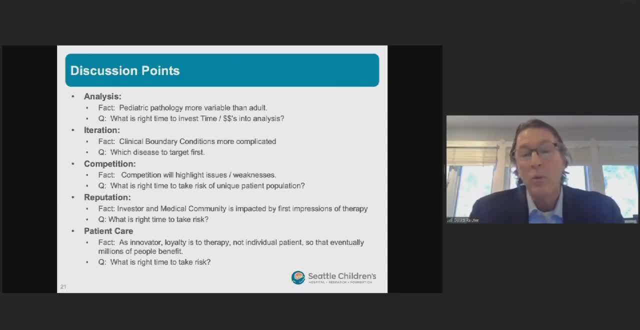 only a certain number of corporates that are going to help us get to the next level. we highlighted each other's issues and weaknesses and so there is a decision point of what is the right time to take a risk with a unique patient population. you don't want to make the company and therapy vulnerable. 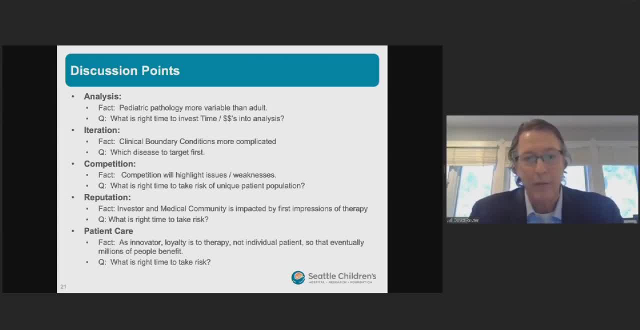 similar with reputation. one develops a reputation in the investor, medical community, the regulatory community, as i suppose as well, and that reputation is impacted by the first impressions of the therapy. so what is the right time to take that risk in a unique population like this? and then patient care, as they already said, as an innovator. it's just fascinating that the 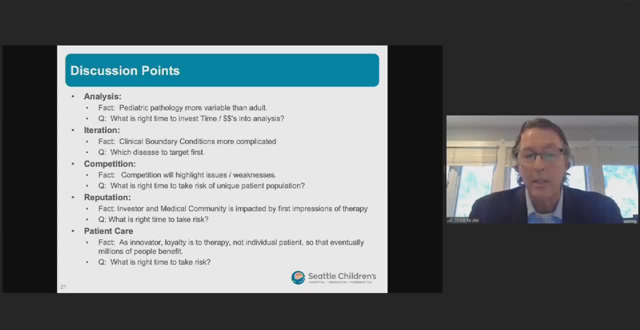 loyalty is to the therapy, not to the individual patient, so that, eventually, thousands or millions of people might benefit. um, and so these are. these are judgment calls, but they're just incredibly important to get right. uh, thank you for the time, and i too look forward to discussion um. 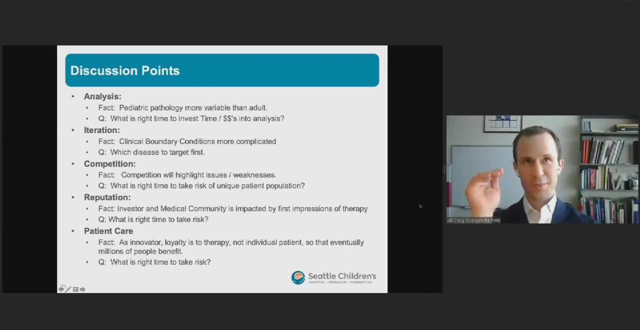 questions at the end. thank you, dr writer. so you went from 90 mortality to 50. i'm assuming third generation got better than that. you were doing a higher, higher, uh, lower mortality rates at that point. well, no, none of it was mortality, all of it was just um. 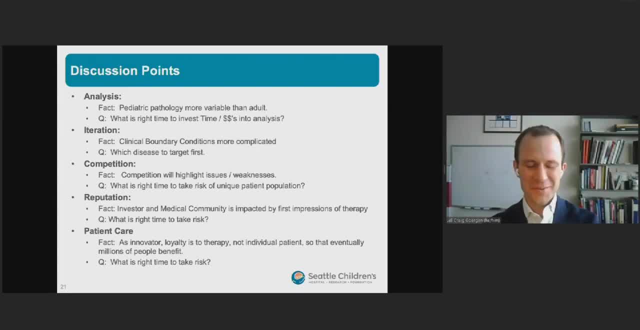 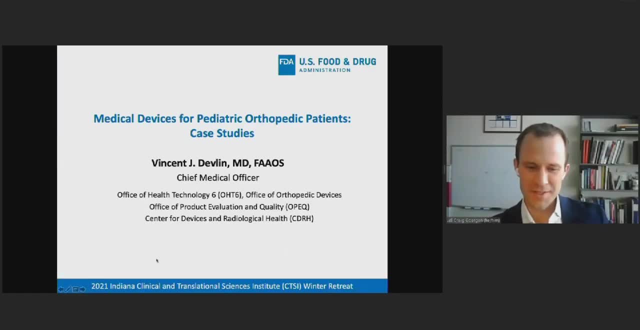 sheep studies and, yeah, studies in australia with the, with the animals. yeah well, thank you, that was wonderful, it was good. yeah, yeah, yeah, all right, and now we're going to move on to dr devlin and i'm actually going to stop sharing my screen. um, and dr devlin, i'm going. 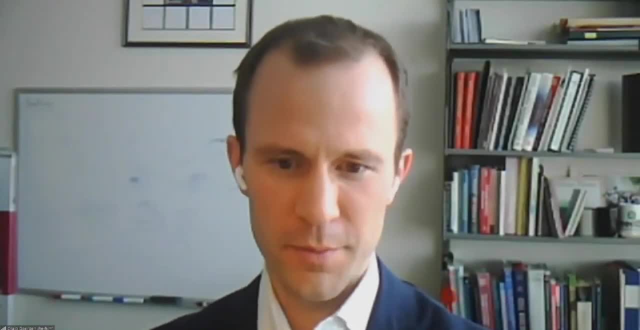 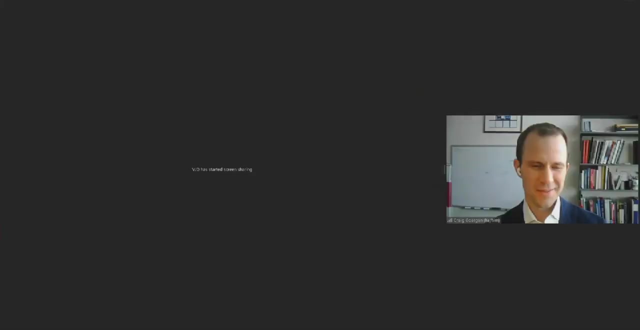 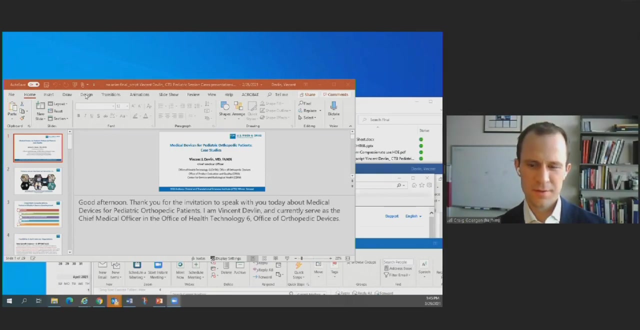 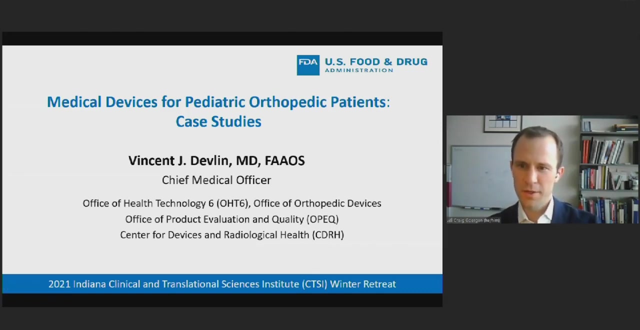 to let you go ahead and share from your end. hopefully you should have that function from your screen. perfect, so we see you. perfect if you go down and hit share screen, wonderful, so we. i am not hearing you, dr devlin. um, i wonder if we can figure out your audio. 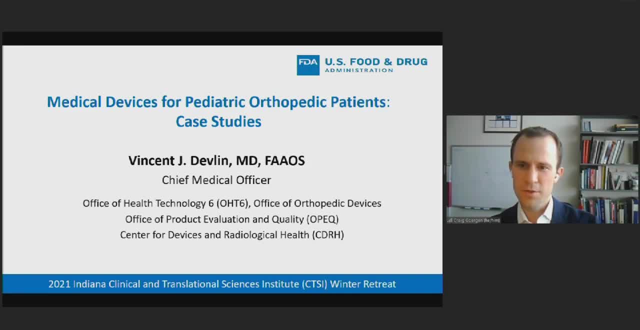 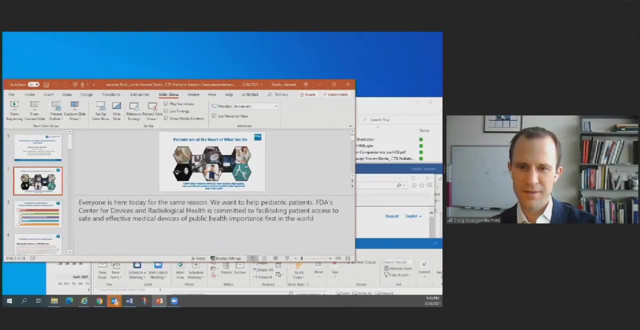 is there a microphone setting? you could try one second as we uh figure out technical difficulties, maybe we can bring it to share, okay, so while we're doing that, actually let's jump into then one question, um, just so we're not wasting everybody's time. um so, dr denny, you were interested. 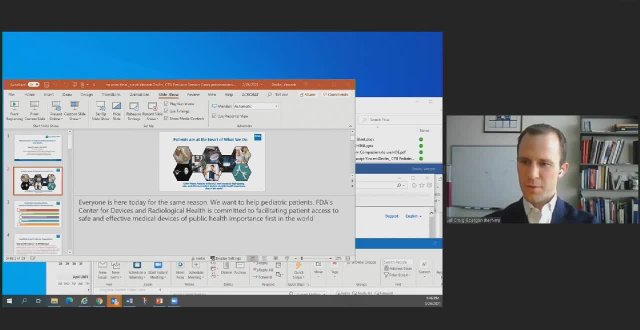 in asking a little bit about um, uh, irb for oversight for these hte devices and exemptions. um, are you available? yeah, go ahead and ask um, so, so the i'm i'm a long time, so i'll just kind of let them know in my next lecture. you know i'm very used to it, but i'm sure you're gonna start to say: 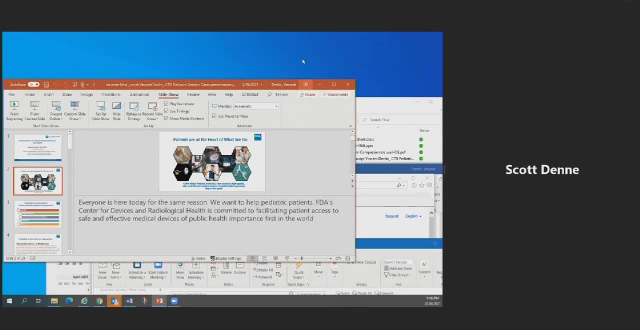 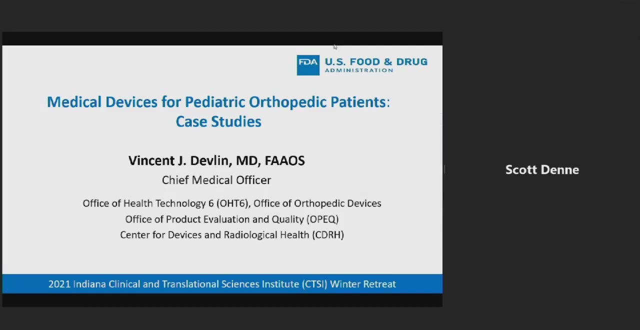 a longtime IRB member and chair and HDE. things come up occasionally and I can anticipate what the IRB member says, which is why are we involved in this and what are we supposed to do with it. And just my experience over multiple reviews is that I don't think this adds anything. 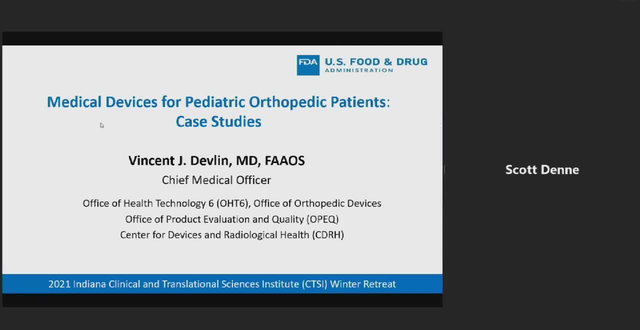 to the process. I'm clearly in favor of robust oversight and review, especially for children, but I don't think this adds anything And I was wondering: has the FDA actually looked at whether they're accomplishing anything by this requirement and whether they've considered? 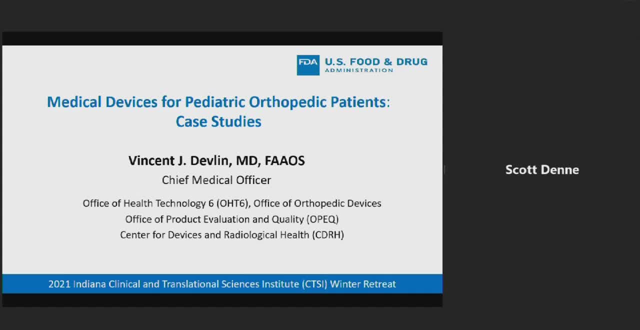 eliminating it. Dr Ibrahim, do you want to start with that? Sure, So I think it's a great question and I've actually heard very similar comments over the years, not only from IRB members, but even more so from the users, from the physicians themselves. 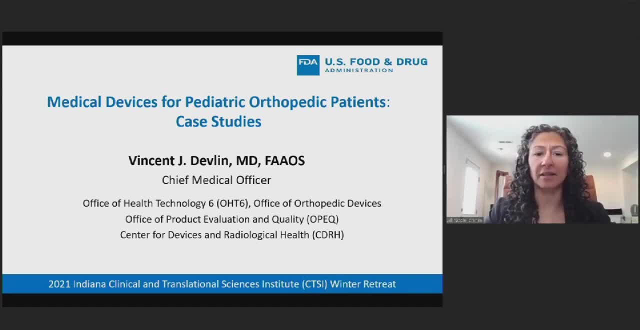 kind of trying to get a better understanding of what the utility is of the IRB approval process for HDE, And I don't know that. I think the question was asked: have we ever re-evaluated or have we ever re-evaluated? And I don't know that. I don't know that. I don't know that. 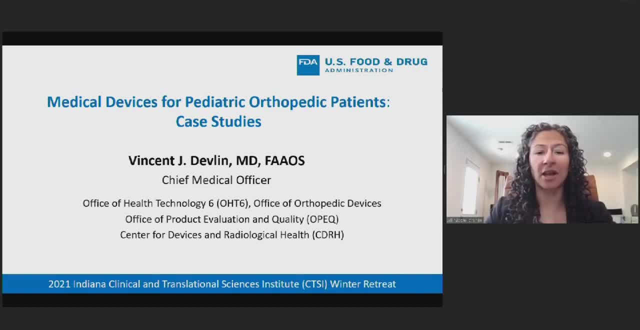 but it was a hard question And you know I'm not going to do that by myself. But I've just thought about whether it accomplishes what we had intended it to accomplish And I don't know that there's necessarily been re-evaluation- I'm not so. the HDE pathway is as you can imagine. 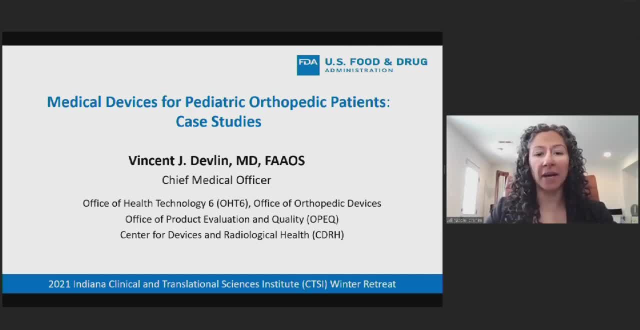 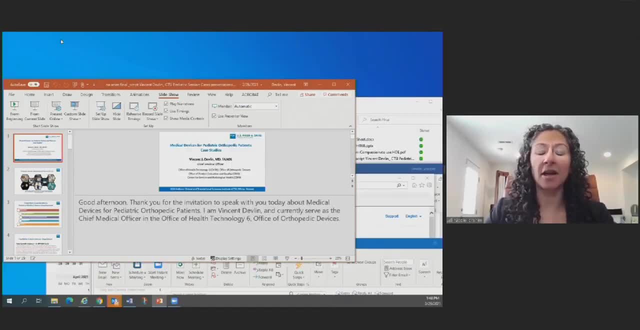 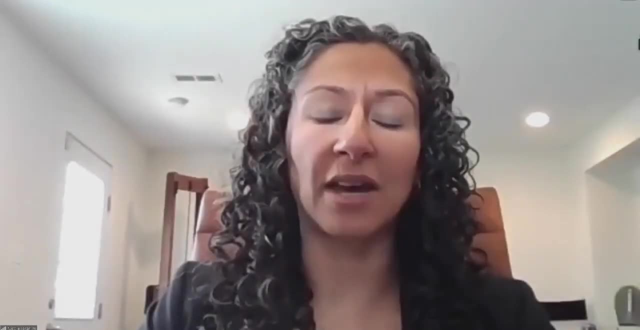 not utilized that often. But I don't know that we have necessarily kind of gone back and looked at the utility thus far. I will say, and I think you're probably aware, that the idea behind the it was to make sure that for a device for which we don't have established effectiveness, that we 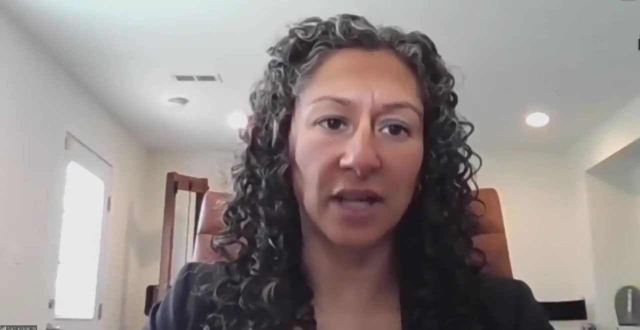 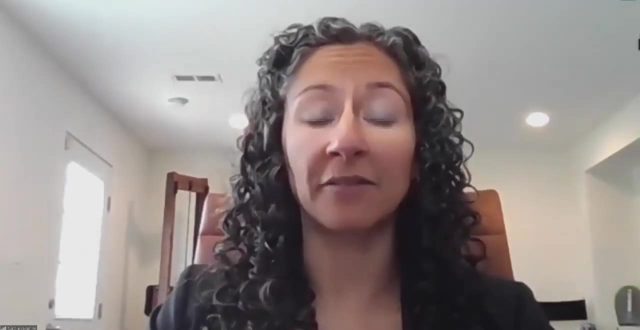 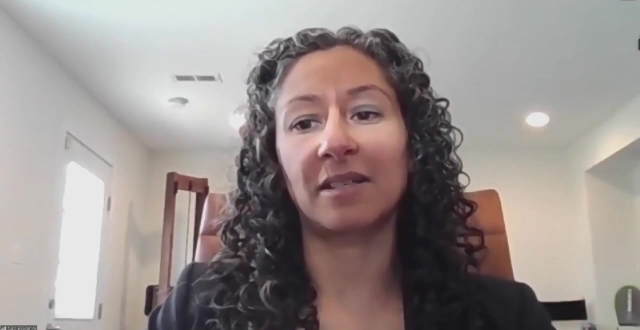 wanted there to be some additional oversight on use of the device to be able to mitigate some of the the- you know the issues associated with demonstrating problem benefit. so that was really the solution that we developed to get at that, but i do think that it is something that 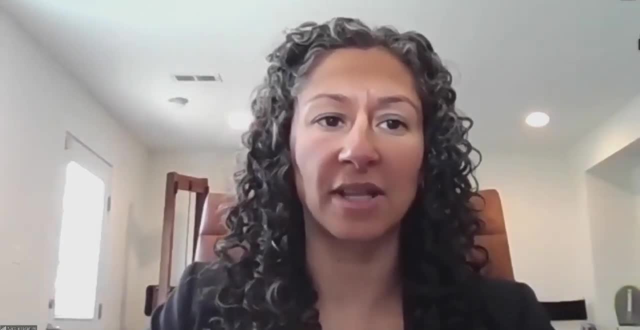 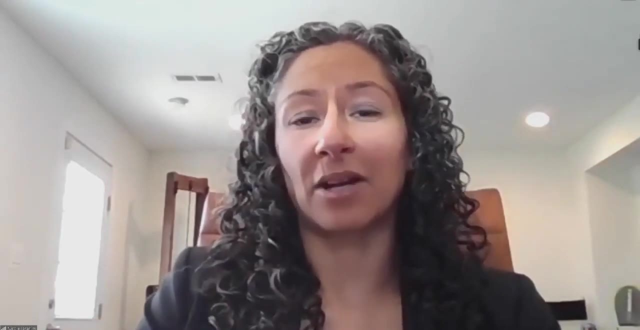 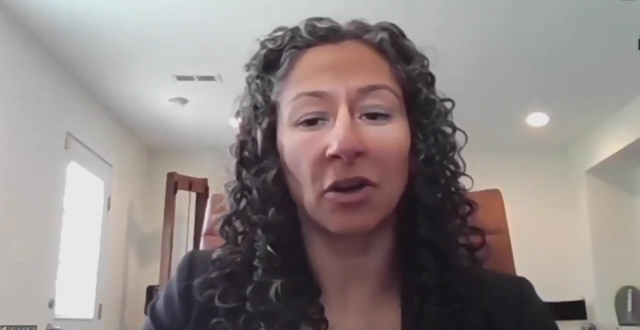 like i said, we've sort of heard from a number of different stakeholders that it not only maybe doesn't add to the add value, but also that it can create barriers, particularly for devices where they're used in emergent situations and obtaining irb approval might be difficult or, you know, can. 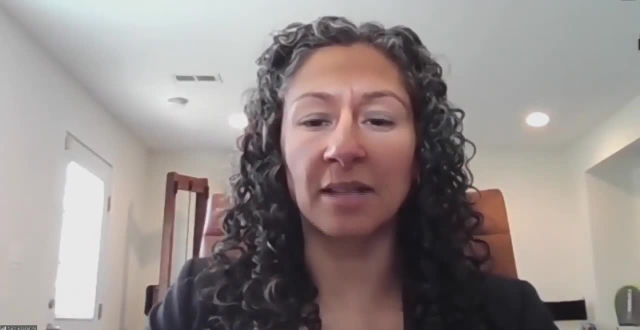 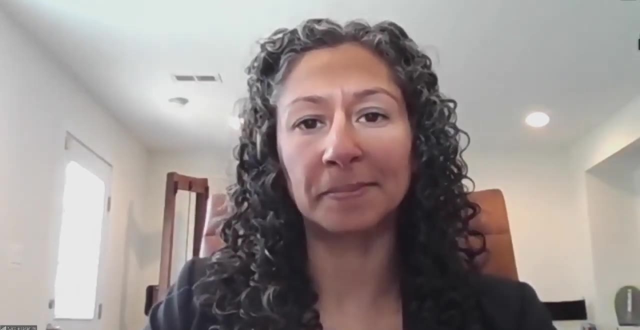 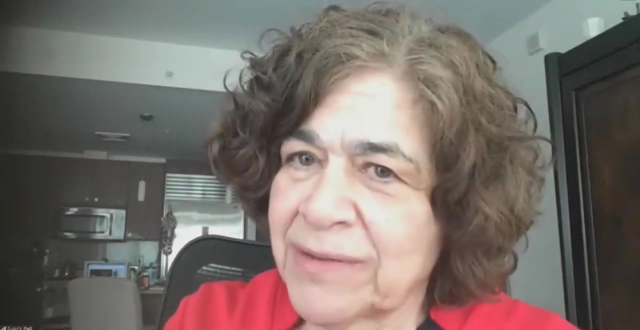 kind of add some level of burden to the process, and so i think it's a, it's a valid question and worth evaluating and something that you know i will certainly take back as well, dr. uh, alpert, yeah, go ahead. add one thing: i i was, i was at ode when we initiated hud and hde, and one: 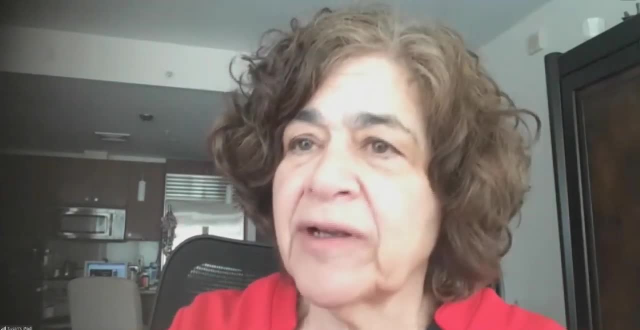 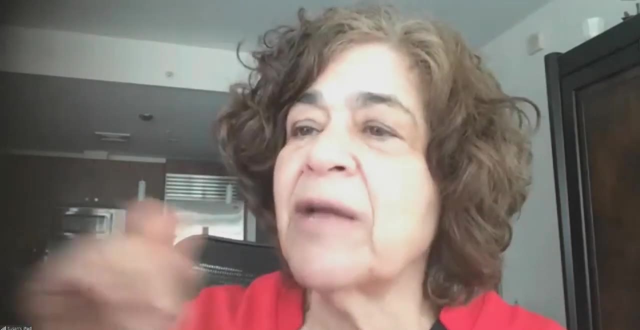 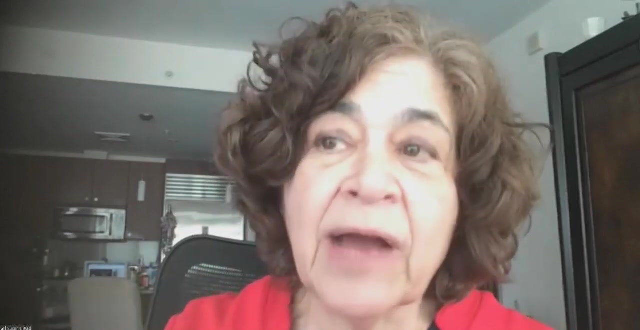 of the goals was that the hospital and the clinician recognize that full efficacy data doesn't exist, that there is some some unknowns in hde and to be able to differentiate, and that we put that in in the beginning, because it's really important when, particularly when you. 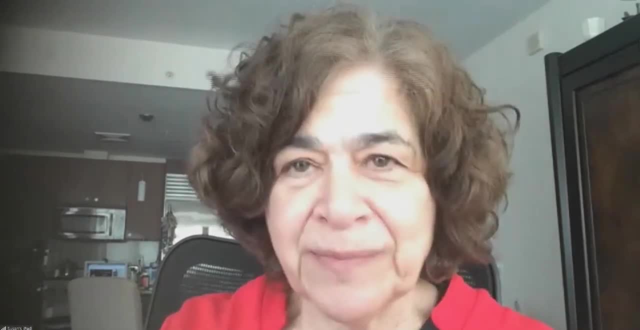 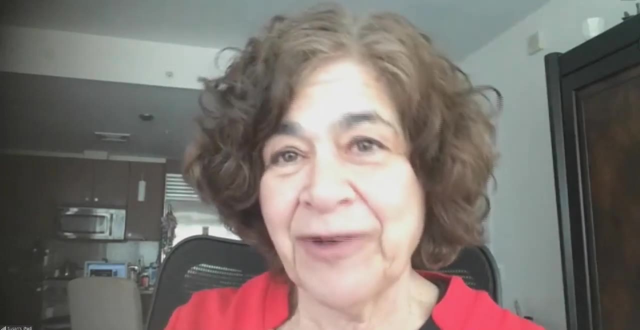 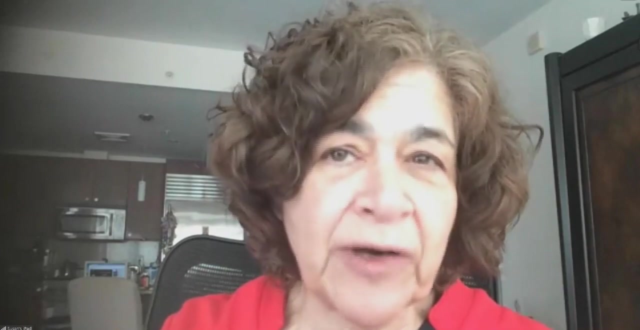 launch something like that that the the end users actually recognize what that data is. they rely on the fda to tell them that things are safe and effective. if there's if there's a question or if there's less data, we felt it was very appropriate for them to know at the beginning of the program. 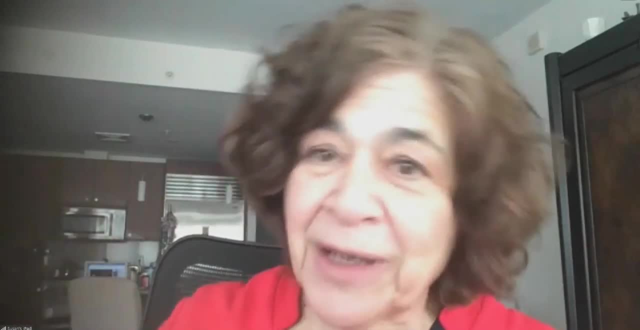 every patient had to start with the first step and then they had to start with the second step and then it happened and we took that route and i'm happy with it. but it was very important that we had a great opportunity to try to bring that into the running and to to start working. 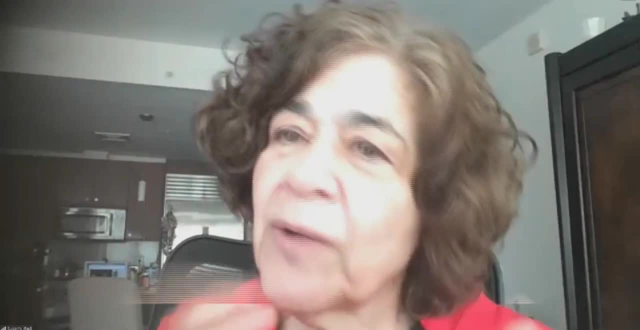 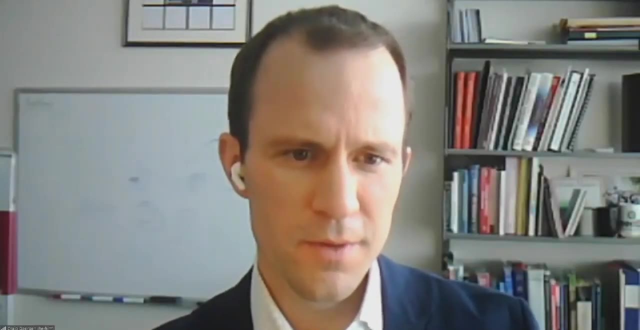 on some of the the the development and the implementation next steps that we were taking. but i think also we should also make sure that we are making sure that we are making the decisions in the right way and that we are ensuring the patient doesn't have the same 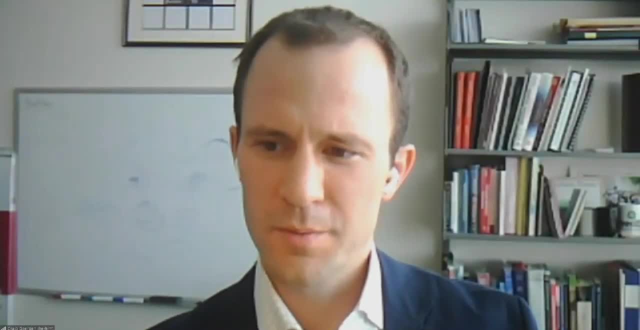 risk, as the patient does. so i think i think that's what's important i would love to talk about is: can we save the patient and do we save the patient? i think one of the things i wanted to talk about was the fact that, because we are using the information that is available to us, we want to 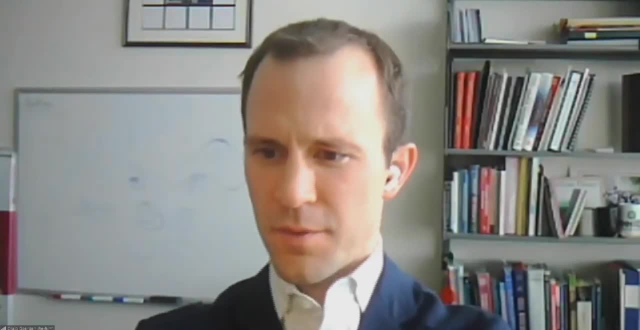 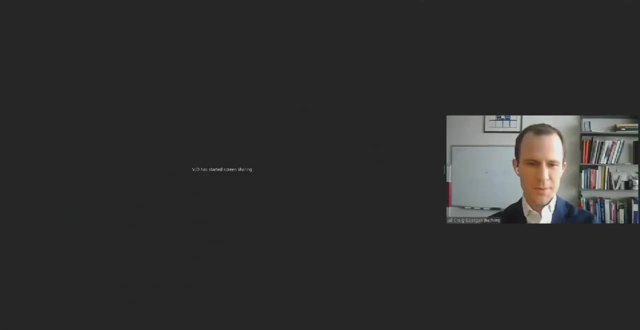 slides and then we'll come back to the IRB question. Dr Heisey from, I think, Med Institute wants to consider from the med device side over IRB oversight and whether it should be kept. but All right, Dr Devlin, go ahead. 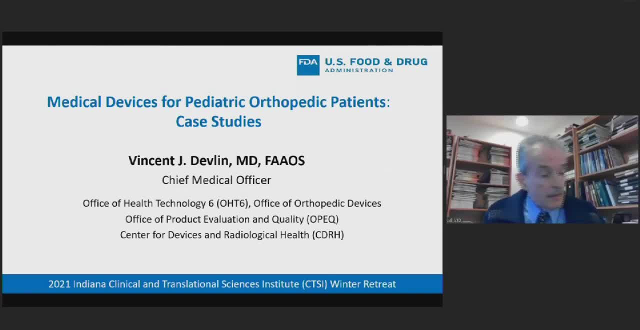 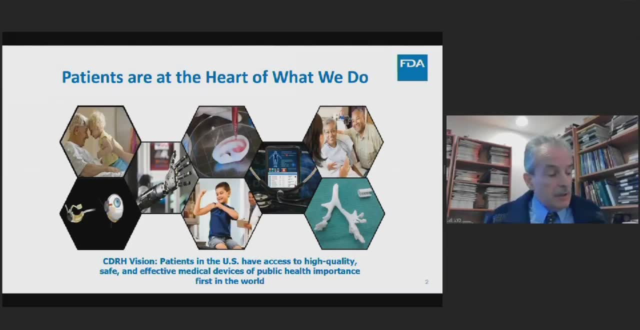 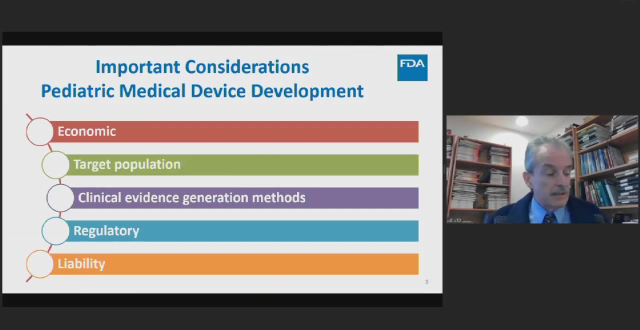 Dr. Okay, thank you for your patience. It's an honor to be here. Thank you for the invitation. Everyone's here for the same reason. as we know, There are unique considerations for pediatric medical devices compared to adult devices, and these considerations generally. 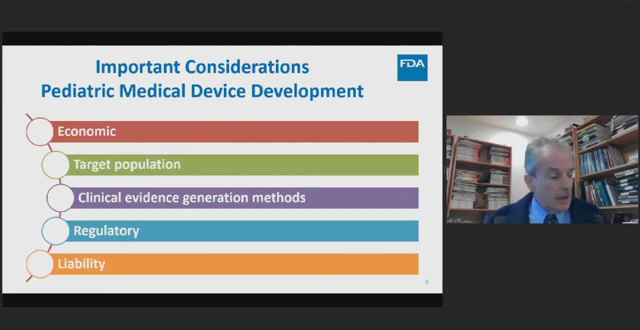 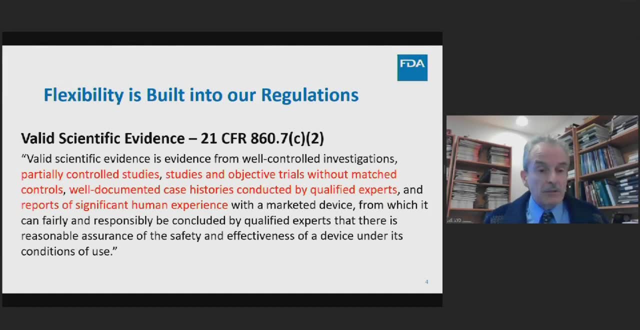 fall into broad categories that we're speaking about. There's a great need for flexibility, as we've been discussing, regarding developing pediatric medical devices and to an extent, this is built into our regulations. You know, our regulations rely on valid scientific evidence. 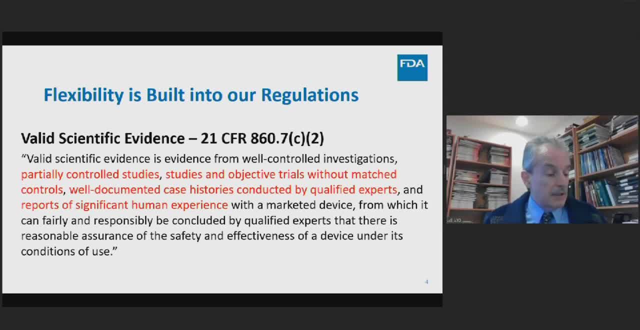 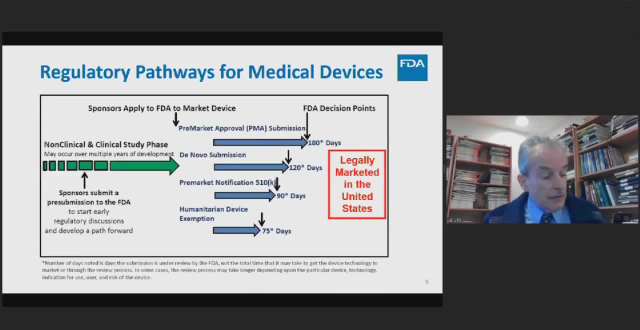 and these regulations allow us to consider many different types of studies and data, including real-world evidence. In our sessions, we've been sharing our interest in reviewing development of novel devices, from the design and development through clinical studies all the way to submission of a marketing application which ultimately enables FDA to review and 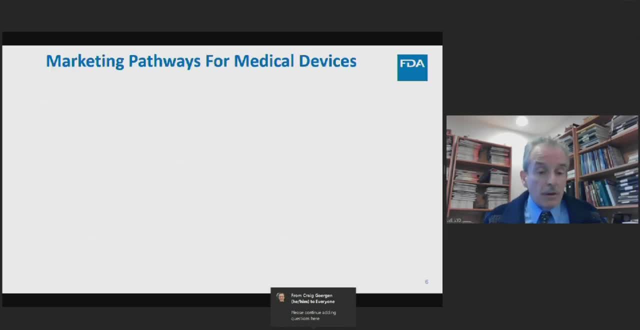 approve these devices. What are the main pathways? We've gone over some of them, but to just run through the main ones, The main ones that all play a role in pediatrics, we would say the 510 pathway. It's most commonly. 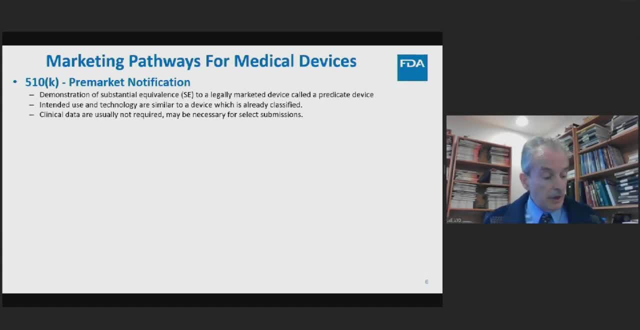 used in the United States. Our goal in this pathway is for the submission to demonstrate that a new device is substantially equivalent to a legally marketed device called a predicate. although performance data are typically required for traditional 510s, Clinical performance data are requested only for a small number of submissions. 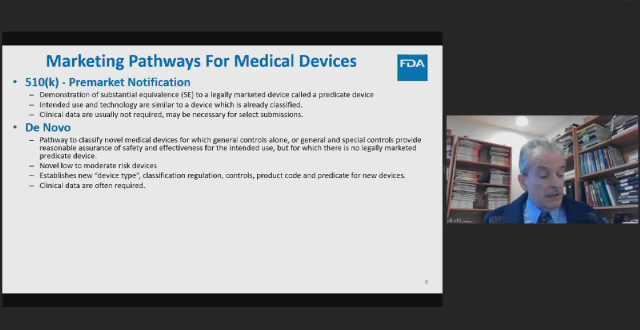 The de novo pathway is used when the risk level of the device does not warrant the pre-market approval pathway but the sponsor and FDA are unable to identify predicate devices to support 510 substantial equivalents. Granting of a de novo classification request authorizes marketing of. 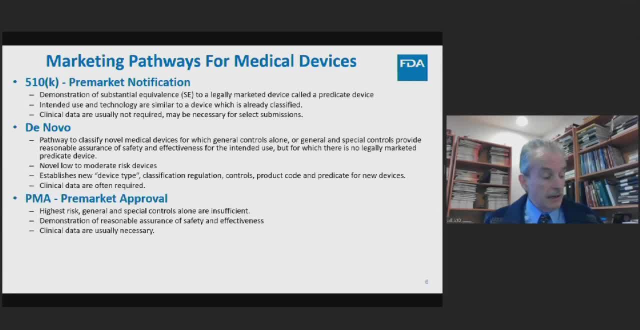 the device in the US and also creates a new classification regulation. The pre-market approval pathway is reserved for the highest-risk devices. It requires that the sponsor provide valid scientific evidence to support a reasonable assurance of safety and effectiveness. The last way to market that we touched on was the humanitarian device exemption. This 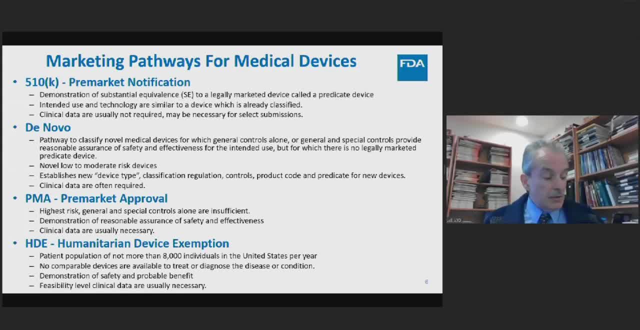 is for medical devices intended to benefit patients in the diagnosis and or treatment of a disease or condition that affects no more than 8,000 individuals per year in the United States. HDEs are exempt from the effectiveness approval requirement governing the pre-market approval pathway, but must show that the probable benefits of the device outweigh the risk. 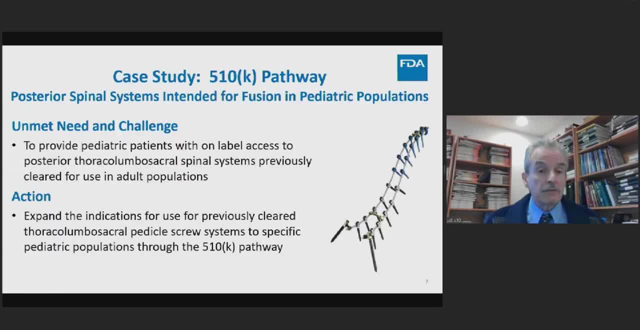 taking into account currently available devices or alternative forms of treatment. I was going to present three case studies briefly on pediatric orthopedic devices to highlight some points about the different marketing pathways. The first case involves the 510 pathway. About 10 years ago there was an unmet need to provide 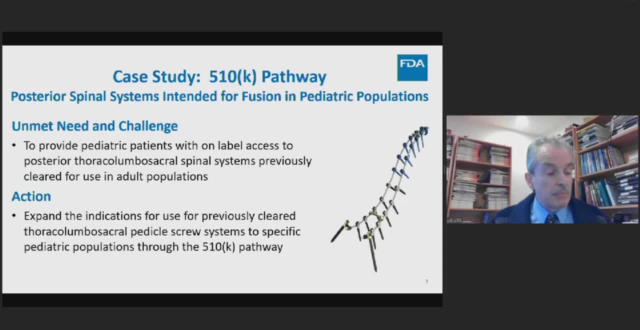 for on-label use of the device with a pre-market approval pathway. The cost was $7.5 for a 3-month adult. The cost was around $3.5 for an individual. on the healthcare facility, The cost was around use of posterior spinal systems, which used pedicle screws for treatment of pediatric. 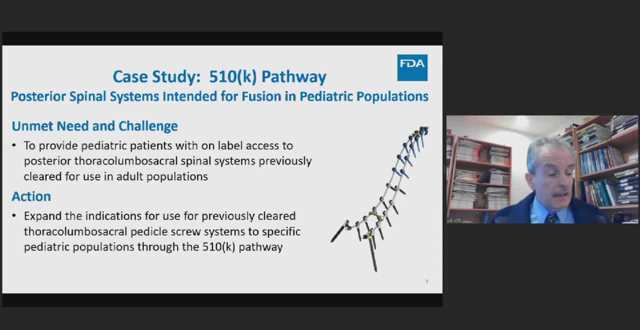 spinal patients. Although these spinal devices had received 510K clearances in adult populations, pediatric populations were not previously addressed. However, the situation was that these devices were widely used under physician-directed use, commonly referred to as off-label use by orthopedic and neurosurgeons across the 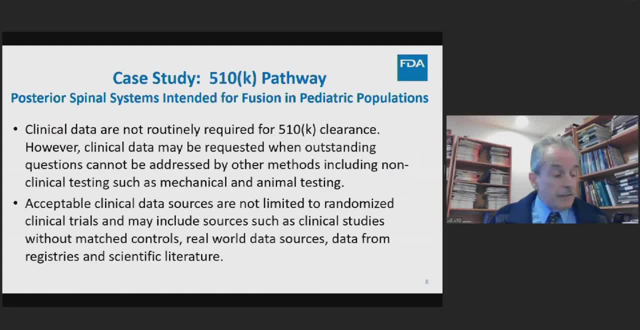 US to treat pediatric patients For 510Ks, we typically need performance data to demonstrate substantial equivalence to a predicate. As I mentioned, this starts with non-clinical data and when these are not adequate, FDA may request clinical performance data. 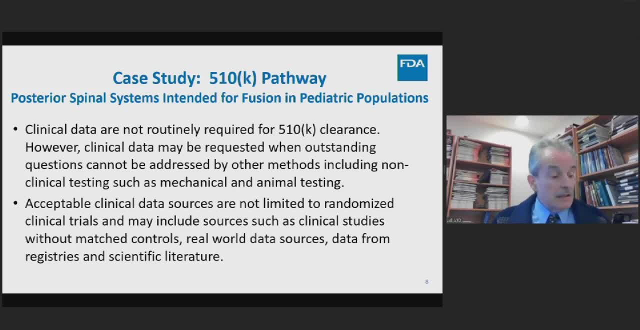 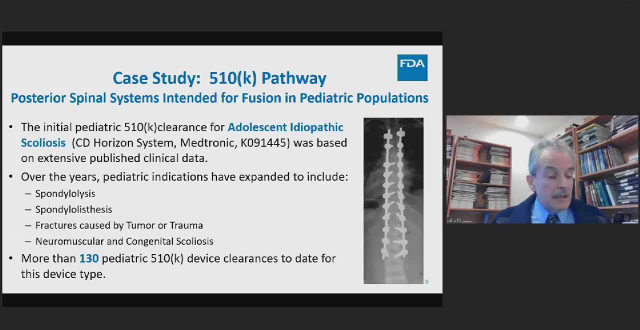 It's important to realize that a request for clinical data does not automatically mean a randomized clinical trial. In this case, our group was able to leverage existing published clinical data to advance the first 510K clearance for pediatric posterior spinal systems that use pediatric pedicle anchors for patients with adolescent idiopathic. 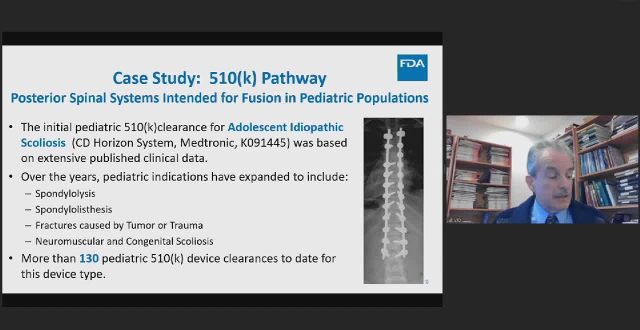 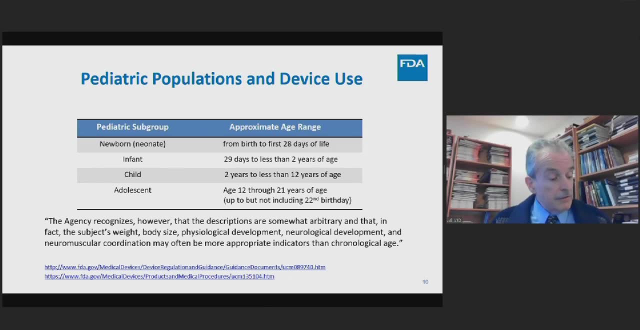 scoliosis. Since that time, we have cleared over 130 systems for use in treatment of a wide range of pediatric spinal disorders. It is helpful to be aware that the Federal Food, Drug and Cosmetic Act defines pediatric populations based on chronologic age. 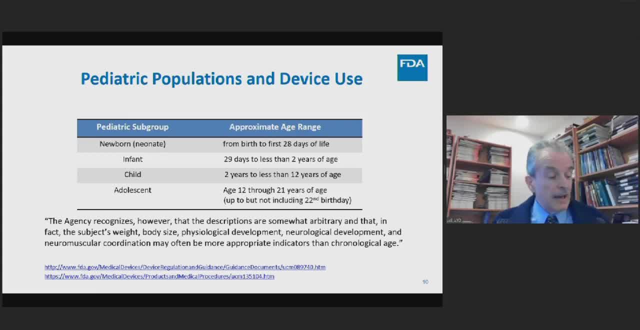 Pediatric patients are those persons aged 21 or younger at the time of their diagnosis or treatment. Pediatric subpopulations are further categorized as newborns, infants, children and adolescents. However, in orthopedics, other factors such as skeletal maturity and growth have an equal 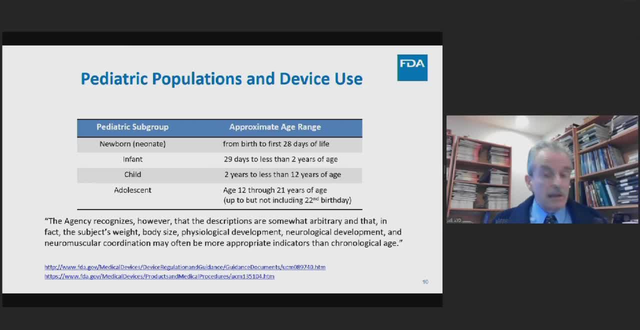 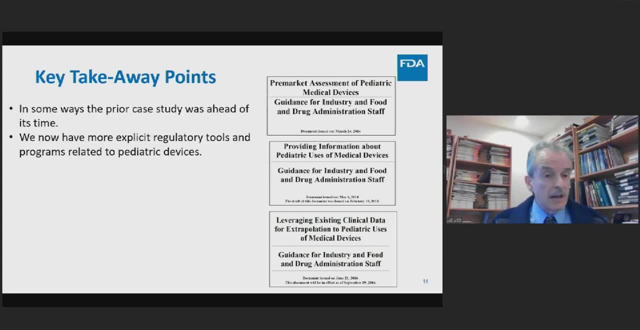 or greater impact on device performance when compared to chronological age. So some of the takeaway points from this case: In some ways it was ahead of its time. We now have more explicit regulatory tools and programs related to pediatric device development. Valid scientific evidence to support device approval can come from multiple sources, and 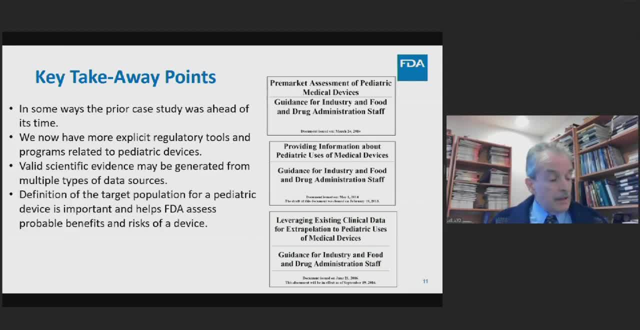 multiple types of data. It's very important to carefully define the target population for a pediatric medical device And finally, reaching out to FDA and interacting early is strongly important. Thank you, Thank you. There are two additional authors or courses about pediatric scoliosis treatment that are: 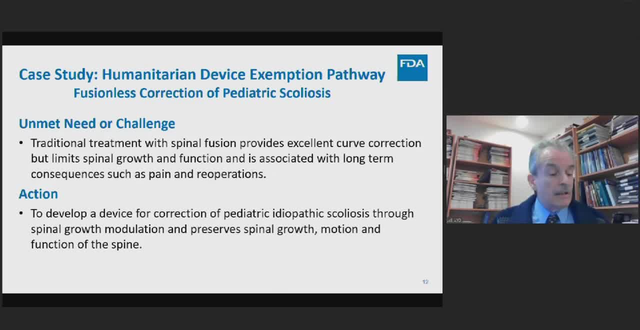 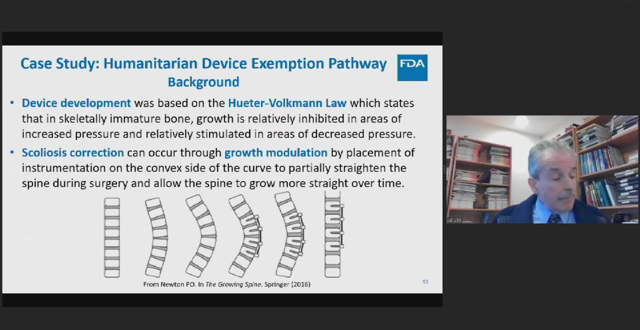 가족 or spinal fusion. While curve correction is excellent and reliably achieved, the treated section of the spine does not function as a normal spine as it does not bend or grow, and additional surgery may be required to address both short and long-term events. Since the 1950s, there has been great 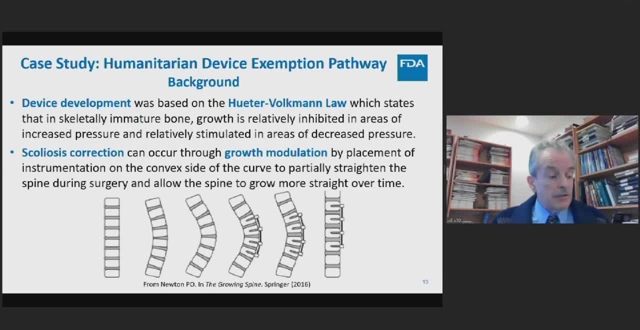 interest in developing reliable methods for fusionless correction of spinal curves. It was known that in skeletally immature patients, that growth of the spine could be modulated based on understanding of how bone grows in relation to mechanical forces. This has been referred to as 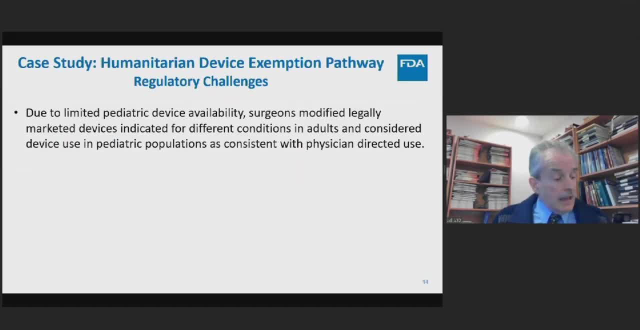 due to Volkman's law or principle. Initial device development in this area was somewhat chaotic, with surgeons developing many different types of devices by modification of devices legally marketed for use in adults and using these to treat pediatric patients in their clinical practices. There was a lot of interest in developing new methods for fusionless correction of spinal curves. 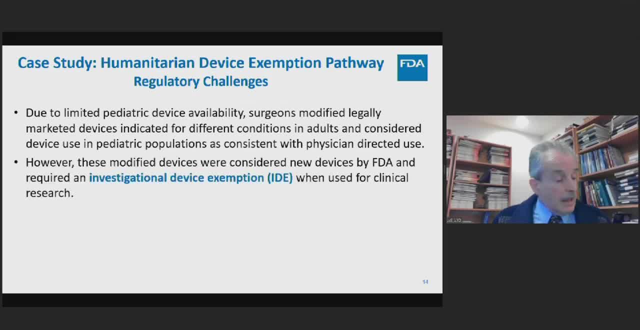 There was a lot of interest in developing new methods for fusionless correction of spinal curves. However, there were limited data available to guide this use and no organized data on long-term outcomes of such treatment, and clinical research to evaluate these new devices required an 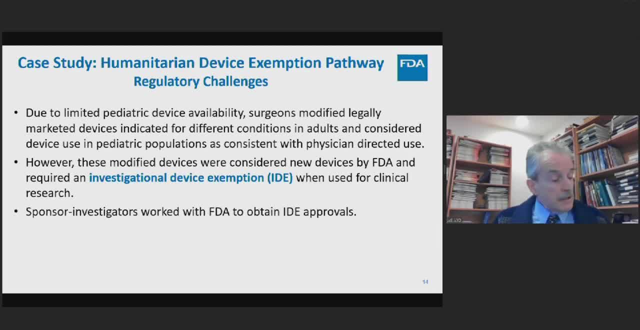 investigational device exemption, As physicians were initially reluctant to pursue these studies. FDA worked closely with physicians, medical societies and the scoliosis community to address this challenge. The first development was that some leading physicians stepped up and became sponsor investigators and worked with FDA to obtain IDE approvals to study new devices at 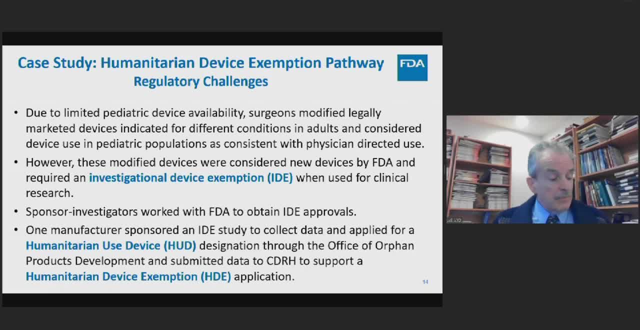 their institutions. Subsequently, one device manufacturer sponsored an IDE study which led to an application for a humanitarian use device designation and subsequent submission of data to CDRH in support of a humanitarian device exemption. The clinical evidence consisted of a single-center study with two-year follow-up and provided adequate 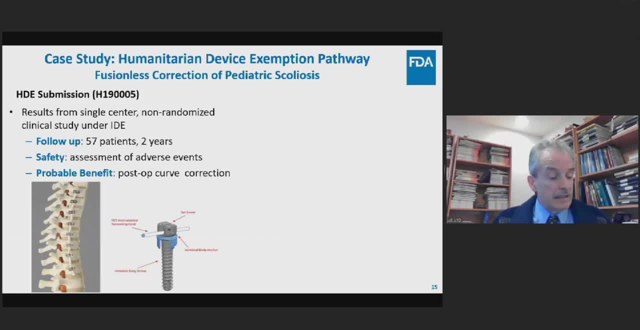 data to support the safety and probable benefit of the device. As the treated patients were skeletally immature and the study endpoints were based on two-year data, there was some uncertainty regarding the ultimate treatment outcomes, as many patients were still growing and their curves had. 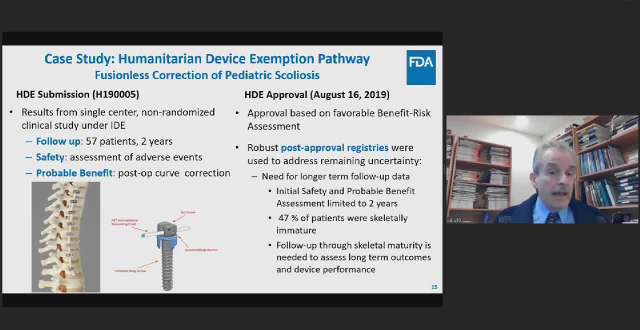 not been assessed at the end of their skeletal growth. As these devices had shown great benefit to patients, it would not be in the interest of the patient's health if they were not treated in the right way. In addition, there was an interest of patients to delay their availability to await these. 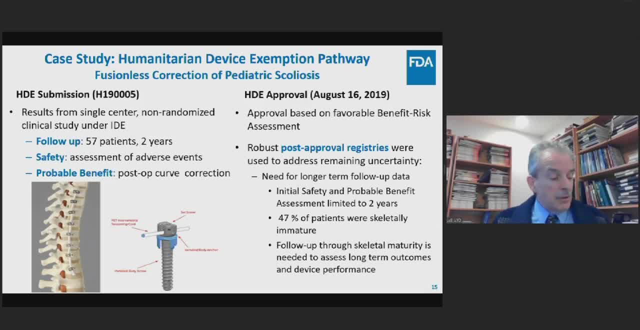 longer-term outcomes. Through creation of robust post-approval registries, CDRH was able to balance pre-market and post-market data collection requirements, and this led to marketing approval of the first pediatric spinal device for fusionless correction of pediatric idiopathic scoliosis in 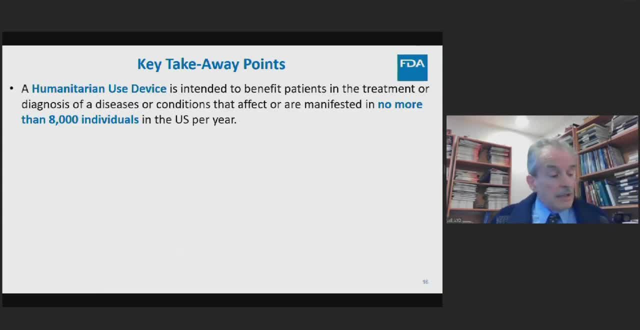 2018.. So the takeaways from this case would be that the humanitarian use device is a intended to benefit patients in the treatment or diagnosis of a disease or condition that affects is manifest in no more than 8,000 individuals in the US per year. Marketing. 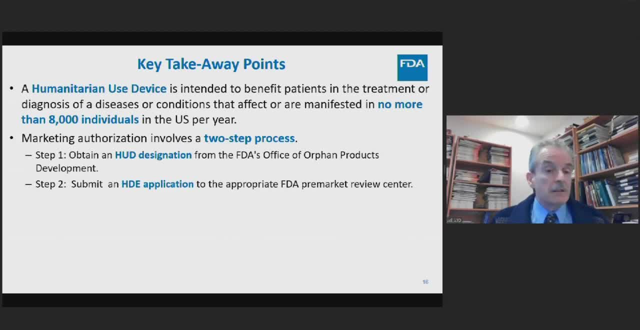 authorisation involves a two-step process. First, obtain a humanitarian use designation from FDA's Office of Orphan Products. Step 2, submit an HDE application to the appropriate FDA pre-market review or pre-market review version of the FDA Optimiz3 cabinet and extract custody and. 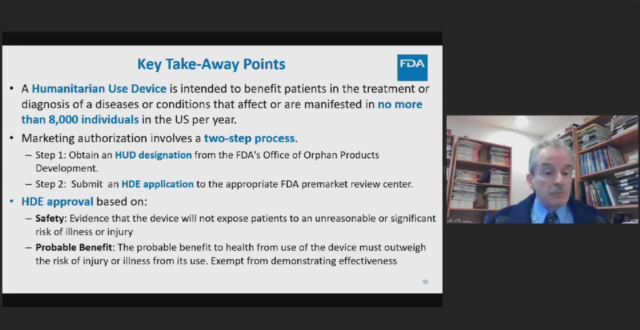 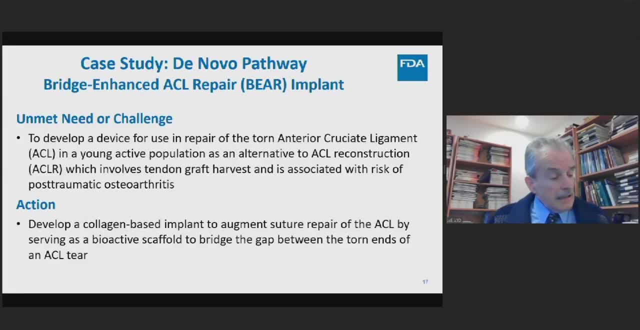 market review center. The HDE approval, as was mentioned, is based on safety and probable benefit. The last case I'll present involves a de novo classification process or pathway. It is about addressing the unmet need to develop a novel device for use in the repair of a torn anterior. 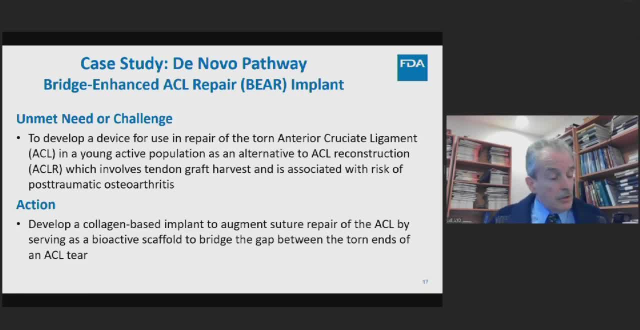 cruciate ligament in a young, active population. Suture repair alone of acute ACL injuries is associated with poor healing rates and outcomes. A new device solution was needed to serve as an alternative to ACL reconstruction. the current treatment, which involves tendigraft harvest and 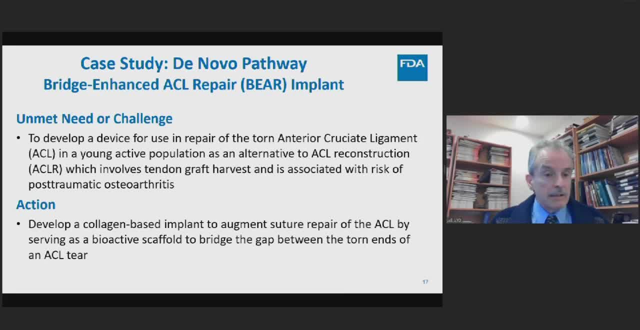 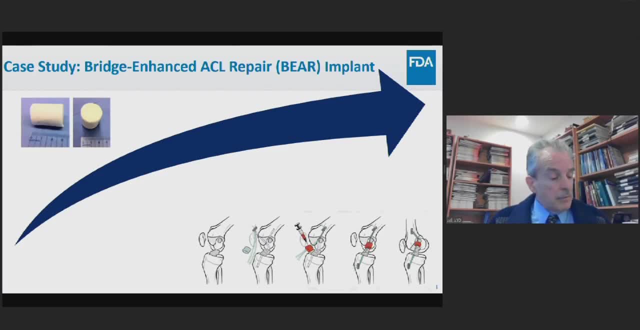 is associated with risks of post-traumatic osteoarthritis. This led to development of a new device, a collagen-based implant, to augment suture repair of the ACL by serving as a scaffold to bridge the gap between the torn ends of an ACL. 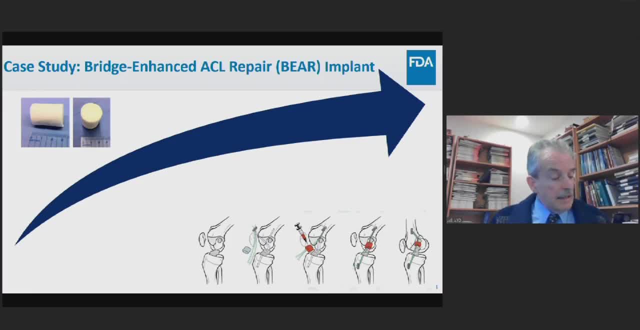 This bridge-enhanced ACL repair implant is a cylinder-shaped device. as shown in the upper left, It's composed of collagen and extracellular matrix derived from a bovine source. During the surgical procedure, as shown in the lower right, the implant is used with autologous blood to 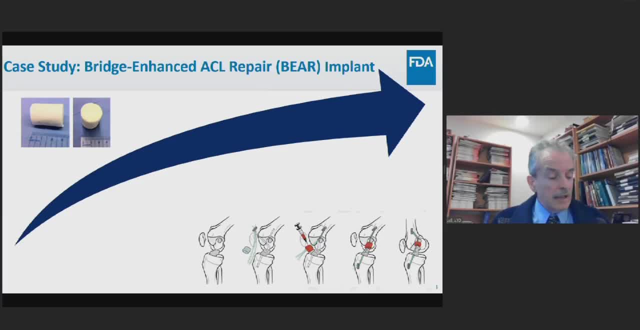 stabilize the gap between the torn ligament ends and protect the biologic repair process as it is resorbed and replaced by repair tissue. During the development of this device, FDA engaged with the sponsor at each of the key stages of product development. 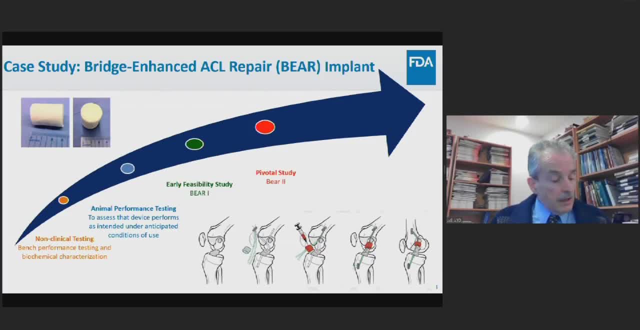 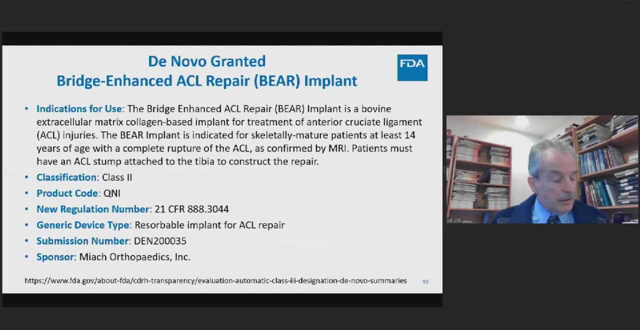 The device progressed from an early feasibility study to a pivotal study, and positive results led to granting of a de novo classification request in December 2020.. Granting of a de novo classification request provides authorization to market the device. In addition, it classifies the device into Class 1 or Class 2 and creates a new classification regulation and the new device type, which is now regulated through 510. 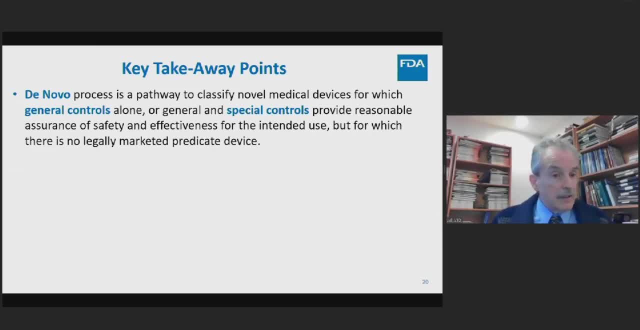 The key takeaway points from this case are: the de novo classification process is helpful to classify novel devices for which general controls alone, or general and special controls, are able to provide a reasonable assurance of safety and effectiveness for the intended use, but for which there is no. 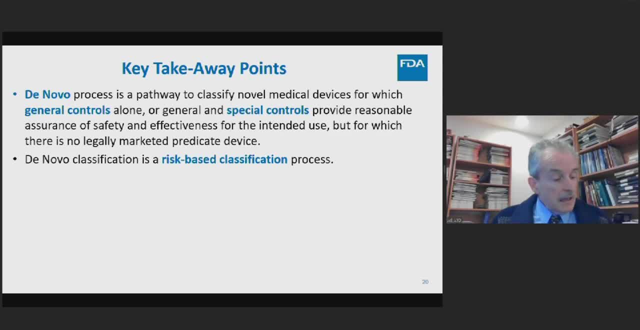 particularophilically marketed predicate device? Is it a risk based classification process and outproduced marketing authorization? in establishing a new classification regulation, Devices are classified into Class 1 or Class 2 based on benefit, risk assessment and risk mitigation measures. The new devices mentioned may 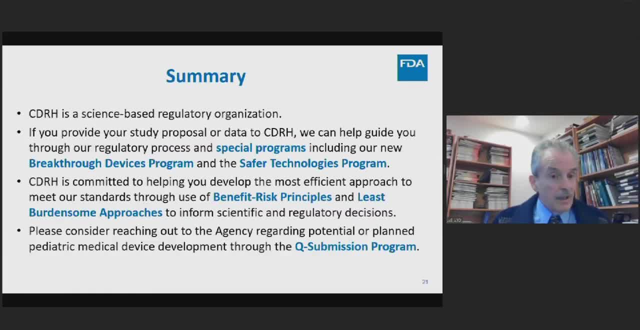 ��목ув 갖죠 Now serve as a predicate for other devices. CDRH is committed to working with everyone here and everyone in the audience Seeing no As a science-based regulatory organization. if you bring your data and proposals to CDRH. 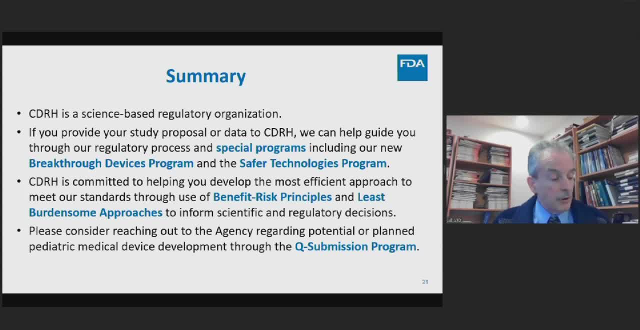 we can guide you through our regulatory processes and our special programs. These include our new Breakthrough Devices Program and the Safer Technologies Program. Also consider reaching out to us early through the Q-Submission Program for assistance regarding potential or planned pediatric medical device development efforts. 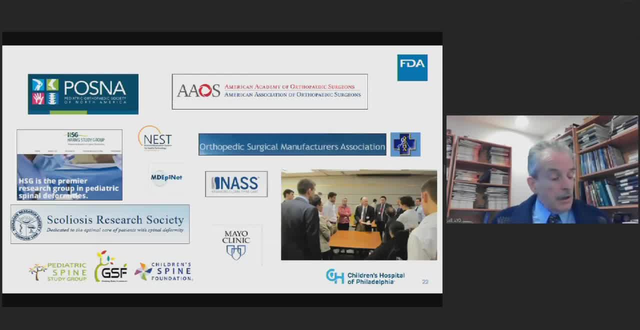 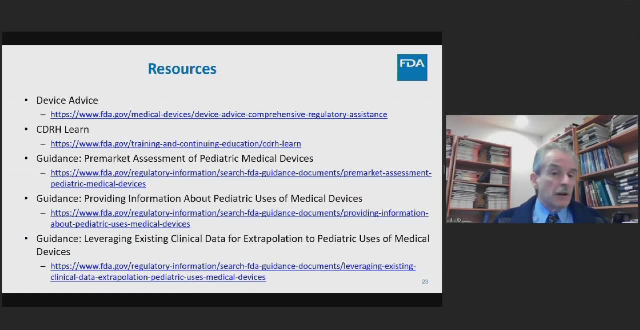 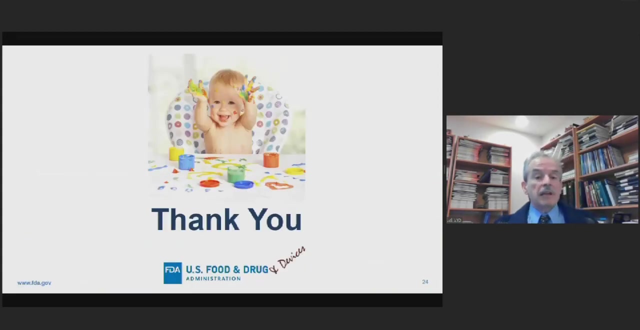 We're also very interested and work diligently to outreach to everyone who's developing pediatric medical devices, and here are some of the stakeholders we've interacted with over recent years. I've provided some helpful resources regarding pediatric device development and regulation and I thank you for your time and attention. 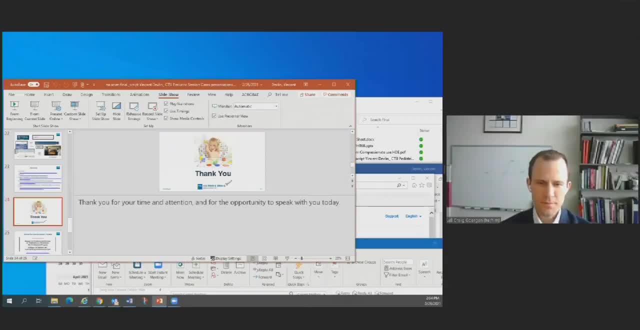 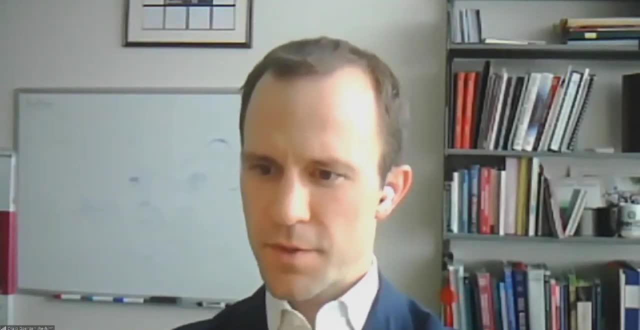 Thank you very much, Dr Devlin. That was wonderful. Go ahead and stop sharing, yeah, so that we can go back to more of the discussion section. now. To kind of wrap up the conversation, then, with the IRB oversight, Ted Heiss. Dr Heiss is. 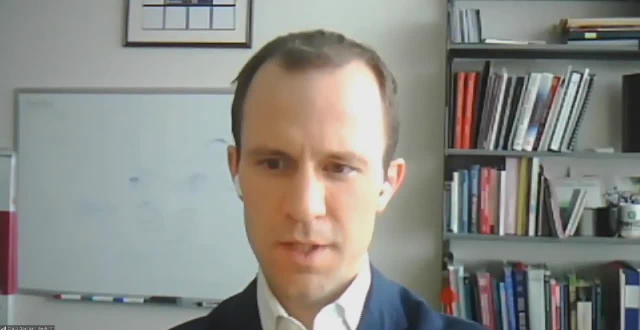 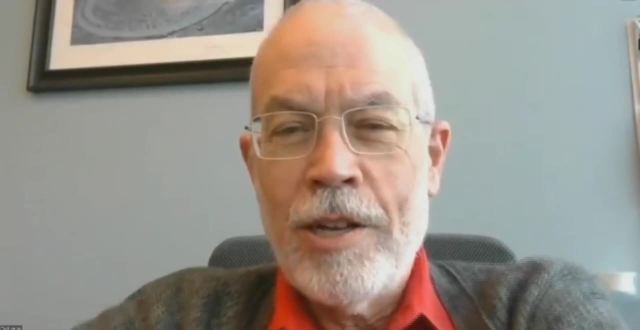 on from MedInstitute. Are you on, Ted? Would you like to answer your question regarding central IRB? Yeah, go ahead, I am, Can you hear me? Yes, So our experience from the industry side has been the same as Dr Denham mentioned. 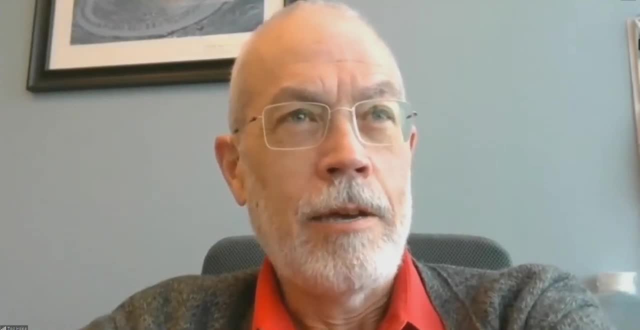 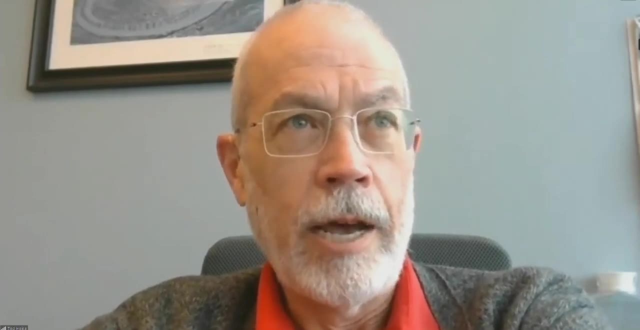 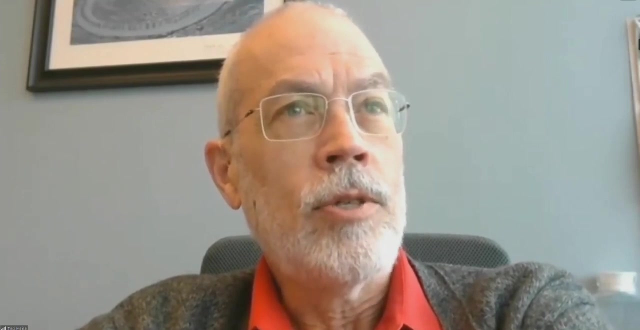 And we've found that hospitals tend to be confused often about the requirement and what the purpose of it is: getting the IRB oversight of access for use of an HTE And I think, in addition, when it's in the setting of a condition of approval study that may be required as part of the HTE. 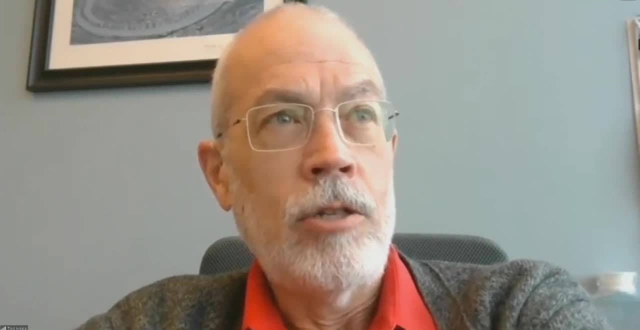 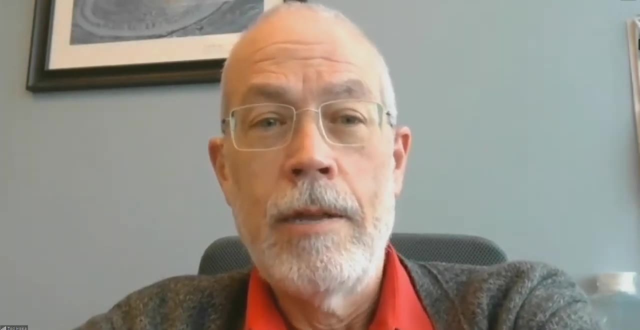 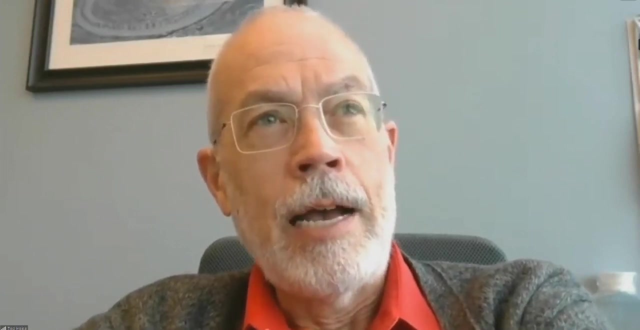 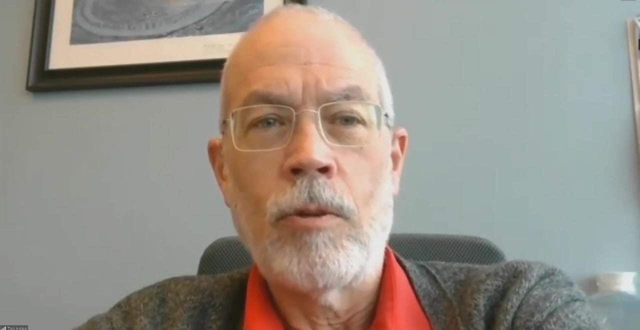 that adds not only additional burden but some additional opportunity for confusion at the hospitals. They often don't quite get why they have to do two IRB approvals in the process, And so I guess for those reasons I would agree with the other speakers who have suggested that the topic maybe warrants some re-exploration. 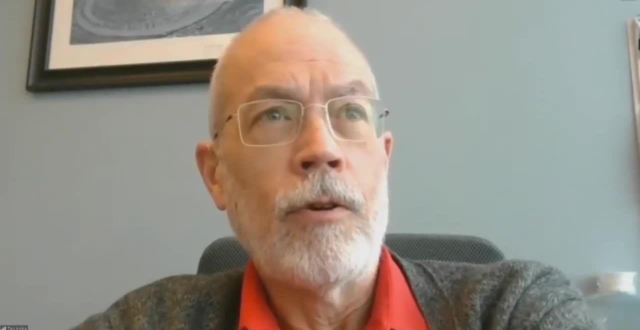 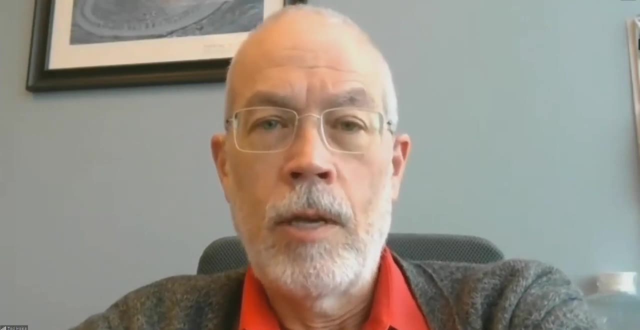 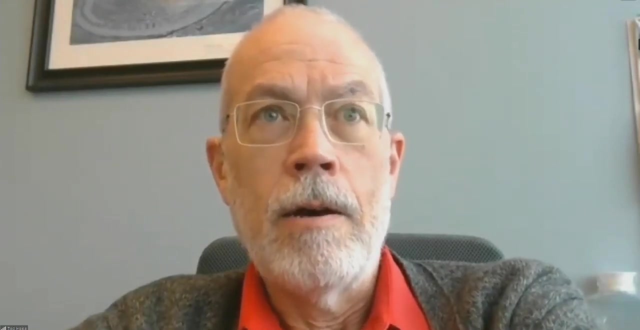 And I completely get the reason that it was put in in the first place, And I guess my follow-on comment would be that if, after discussion, it seems that there is value in keeping some IRB oversight, perhaps it could be simplified a bit by mandating use of a central IRB for the process. 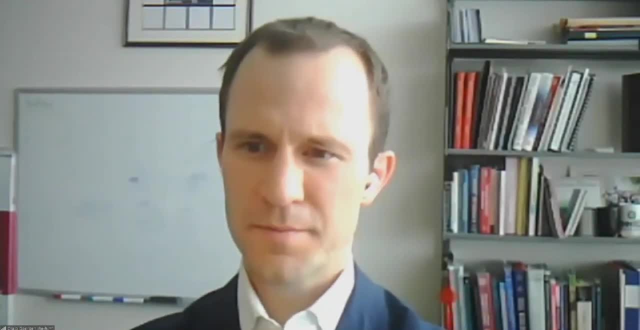 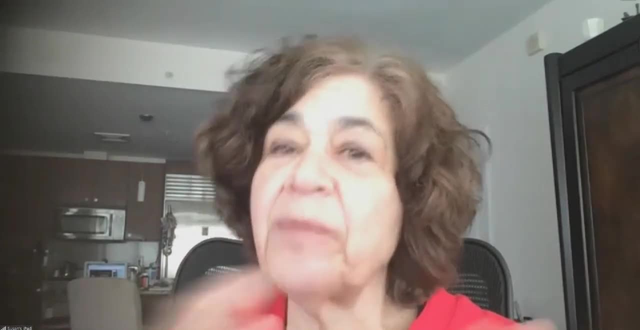 The panelists want to have any comments on that. Dr Alford, Yeah Comment. So central IRBs are a great idea, but individual IRBs still need to work with the central IRB and agree, Agree, So it's. 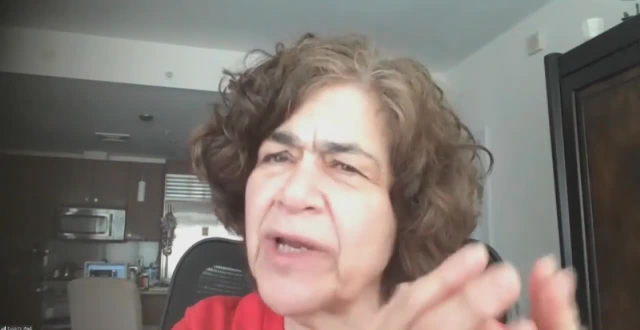 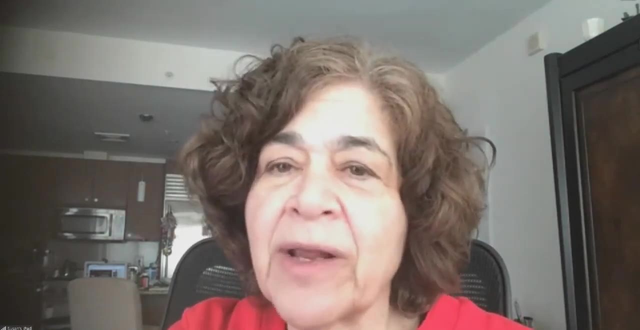 it doesn't completely take it away, although it does take away the initial, the initial review process. So I think you know that's. that's something worth we're thinking about, And it may be also that we should be speaking to. 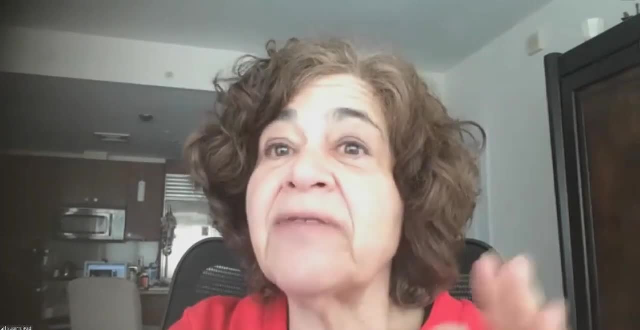 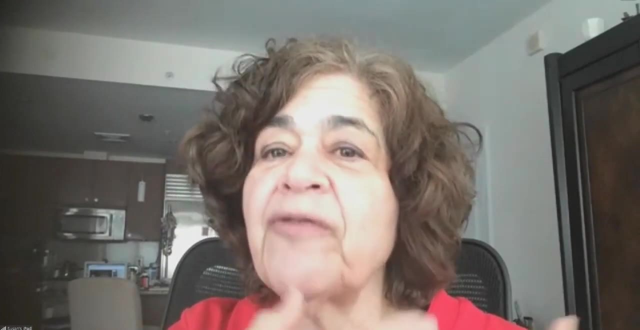 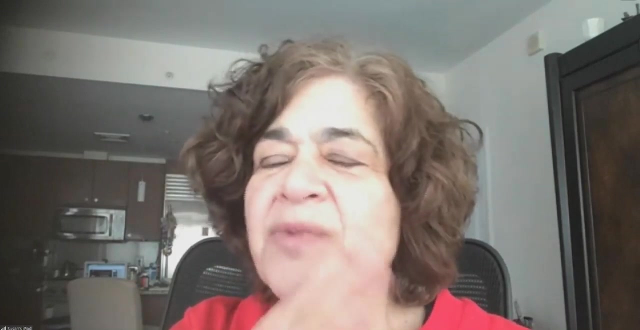 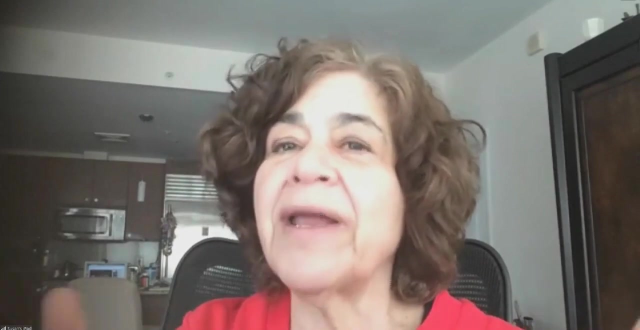 I'm going to forget the name, the H, the HHS level folks who deal with IRBs, to make sure that we do some education, to provide some educational information on their website about HDEs, which would be would be really helpful, as well as having some conversation at the annual IRB meetings about what an HDE means and why there's an involvement of IRBs. 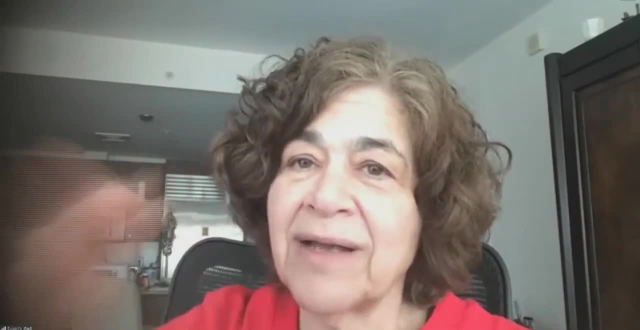 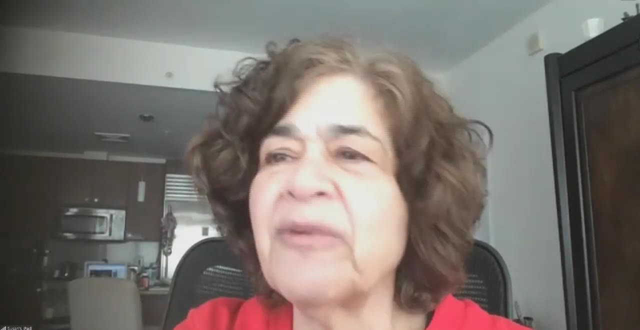 That those are just some things that that could be thought about as a stepwise, a stepwise way to make sure that we still have the oversight, but but take some of the burden off by doing broader education. Yeah, that makes sense. Yeah. 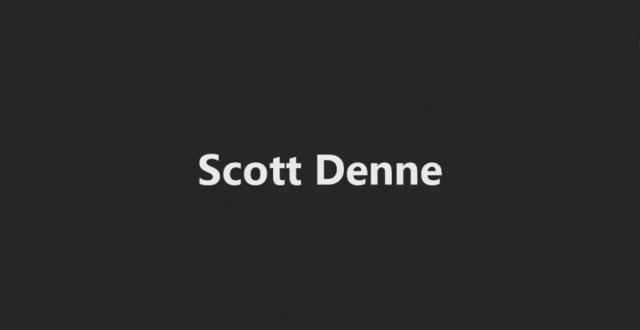 It's a good go ahead. Just just a brief comment, just in response to that. I mean, we we go over that every time it comes up with the HDE. I just don't know that it's actually providing the oversight that you expected to do. 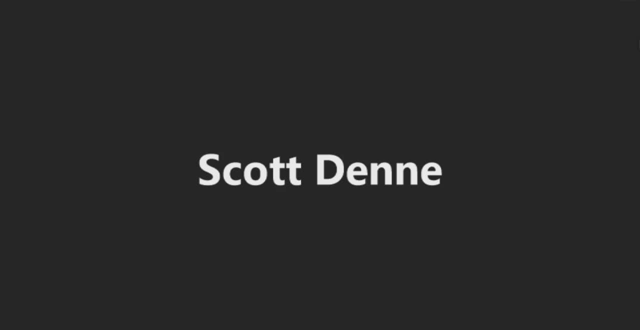 It. so I I mean to your point about letting in, letting physicians know that it's you know that it's not fully approved. I think there are other ways to do that, So I I will leave it at that. 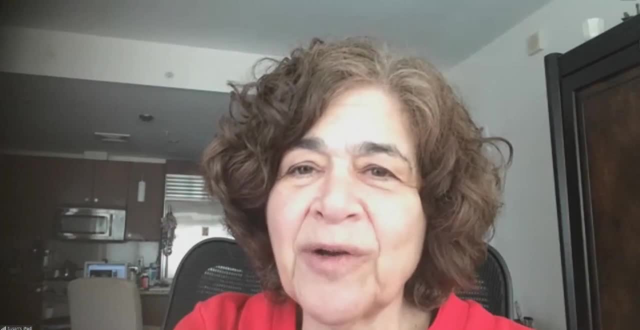 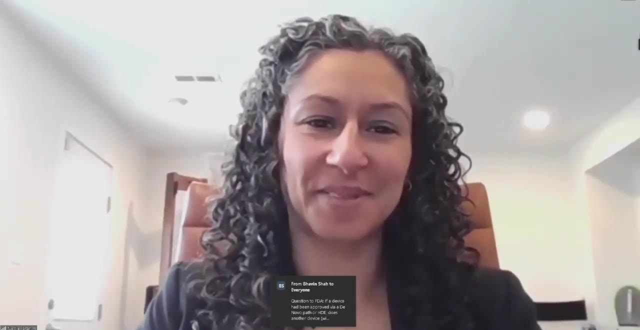 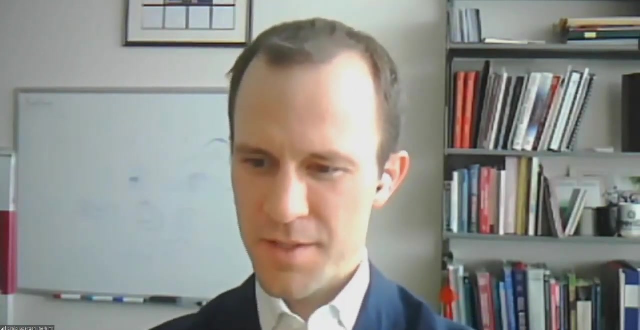 We need. we need to have Nicole take that back to the. Yeah, exactly, Yeah, certainly, I will, Yeah, Provide that feedback. Bobbin's got a question. Bobbin, would you like to unmute and ask in person? 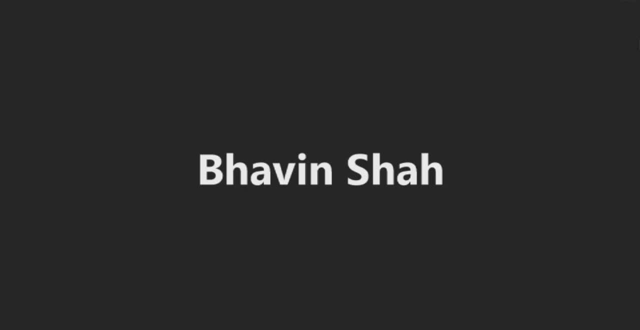 Yeah, thank you. Thank you for this opportunity as well. Sure, So I wanted to understand if an, if a, if a previous device had gone through a de novo pathway or an or an humanitarian device exemption pathway and now another company, or even the same company, has come out with with a slightly improved technology and would like to pursue that device, would they be required to go through a PMA or an HDE all over again, or is that a chance that it could also be a 510K? 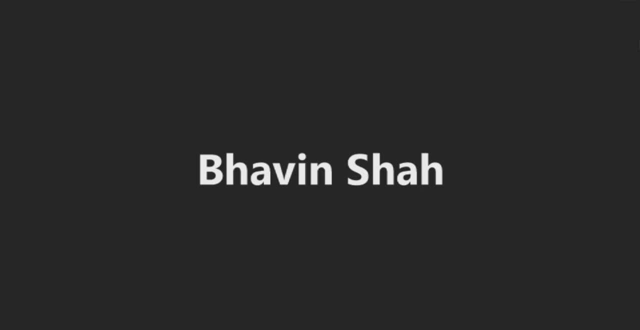 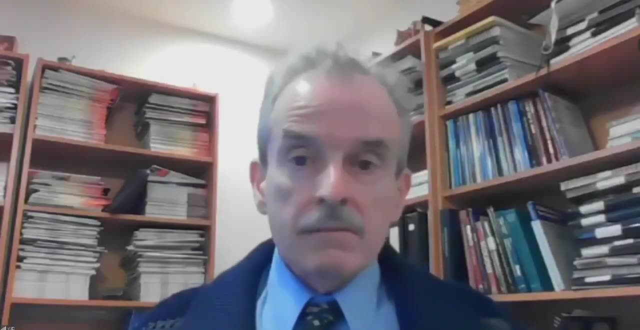 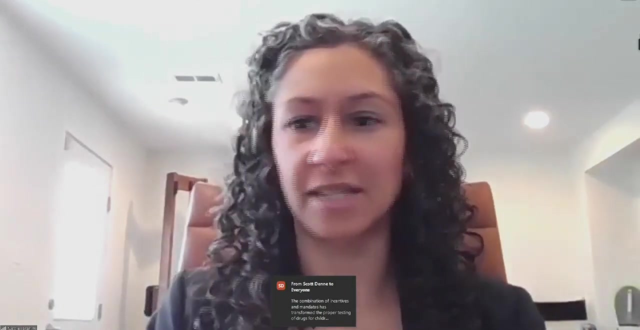 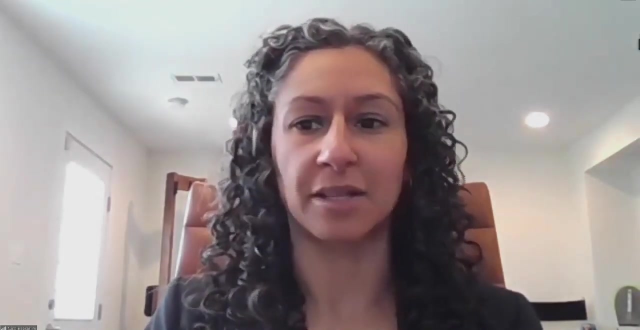 Yeah, I would like to tackle that question. Go ahead, Go ahead. So I think there are a couple of things, a couple of different scenarios that you've mentioned here. So, if a device has gone through the HDE pathway and has received HDE approval, 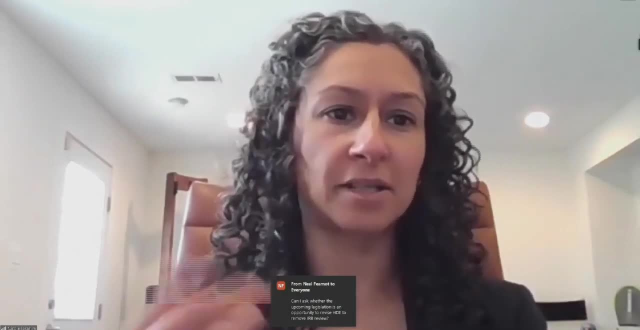 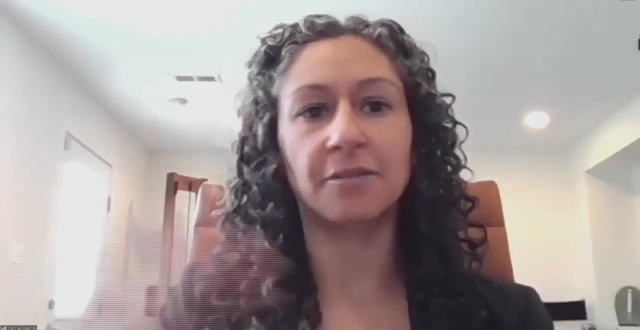 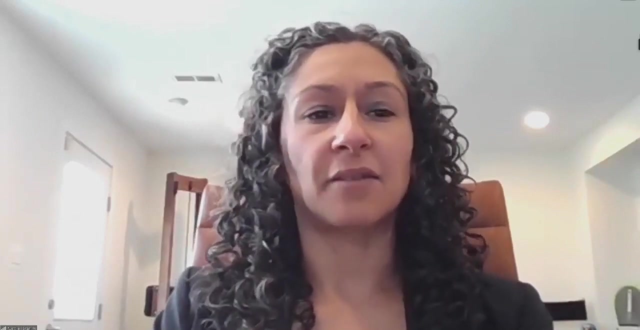 if they make changes to their device and it's it's an improvement, it has the potential to just be a supplement to the original HDE. If indeed it's a different device or maybe a different manufacturer developing a device that is an improvement and it's of the same device type, treating the same patient population for the same indication. 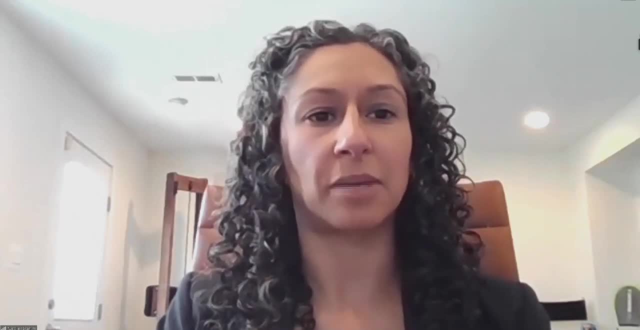 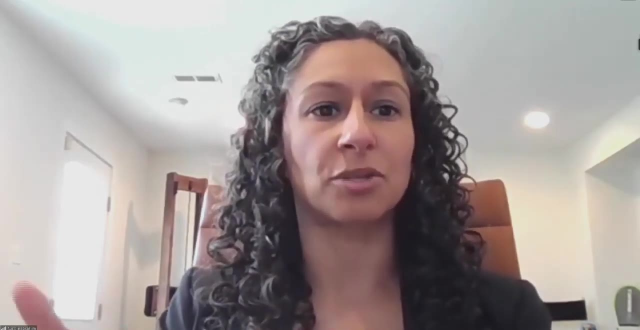 then they would not be eligible for the HDE pathway, because HDE is intended for devices for which there's no alternative. So the only other option would be either a 510K or PMA, depending on if it's a class two or a class three device. 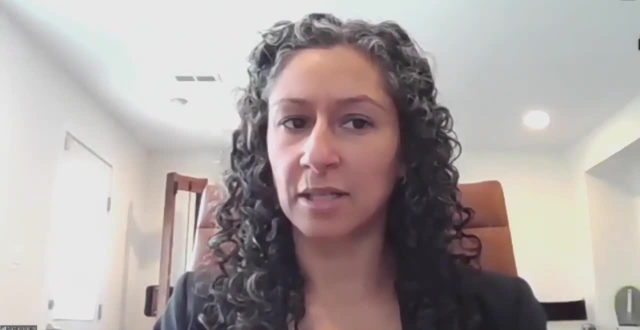 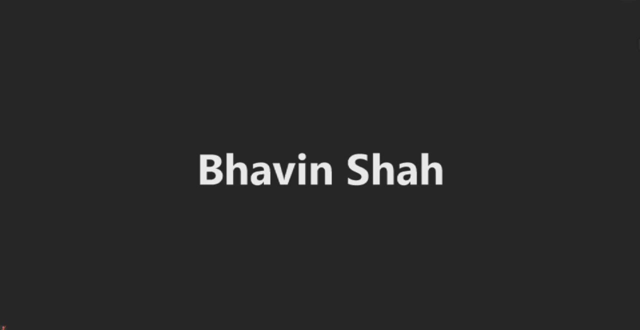 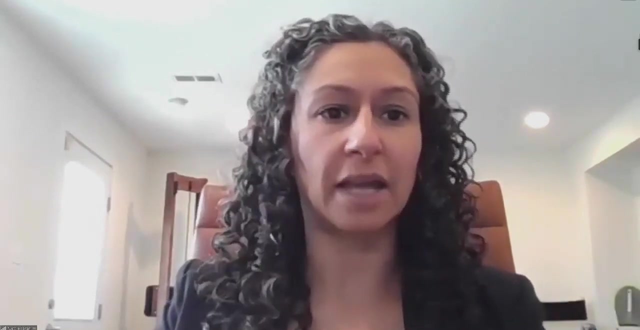 I think I hope that addresses the question. Yes, thank you, And I will say- I'll maybe just add one other comment- that if the second company decides to go through a PMA or a de novo pathway, then the company that holds the HDE. 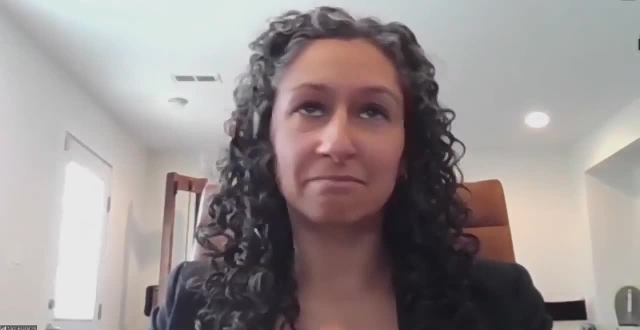 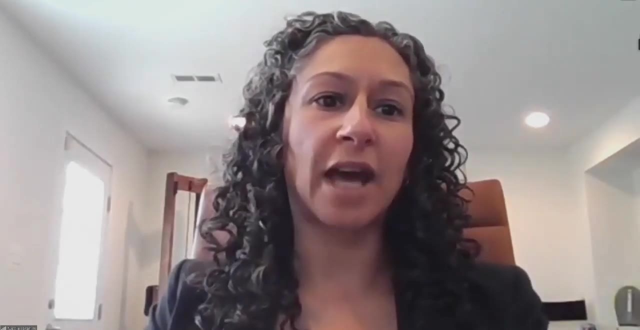 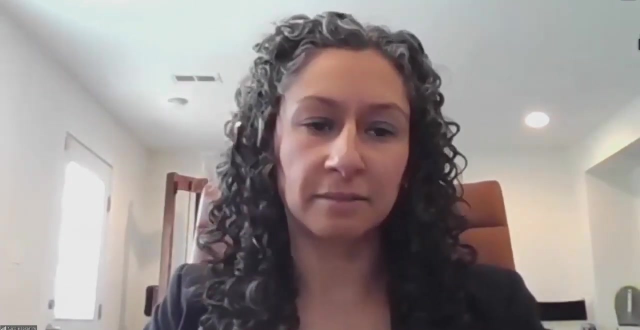 their HDE would no longer be valid, I suppose because now there is the, now there are two devices available to patients, and so they would have to then submit for a traditional marketing submission, either a PMA or a 510K. Very interesting. 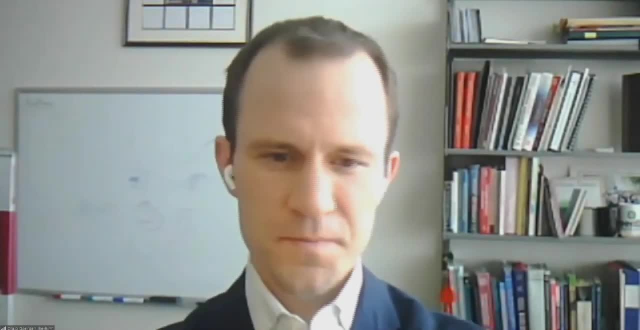 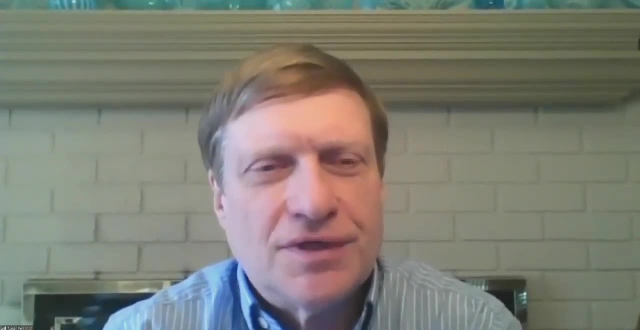 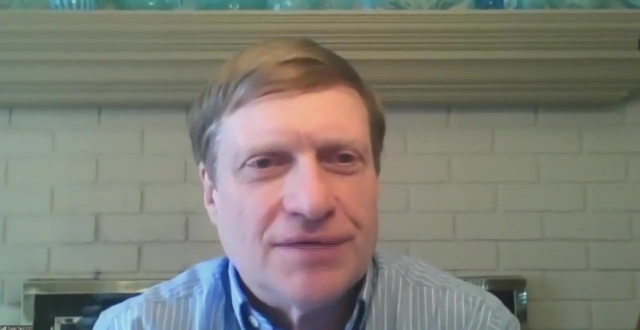 Dr Fearnot, do you want to unmute and ask your question about legislation? Yeah, we just talked about um HDE and you know that HDE regulation has, or the legislation has, been changed every few years, every several years anyway, since it was started. 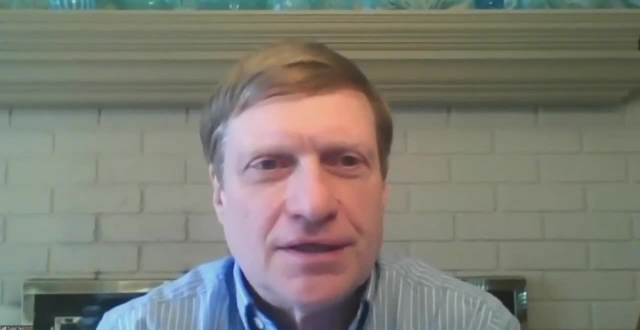 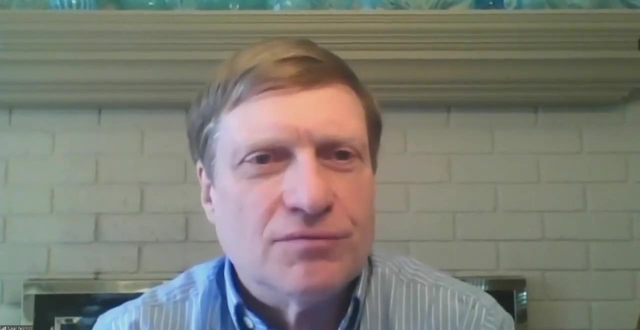 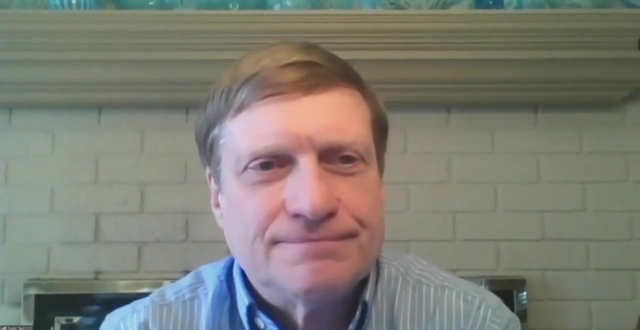 And I wonder if this upcoming manufa negotiation has any chance of including fixes to the HDE that would remove a couple of those elements that really haven't been serving us well. Thank you, Any comments on that? Dr Alpert, I'd say that there's the option. 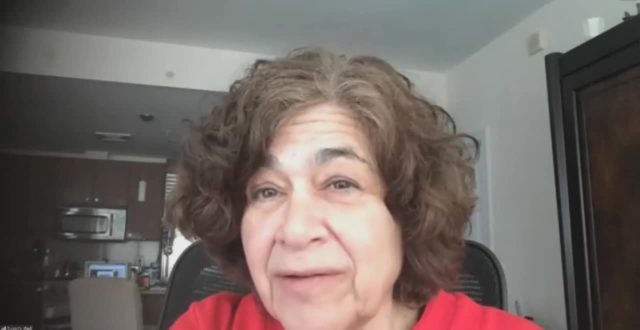 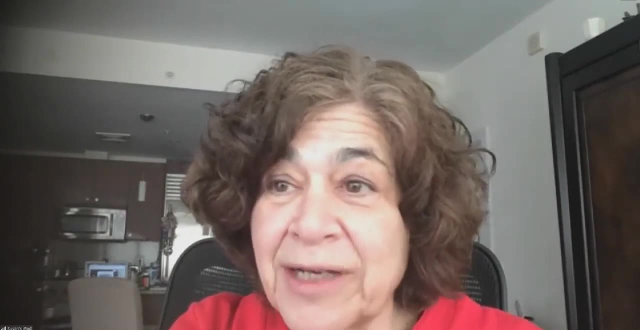 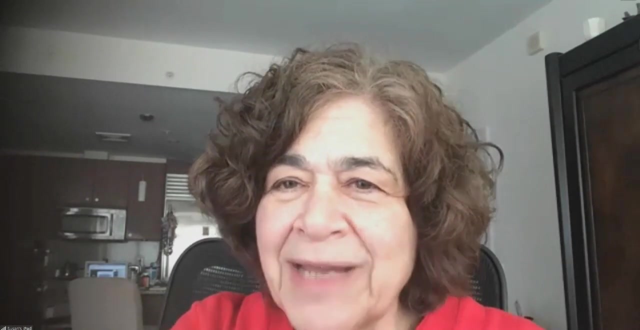 one of the options is to talk to the negotiators and on the on the industry side, it's AdvoMed and MDMA who can bring things to the table, So it might be worthwhile. You know, I don't think we know what's on that agenda yet. 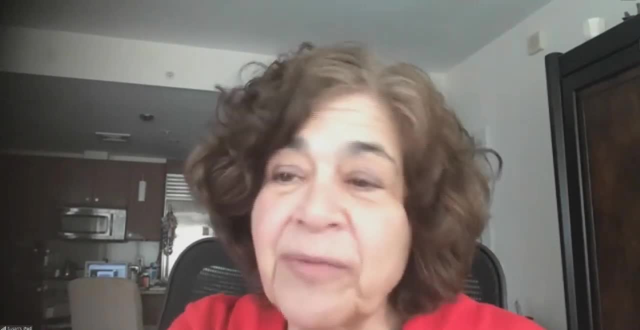 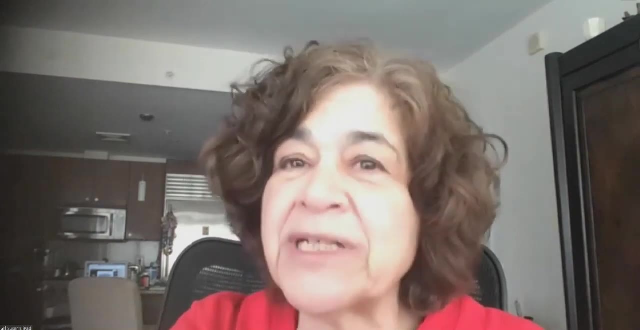 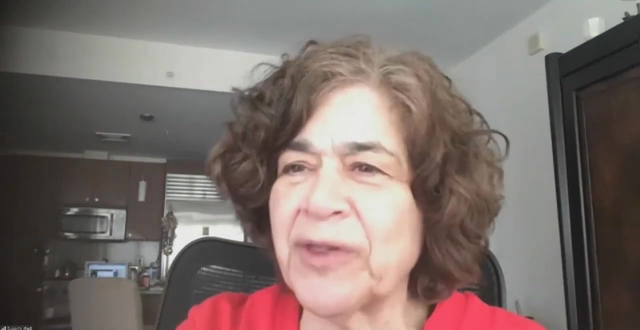 because that agenda is still being developed. Right, But from the industry. you could talk to the people who represent the industry in the negotiation and see if there's room or appetite to do that. But that's how – just for everybody else who isn't as familiar with the process: it's every five years we renegotiate user fees. 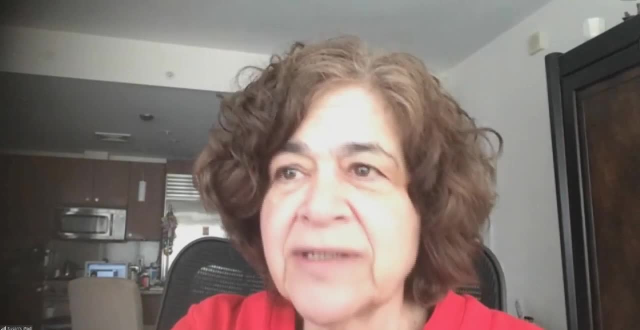 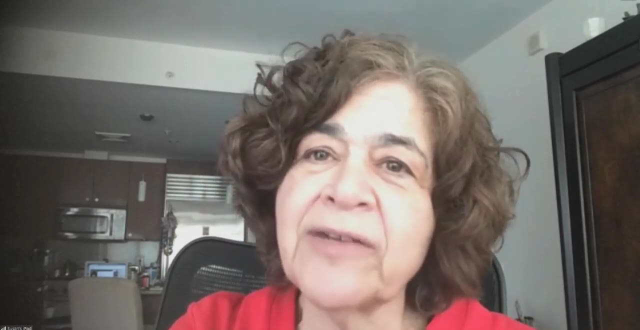 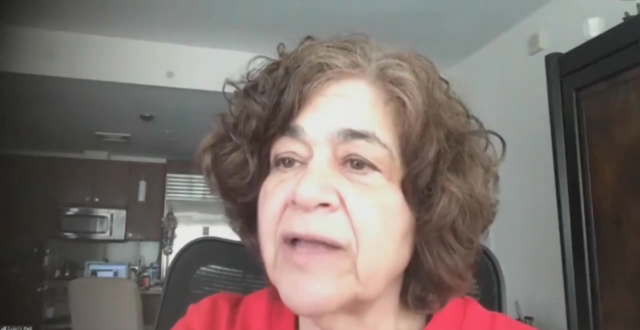 And at the time of the renegotiation of user fees, something I've done three times in my career, is to identify issues that either the industry or FDA wants to change in the law. It's an opportunity, because the law is open And so there's an opportunity to make changes to the device regulation – the device actual statute. Absolutely At the time that user fees are negotiated. So there are many times when something new will be added or something will be modified in that cycle And we are at the very beginning of the next cycle for user fee. Those negotiations are just beginning. 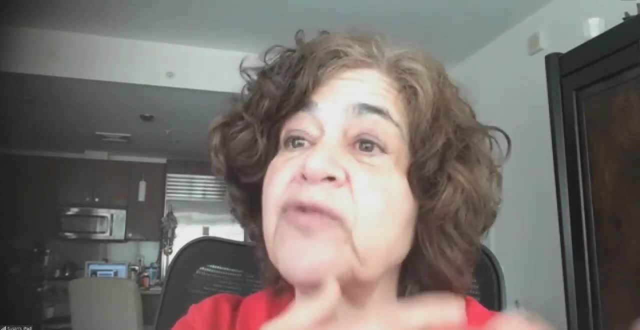 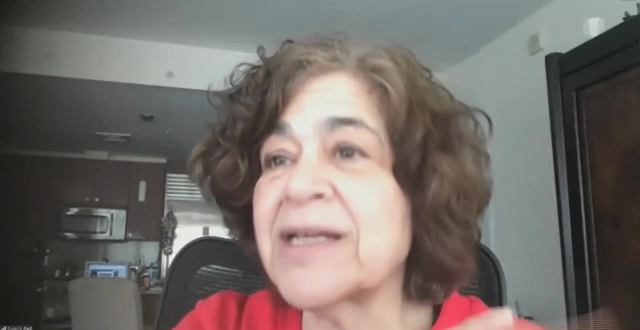 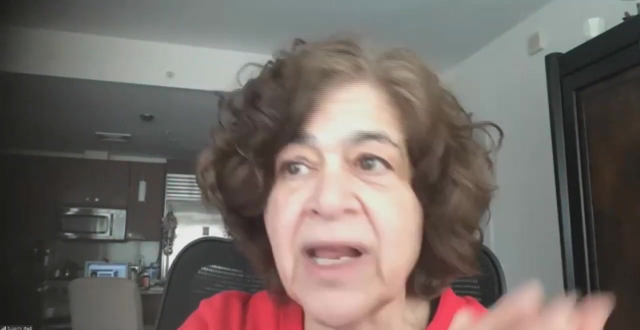 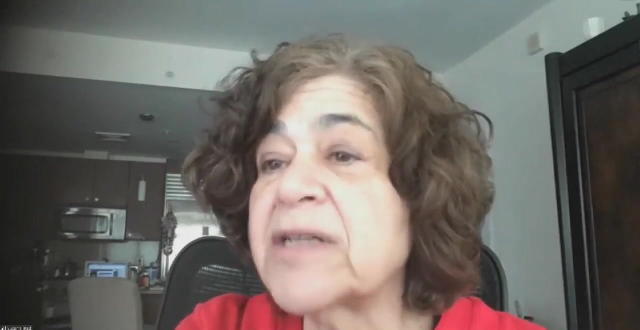 And so to Neil's point, this is an opportune time to raise some of the things that industry might want changed in current law or new law, Because this is the time to do it, When the –, When the statute is open and when the discussions are taking place between the industry and the agency, and then that agreement will be presented to Congress for their consideration, alongside the fee changes. 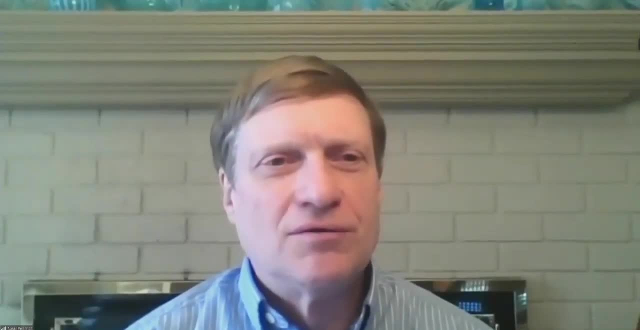 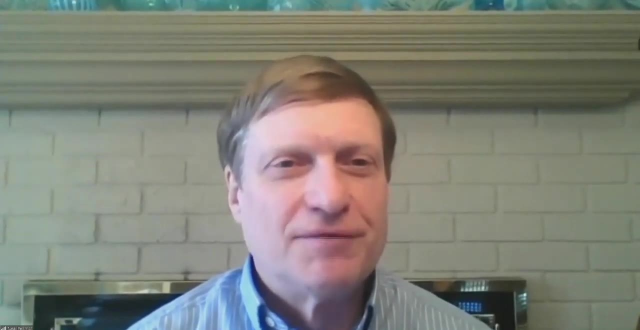 It seems like to me that we've – I've heard numbers – I have been in numbers of these discussions about HTE and it seems like everybody would like it changed. The IRBs aren't happy, The FDA has not. The FDA has not been happy. 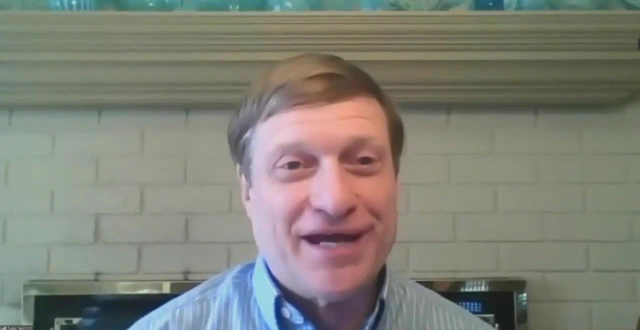 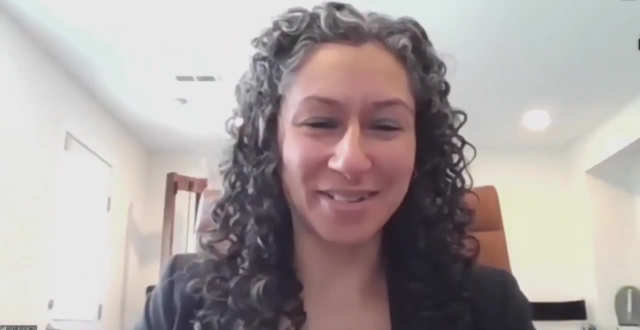 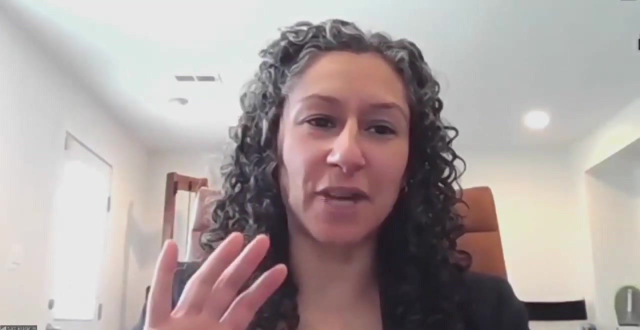 Industry is not happy. I don't know of anybody who's happy. actually, Dr Ebring, I know that was a question or not, Neil, but maybe I'll just make a comment in response. So I will say – and I'm speaking, of course, from the cardiovascular side. 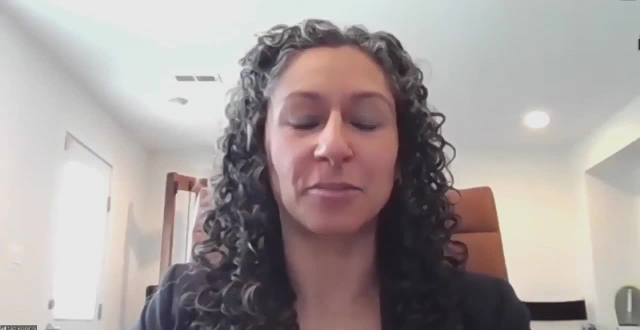 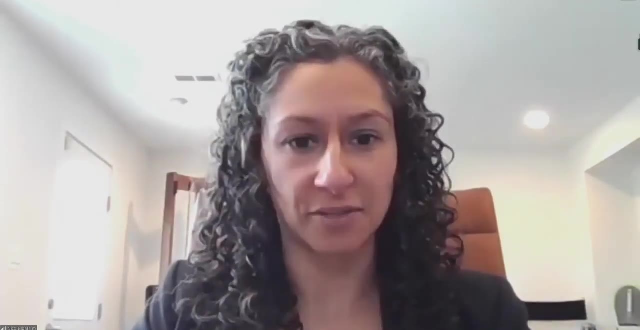 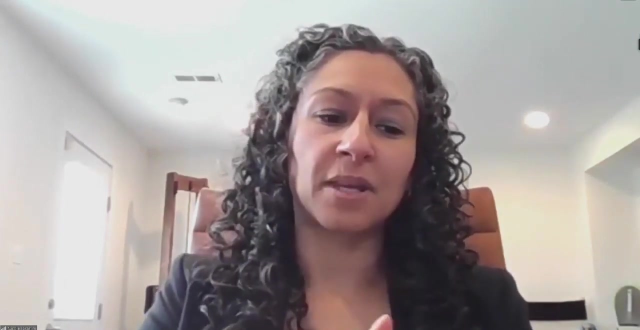 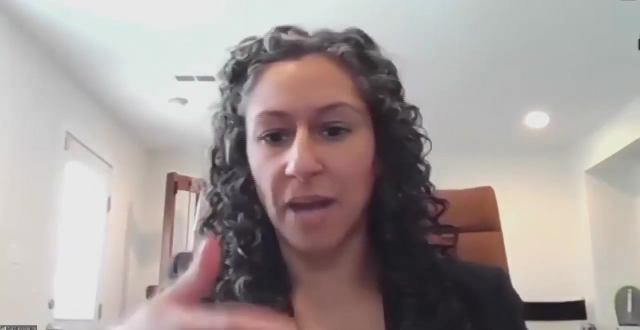 And Dr Devlin, please feel free to give a different perspective from orthopedics, But I will say in cardiovascular we have taken a different approach or a different – a different perspective to the HTE program in recent years And we viewed it as more of a milestone or a stepping stone to a longer regulatory pathway. 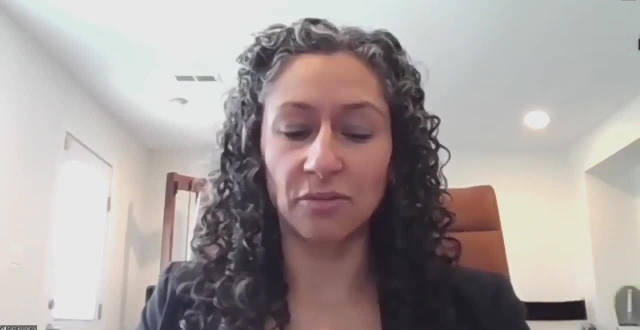 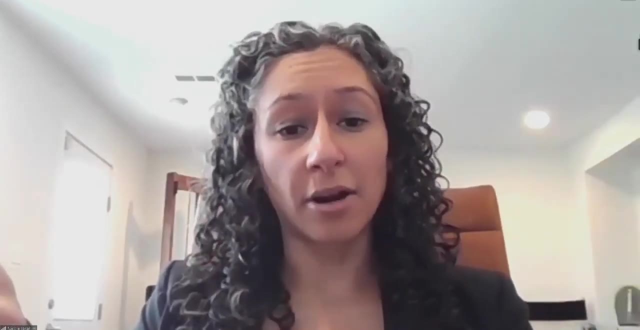 So, in other words, there have been a few devices. So, for example, two of them that I can think of – there are three in the cardiovascular that I can think of. Two of them are pediatric devices, So the Berlin Heart X-Core device and the –. 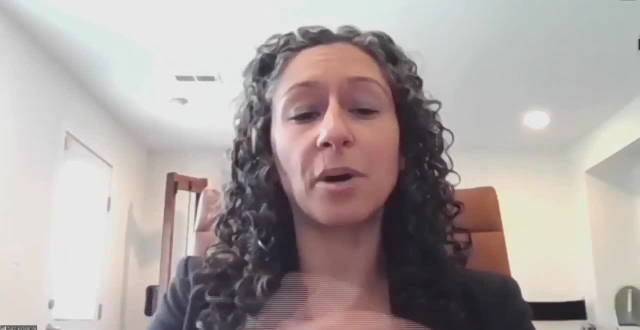 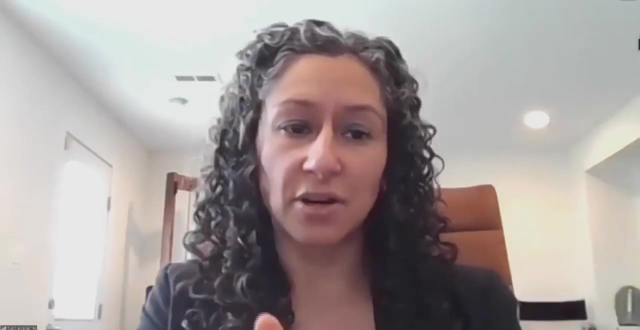 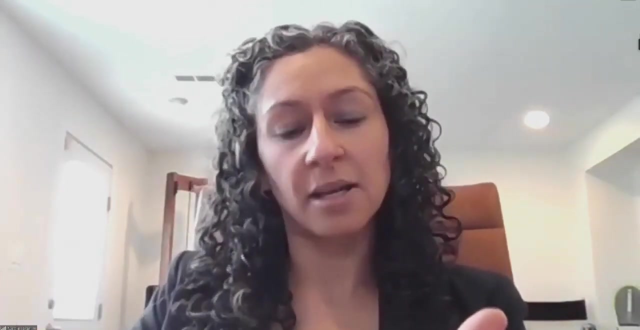 Yes, Melody valves- the Medtronic Melody valves have both gone through this, where they started out with a small study that supported safety and probable benefit, received their HTE approval, but then we worked with them to design the post-approval study market requirements. 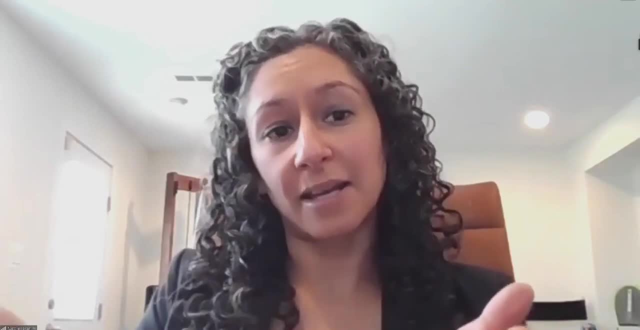 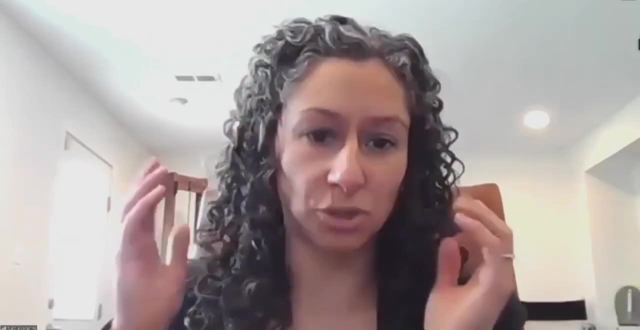 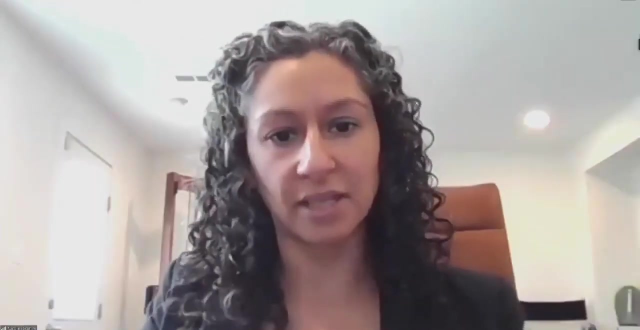 and data collection to be able to gather the right data that they would then need to support safety and effectiveness for a PMA, And so it was more of a progression as opposed to an endpoint, And I think that it makes a little bit more sense when you think about it in that sort of holistic view. 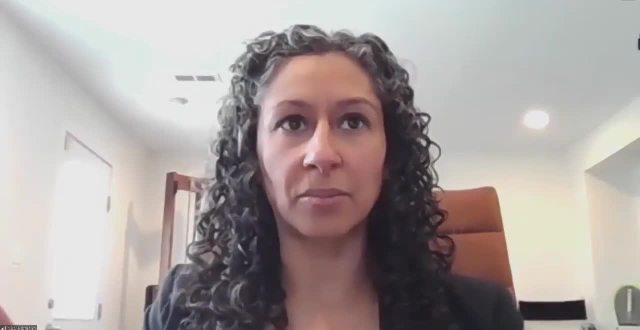 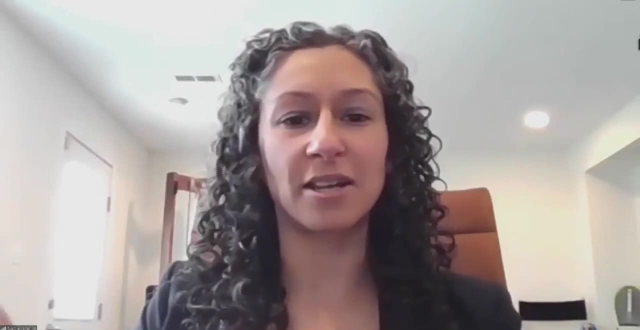 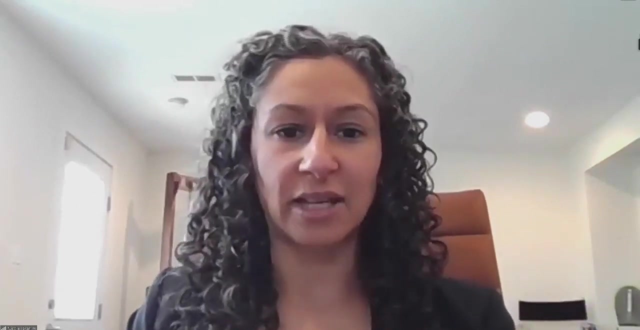 And it also makes the path to market a little bit less scary, maybe, in that you have these milestones that you can achieve on the road to establishing safety and effectiveness. So I hope that there are more devices that don't necessarily get stuck in HTE RAMs. 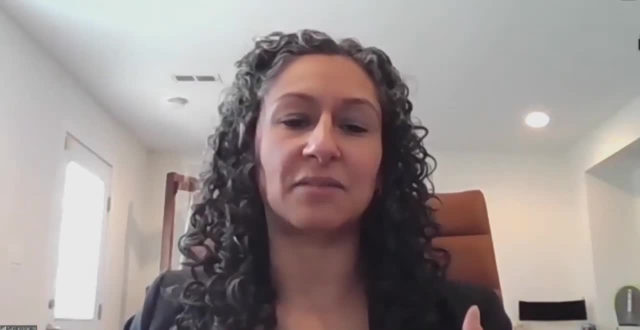 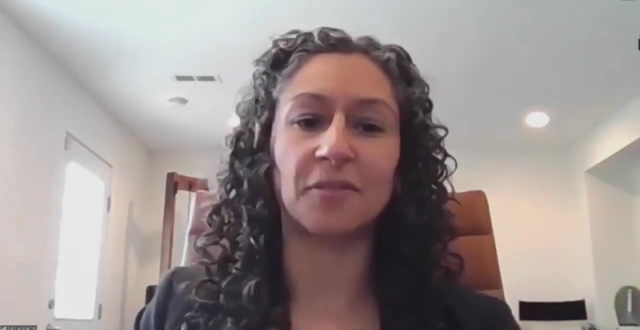 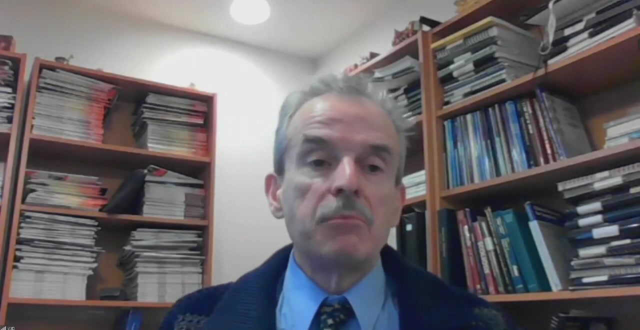 but that we can really gather the data for, so that we have the effectiveness data and the clinical community can, you know, really make use of an effective device. I would agree with Dr Ibrahim Precisely in the example that I presented on the HTE for the spinal tethering for fusionless correction of scoliosis. 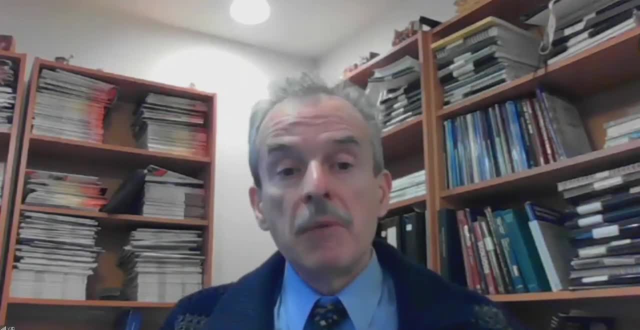 that was our rationale, because if we were going through a PMA process, that device would not be approved yet. It would still be collecting data to see what the outcome was. So our thinking was: if we can get some of the HTEs going, that's a great accomplishment. 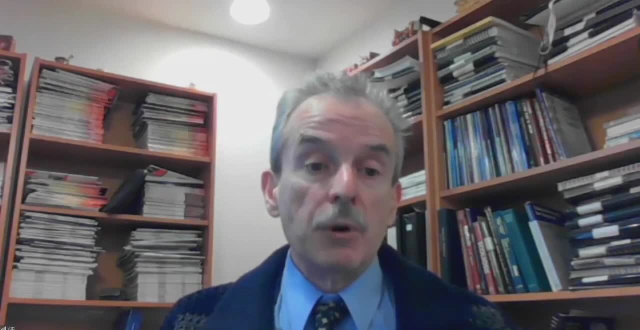 because we never would have got the data that we have. and then we're expecting, when we collect more from the registries, that we could have those devices through a de novo, Because in orthopedics the majority of our devices are class two. 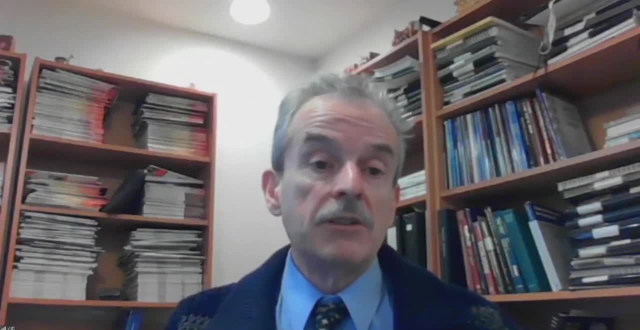 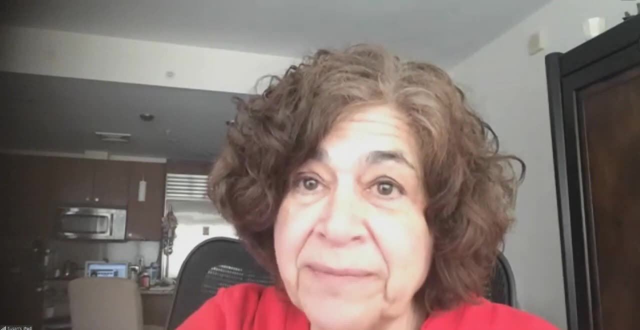 We don't have a lot of class three devices, So the HTE to de novo will work very well for us in the future, we think. And one of the issues there, Yeah, Is payment, which is not FDA's issue but it's the issue for the industry, and working with CMS. 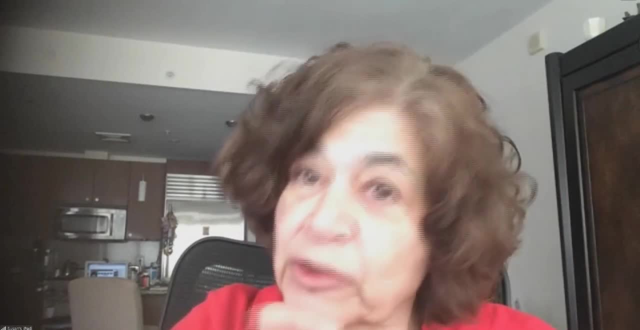 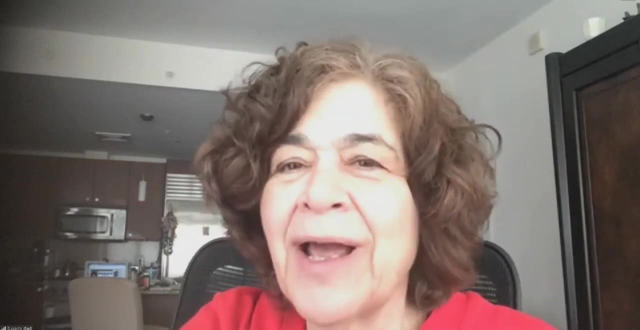 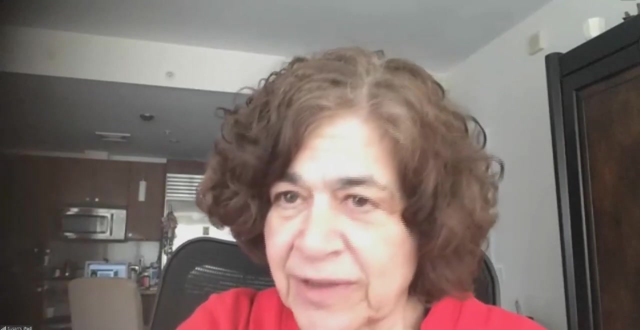 And that it's a little trickier to get reimbursement on the HTE side. You can charge for the devices, but they don't necessarily get paid what you want, Whereas if you continue to develop the data and do go to PMA, it's a very different process. 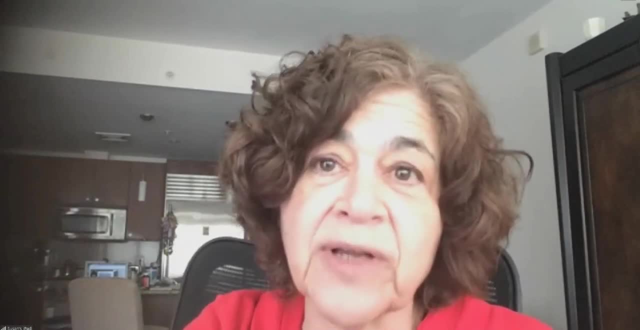 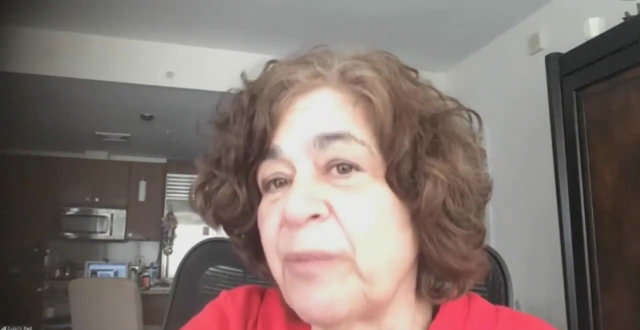 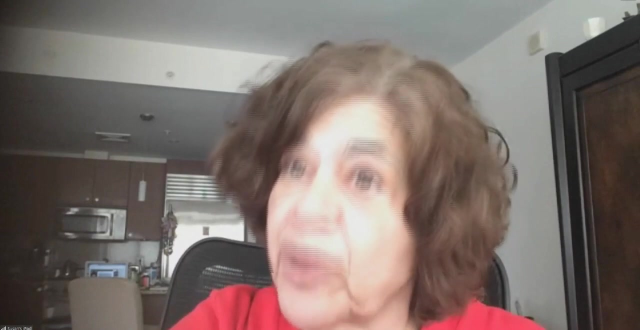 for reimbursement both from individual insurance companies as well as from the federal government. Yeah, So there are benefits again have in taking Melody through. There are very. there are wonderful benefits for being able to do that And in terms of broader access to the device for the people you developed it for. 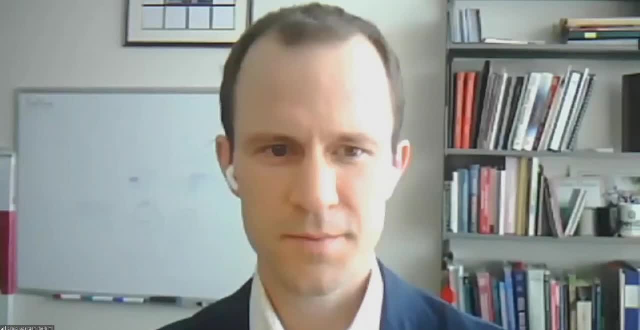 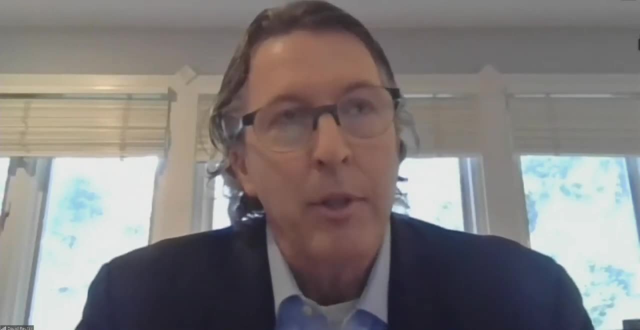 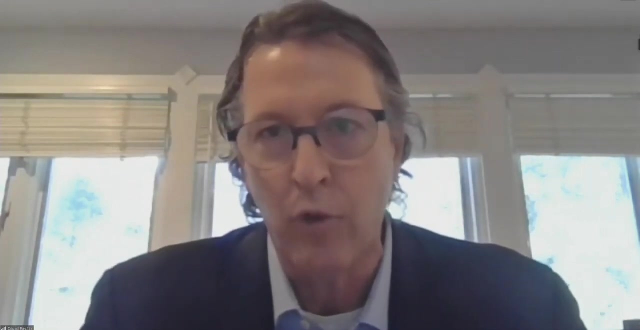 which is for the kids. Yeah, That's great, Dr Reiter. Let me shift topics, if I may, just a little bit. I'm intrigued with the purpose of the CTSI and the whole purpose of this session, which is to generate innovation and ideas for our kids. 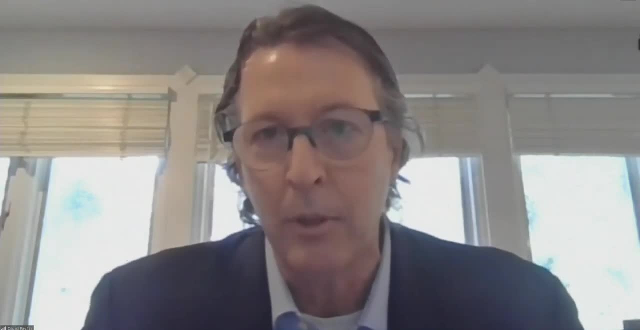 And we've talked about ecosystems and I'm aware of at least a couple of different partnerships that exist And I'm just curious how we can best leverage them. We've got this partnership between Riley Children's Hospital, Purdue and Cook, where you can take complimentary expertise and try to create some sort of synergy. number one: 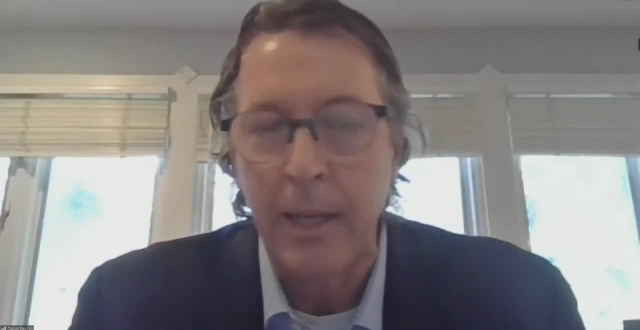 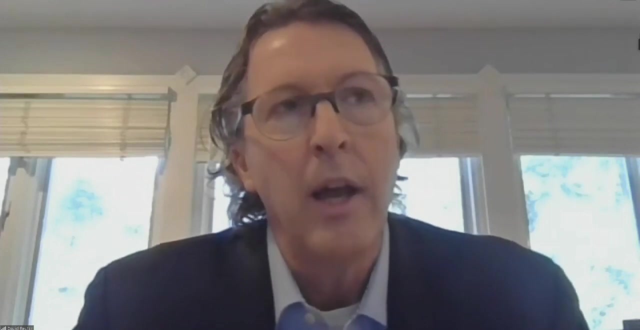 And number. two years ago, Wade Clapp started the, the MD-PhD program within Indiana, and now IU School of Medicine, in collaboration with Purdue, has an extremely robust MD-PhD program. So my question to the group is: do we have an opportunity to use that resource? 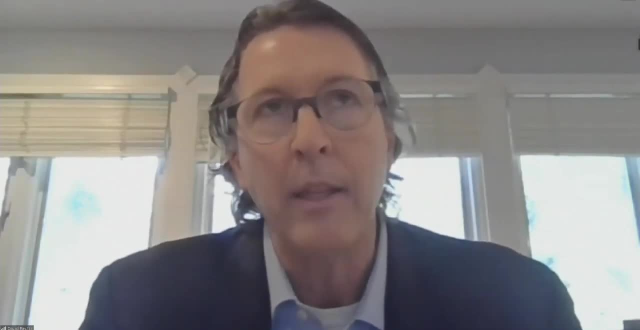 Some sort of an MD-PhD student who in the first part of their training they just kind of they find that problem, they study the problem, they do that intellectual heavy lifting that I talked about And then they have the opportunity to do that. 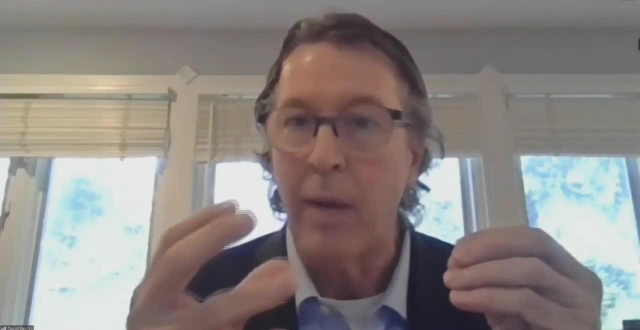 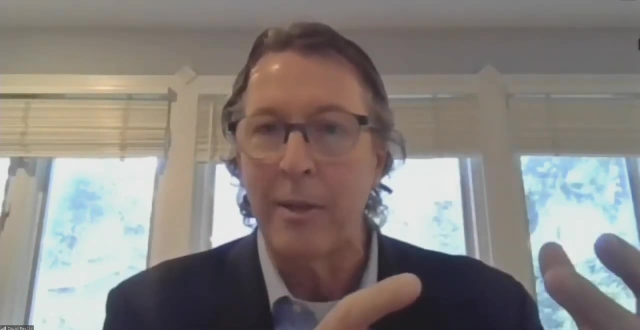 So I think that's the key And I think that's what we're going to be focusing on early on. And again, you leverage the fact that you've got the insights of Riley's clinical data with the technical expertise of Purdue, and let that be the formative stage, the IP stage. 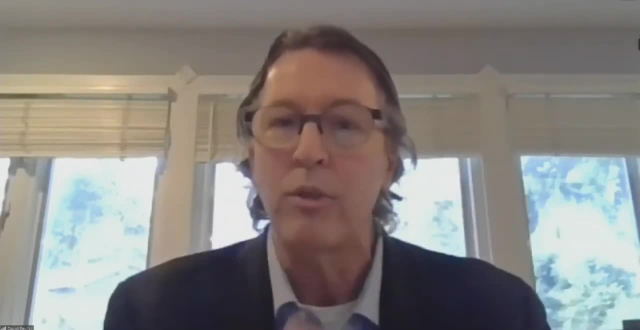 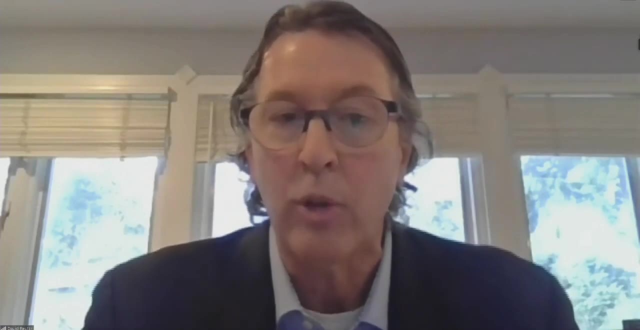 et cetera. you take advantage of Cook's proximity and say we can now mature this and kind of get you through some regulatory steps. And then maybe that MD-PhD student- by the time they're in clinical studies, they've generated some sort of clinical trial and they're the ones that are trying to push. 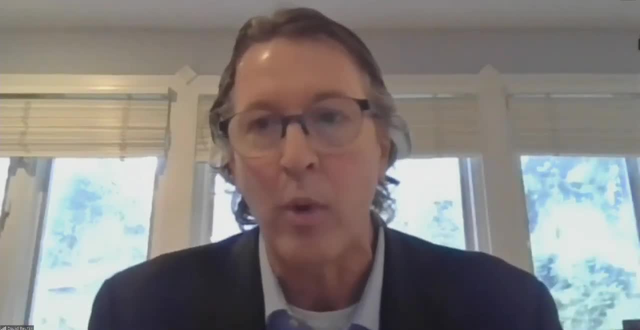 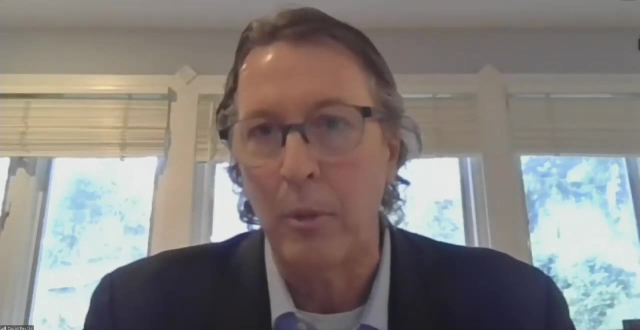 forward And maybe it's simpler. It doesn't have to be a cardiac implant, It can be a wearable device, But it seems like generating momentum is going to be valuable, And if we want Indiana to be a go-to place, you don't just get there, you have to build. 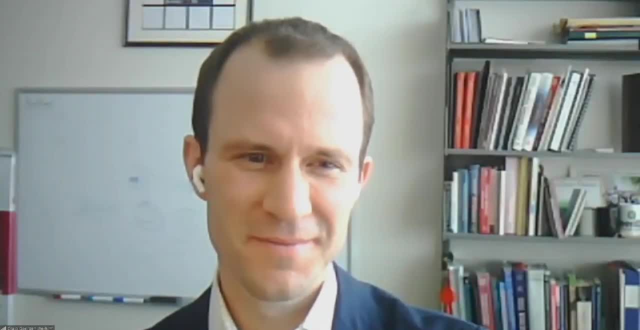 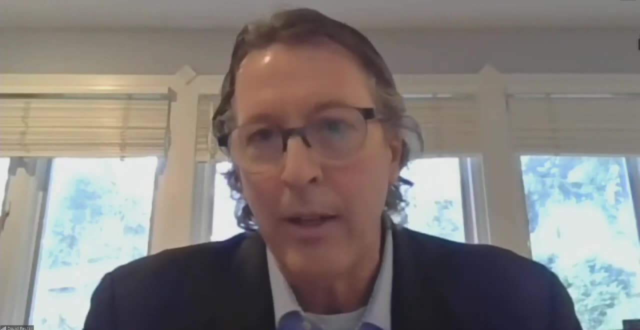 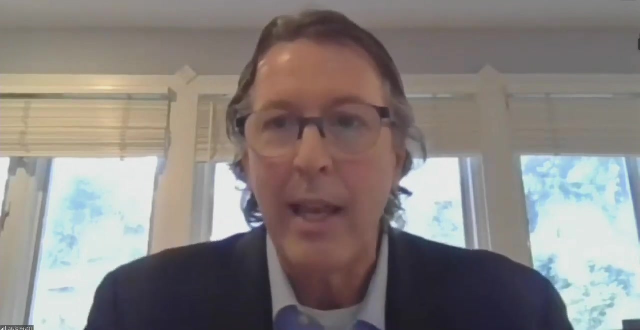 your way there. Ramp up too, Yeah Yeah. So I guess for the FDA that might have insights on a number of different states. are there any other examples out there of collaborations and institutions? Are there any other institutions that have taken that MD-PhD brain trust and been able? 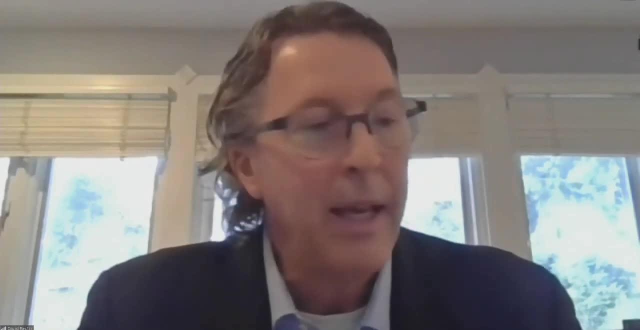 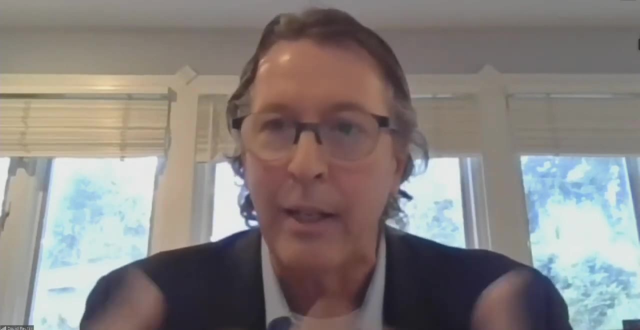 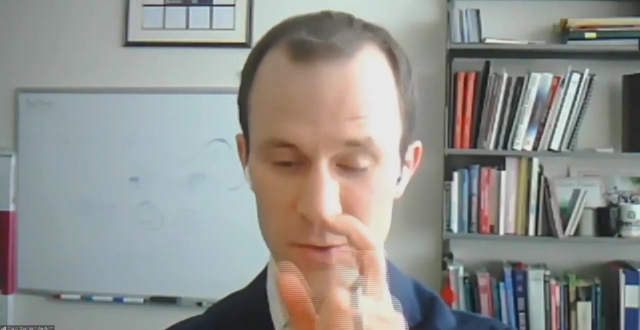 to generate some sort of innovative momentum, And can the CTSI effort take advantage of anything that others are doing and kind of get the momentum started here? Yeah Well, I'll throw it to you, Susan, in just a second. But right at Walden School, engineering at Purdue is closely connected to both Cook and 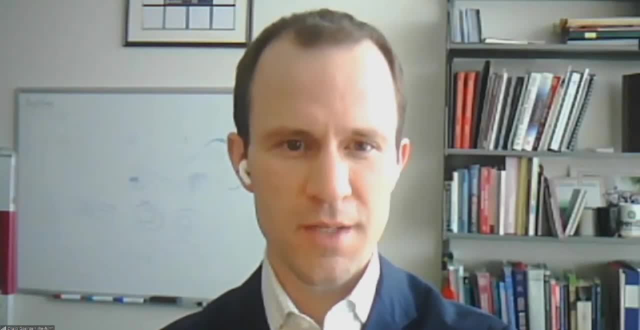 Riley. It's a true formalized consortium that's going to take advantage of and build the momentum and expertise of each of those institutions. So one of the MD-PhD students in my group is Connor Earl Connor, if you wanted to join, maybe you could tell us a little bit about your recent efforts. 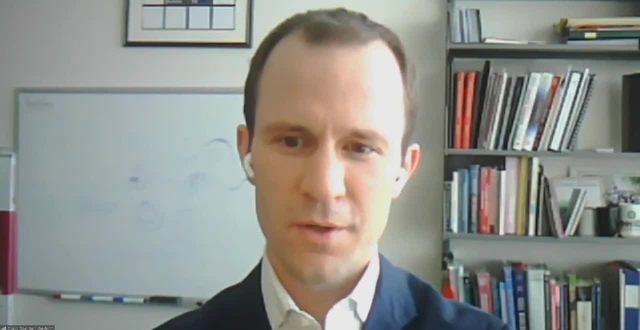 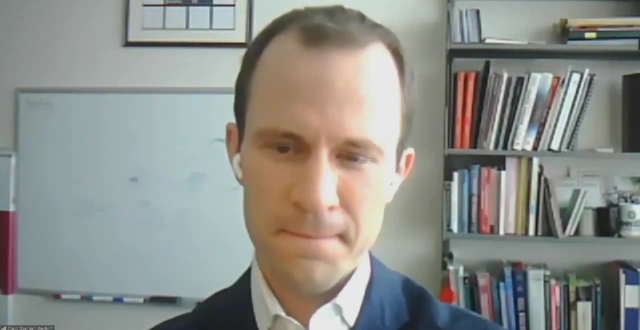 to identify unmet clinical needs at Riley and connect with Cook Medical and Cook Research in their efforts to develop medical devices for pediatrics. Sure, Sure, I'd love to. I'm having a hard time starting my video. I'm going to go ahead and start. 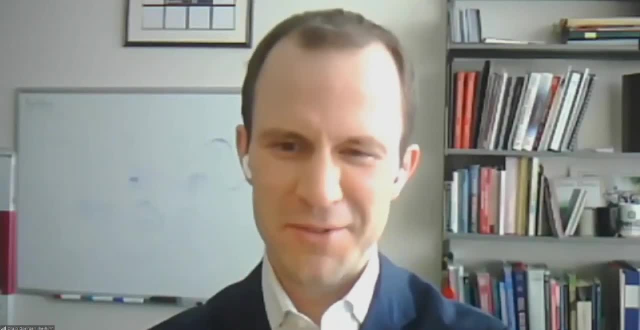 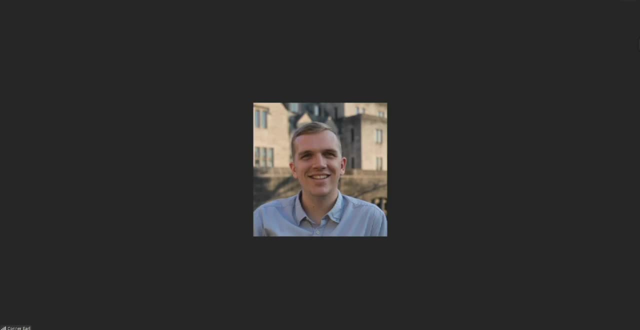 Yeah, Starting my video, I think We see your picture. That's fine, Okay, Perfect, That's what I look like. But yeah, Dr Royer, that's a great question, And so, yeah, one of the things that I've been working on is that, as part of this collaboration, 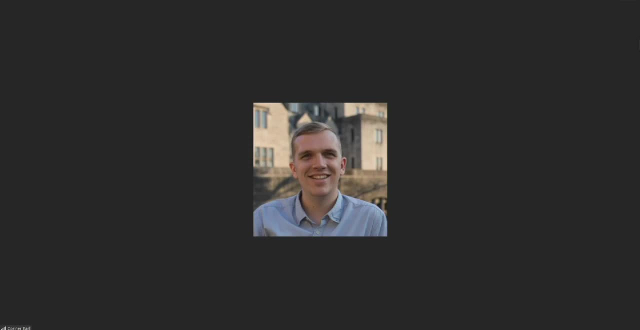 between Purdue and IU and Cook and, to give you a quick background, I'm an MD-PhD student. I'm a PhD student. I'm a first-year PhD student in the lab with Craig And I'm hoping to do exactly what you're talking about. 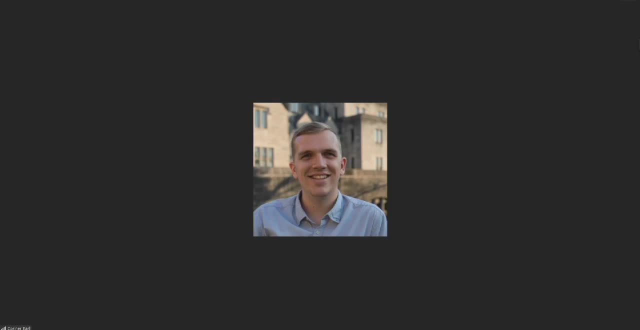 And I've been working as a liaison for this consortium initiative, trying to identify clinical needs for others as well as myself that I can leverage in my PhD and beyond, And so it's been a wonderful experience, And I think there's a lot of work to be done. 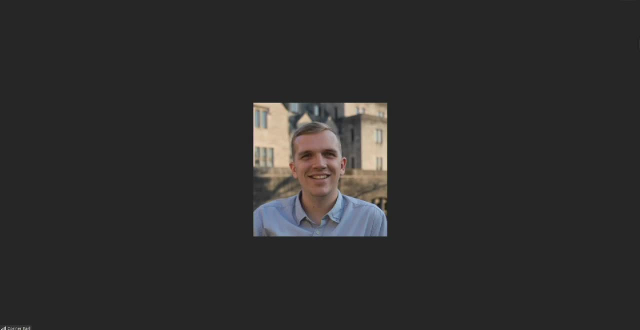 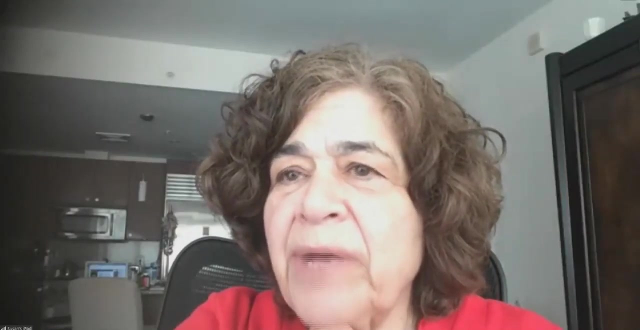 Thank you, Thank you, And I think there's a lot of potential to grow that, And I see that happening at Purdue with Riley and, of course, with Cook. Great Thanks, Connor, Dr Alpert- I'd let FDA talk about the pediatric consortia. 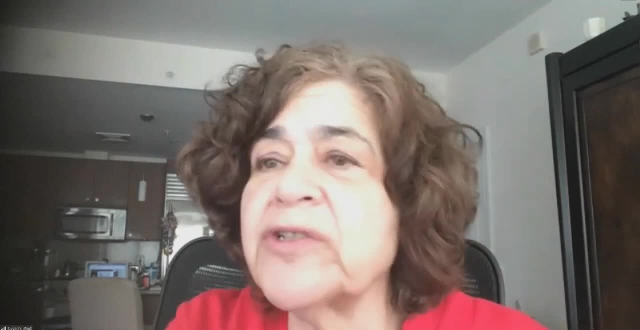 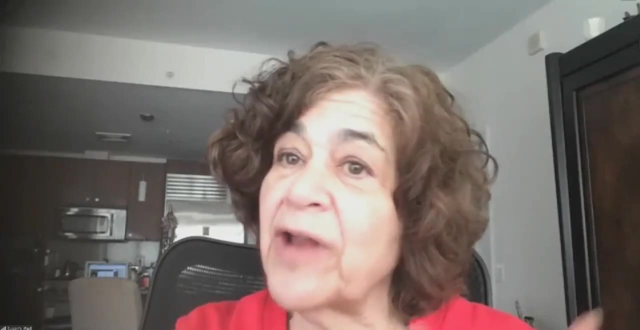 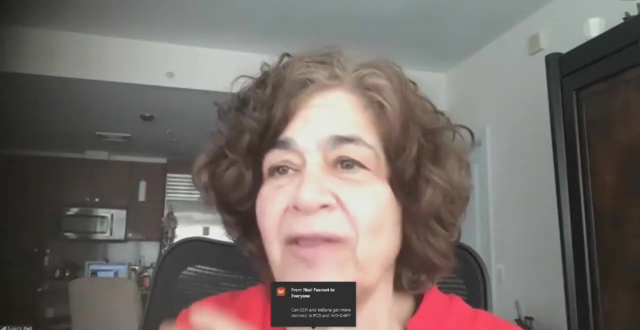 But if you want an example for something that's not one of the formal consortia, talk to the folks at the University of Minnesota. They've been working in that arena. They're not one of the formal funded consortia, But they have a pediatric consortium that's working on those kinds of issues. 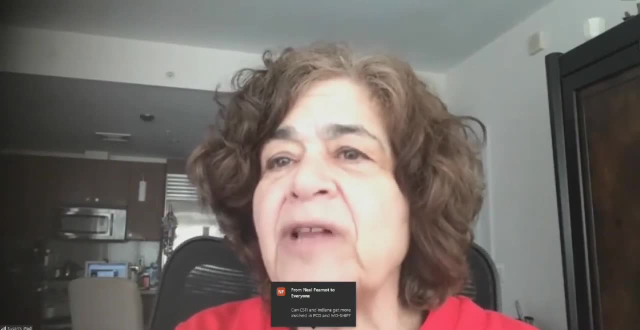 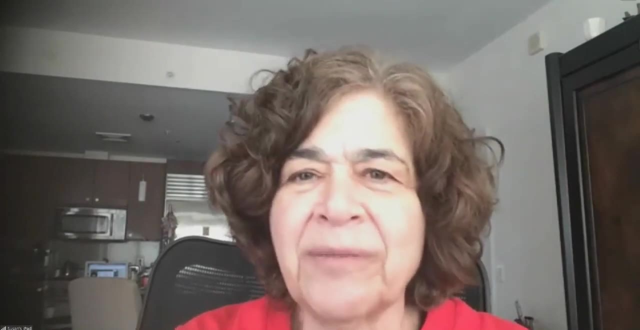 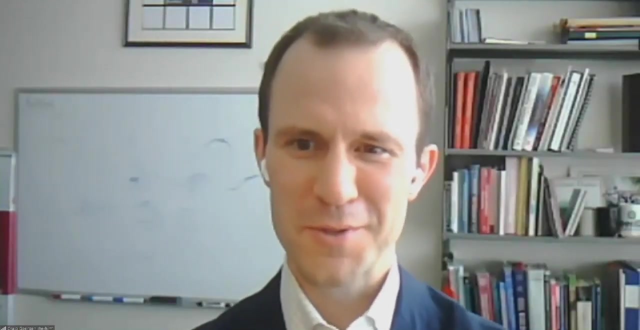 They also have a fellows program, the Erlbach, and Fellows that work with them as well. So there are some really nice examples, but I'll let FDA talk about pediatric consortia. Dr Ibrahim, do you want to mention anything about pediatric consortia at the FDA? 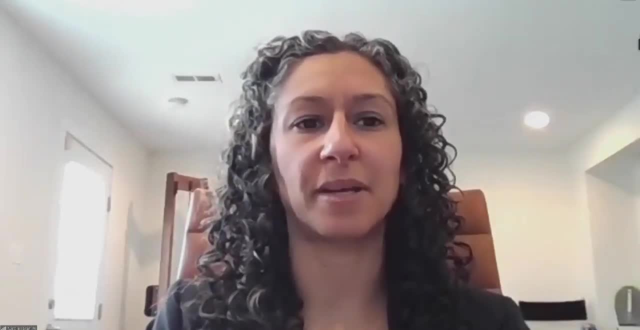 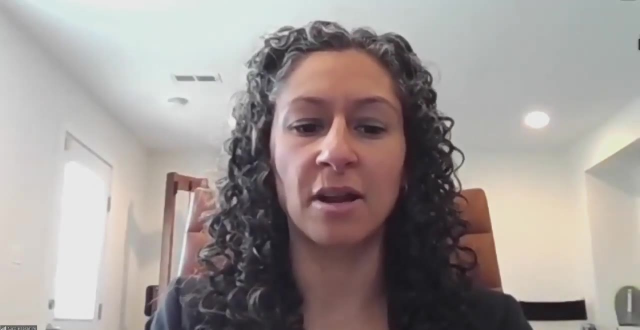 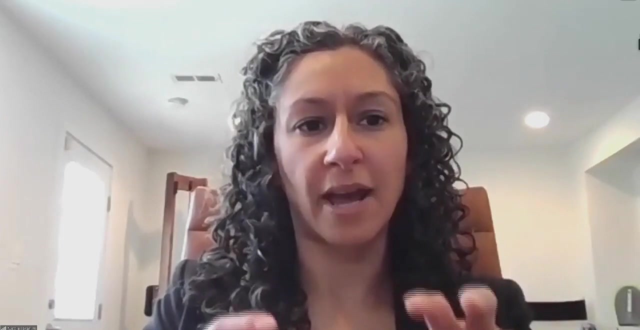 Sure, I can start. So the Pediatric Device Consortium: It's a consortium, It's a consortium. The Pediatric Device Consortia are. there are five different consortia around the United States that are basically hubs to try to And they're sort of headquartered at medical centers of excellence in pediatrics. 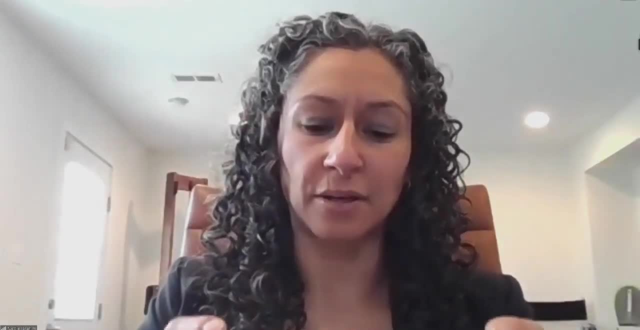 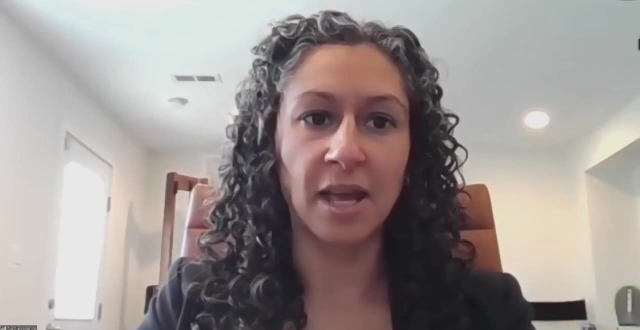 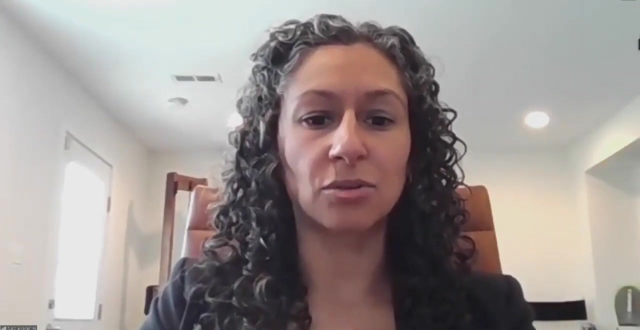 And the intention is that they form a group that can help, support and assist with entities that are developing pediatric medical devices, And the consortium does that. It's a consortium where we have a few pharmaceutical companies. consortia are funded through the FDA, so we receive a grant every five years and the consortia apply. 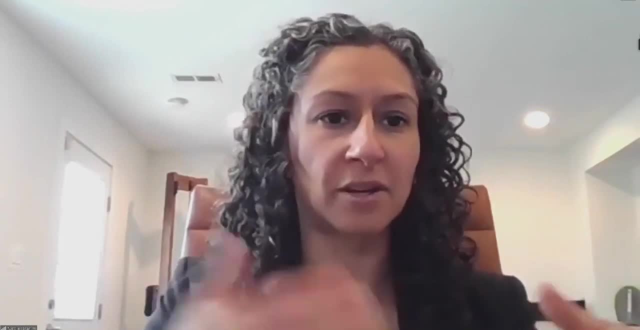 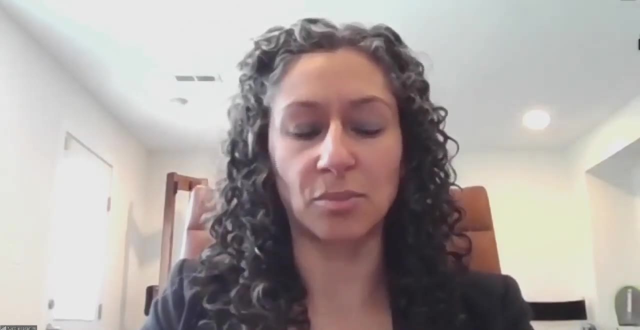 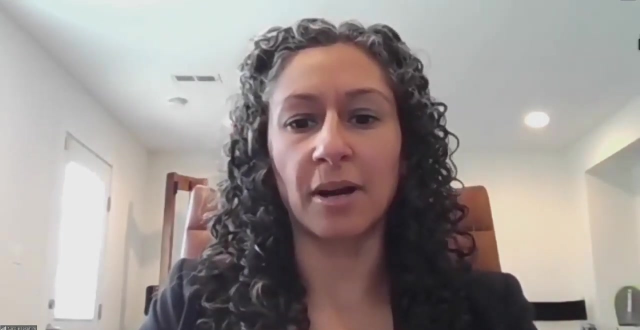 for the grant and, like I said there's- there's five of them and their funding gets renewed every so often- but but they offer regulatory services, they offer support for how to deal with raising funding, they offer support for a pre-clinical testing paradigm, so that there's a whole breadth of 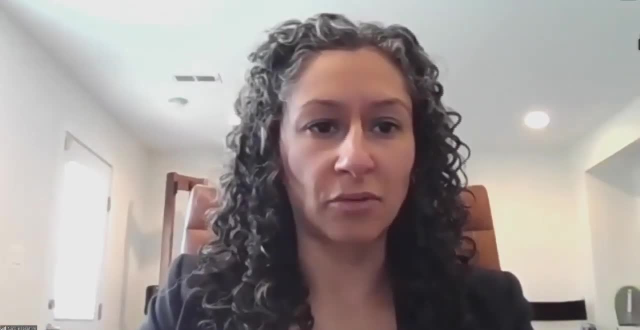 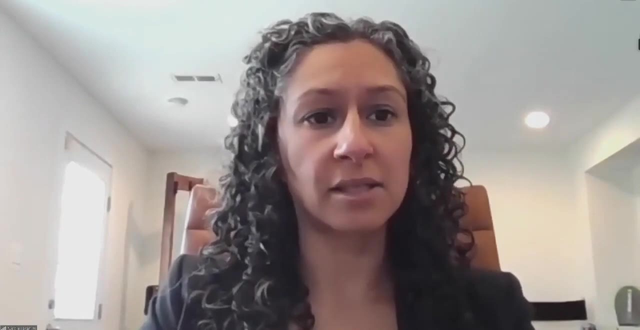 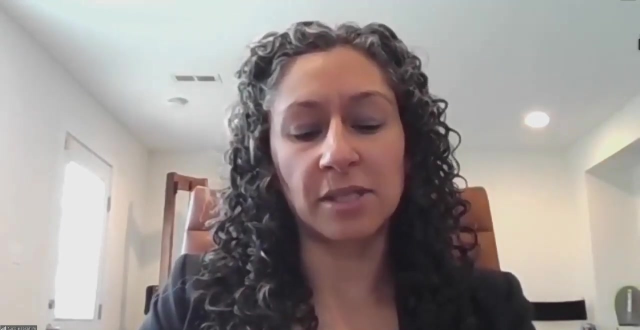 information and resources and support that they can provide for developers that are looking to bring a pediatric device to market, and so they award grants. so you can apply for a grant if you're developing a device from any of these consortia, and I would say that the majority 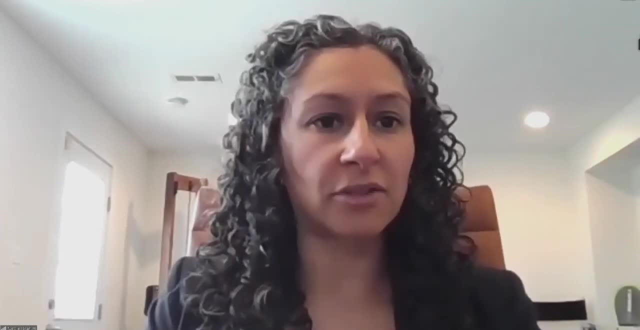 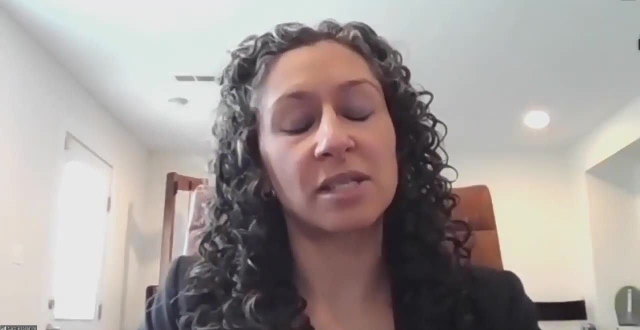 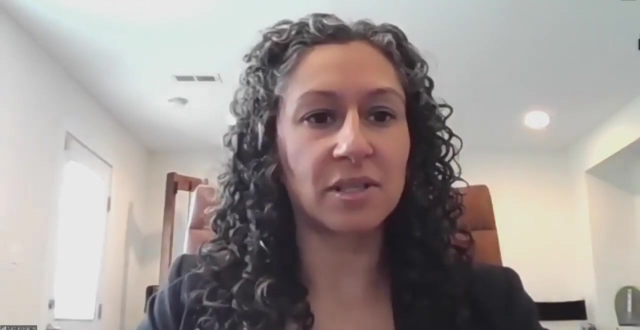 of what we've seen from the consortia are probably class two medical devices, although there are, you know, a handful of class threes there. I would. I actually saw a presentation recently on a couple of the consortia and I would say about 10 percent of the devices that come through the consortia make it to market, which 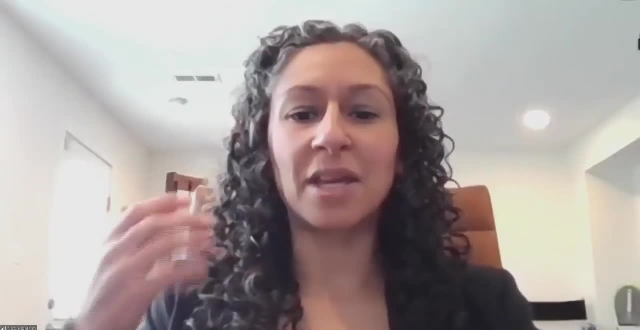 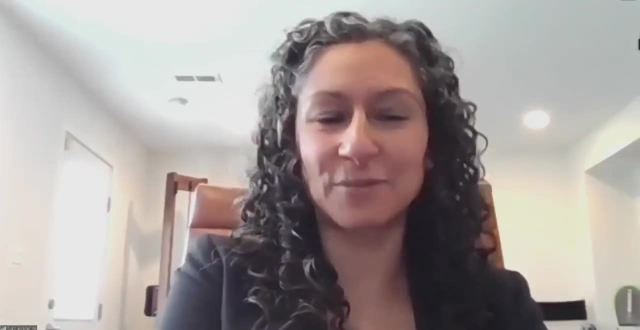 sounds like a small number but I think when you consider in general the yield of device development and you know devices that start out in the, in the ideation phase, the number of devices that actually make it to market are quite small, and so 10 percent is actually. 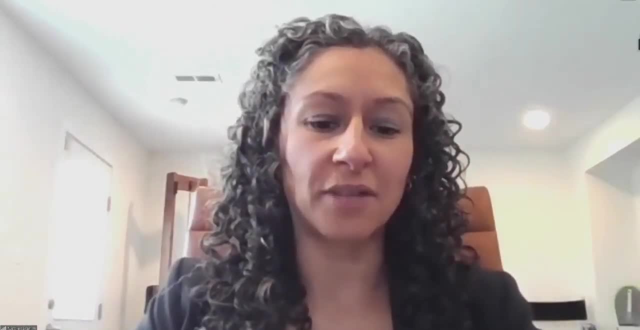 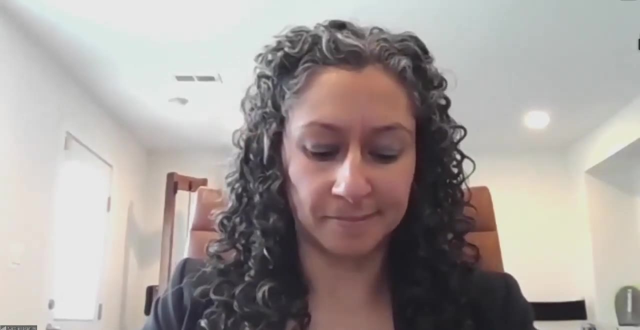 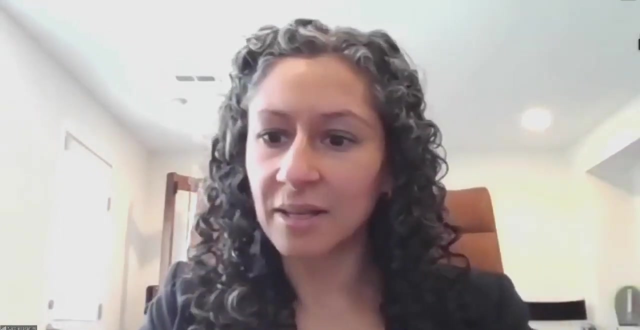 not that bad and so so. yeah, so they. they're a funding source for a number of different device developers for pediatrics around the country. awesome, Dr Fearnaut was asking a little bit about the ship md nascent effort as well. right, were you on some of the calls a few weeks ago, Dr Fearnaut? yeah, I just wondered is. 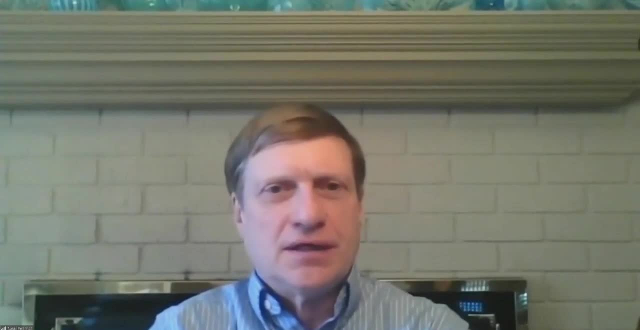 way that CSTI in this group could become more involved in that program, since Riley is it's a huge hospital for children and has a tremendous database behind it, with Regenstrief and and the other relationships, part of a big medical school. so I just wondered: why aren't we more involved? 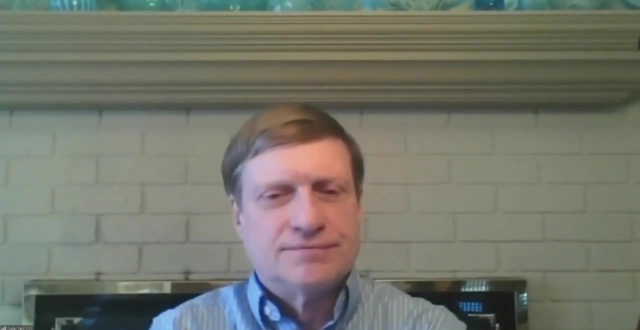 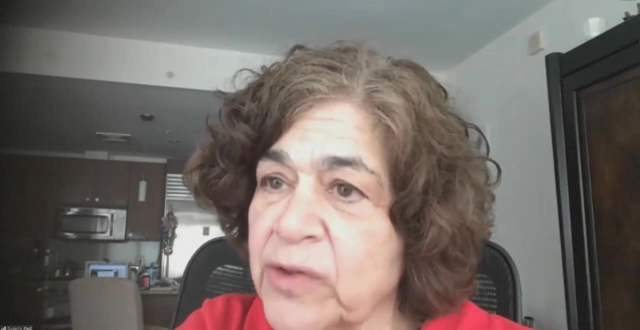 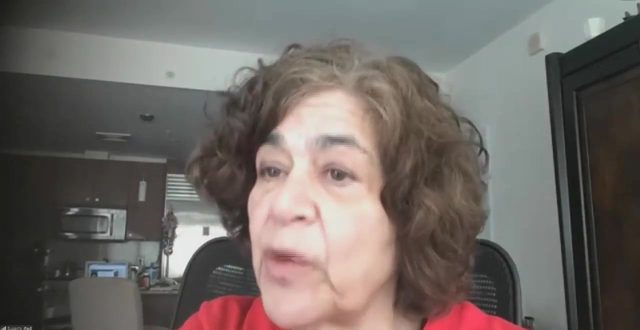 and can we get more involved and what would those steps be? thank you, yeah, I would just suggest that you talk to you. talk to the, the folks running the pediatric consortia at FDA, but also talk to some of the consortia that are not in the funded group to see how they're working. so, as I said, UMN is. 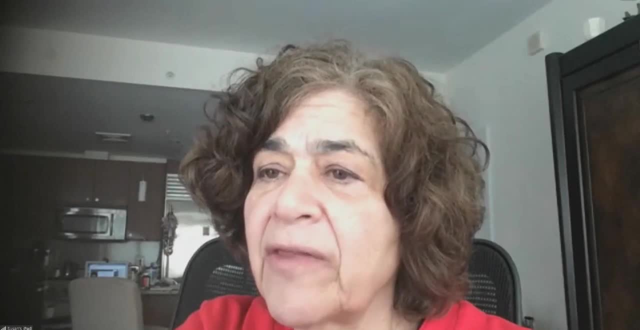 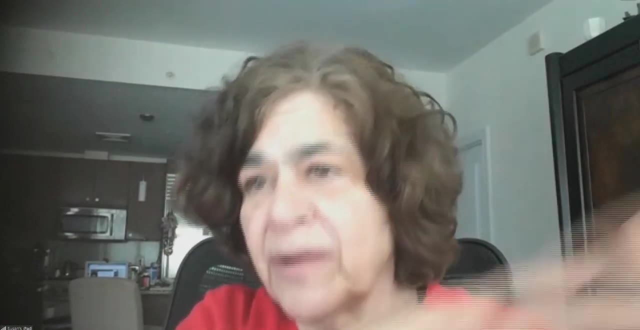 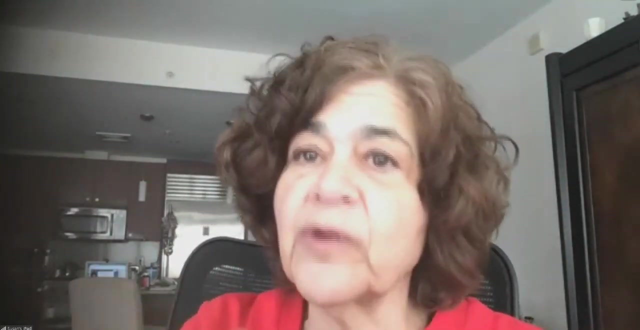 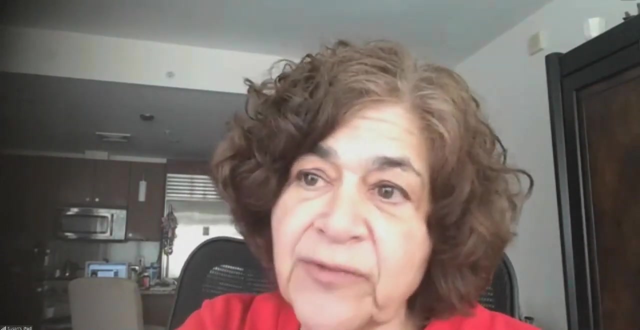 one there, there are several. there are four or five around the country that are not part of the, that funded consortia that are that are funneling government funding to, to end of, to pediatric innovation. but there are other, there are other groups that are working in that same, in that same sort of environment, creating opportunities. 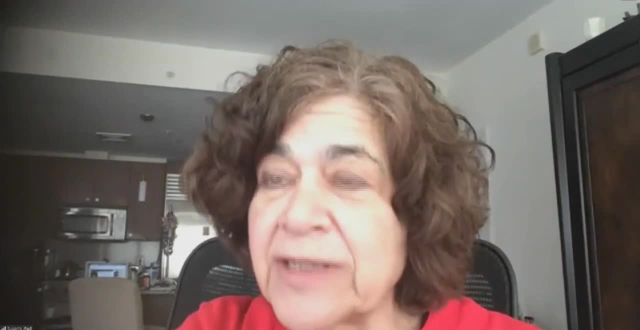 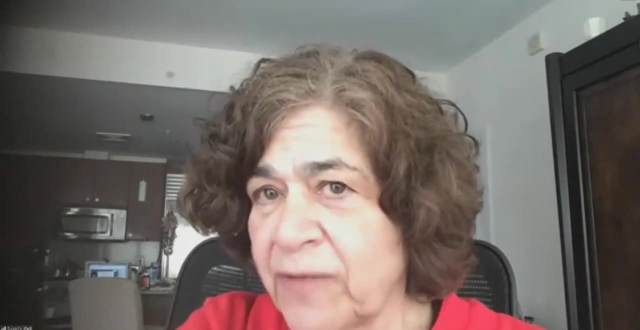 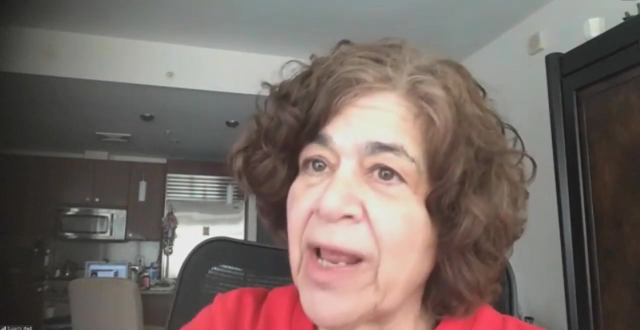 for innovators, particularly from inside universities, to move, and I think the other, the other group that you might look at are some of the tech transfer offices from the universities who also are are working in in that arena to try to get better at taking academic ideas and turning them into viable product by 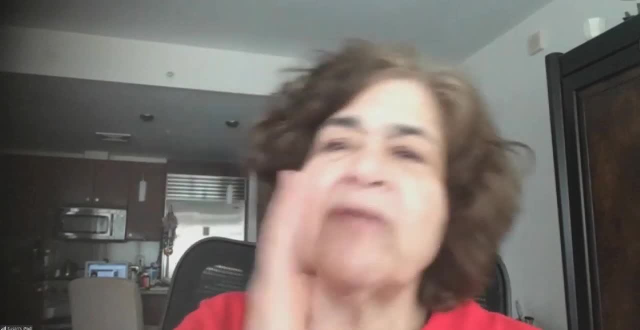 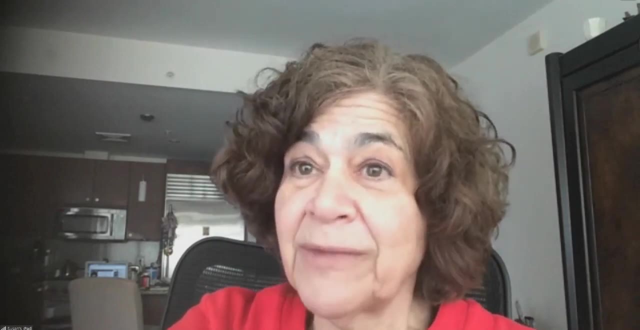 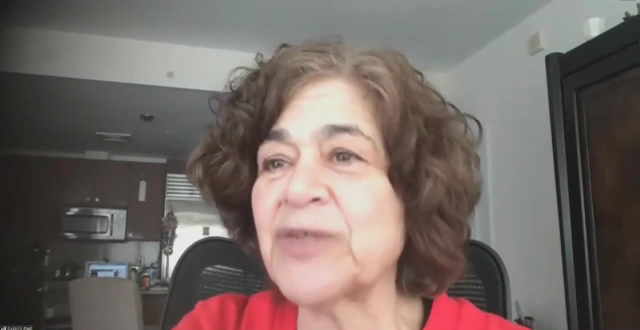 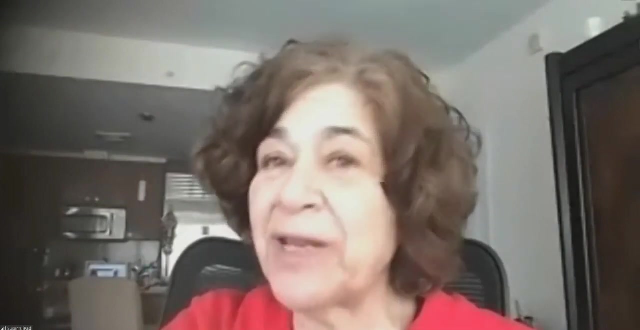 paying more attention. universities about about five years ago or so- maybe it's 10 now- realized that they could actually get some finances by investing a bit in their, in the innovation that's taking place within the university and helping those innovators, those professors and graduate students, to make their products enter the market. 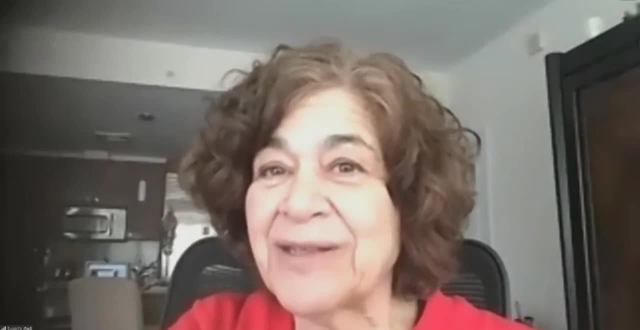 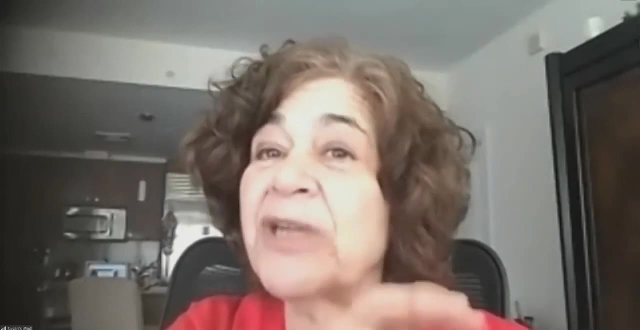 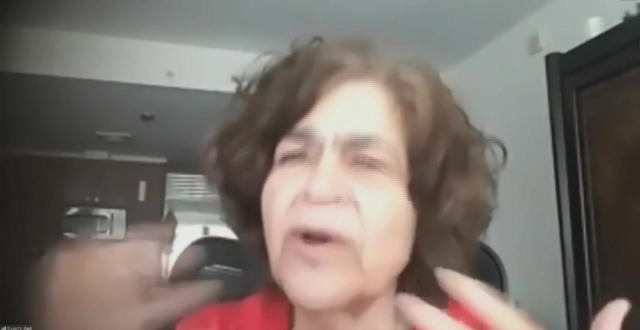 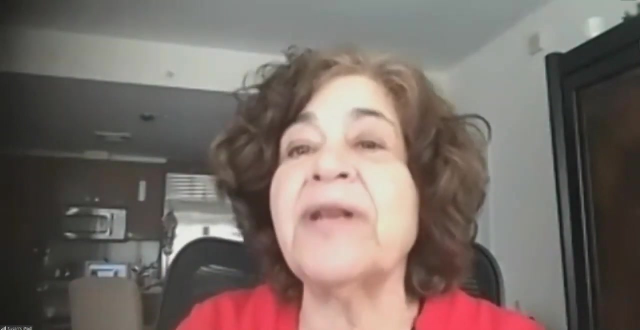 because the university owns some of the IP and many of the of the of the tech transfer offices have have now become much more facilitators to help academics who are not innovate, who don't understand the the business of innovation. they innovate, don't understand the business and the regulatory environment, but create it. create pathways for them to get into much, much more of. 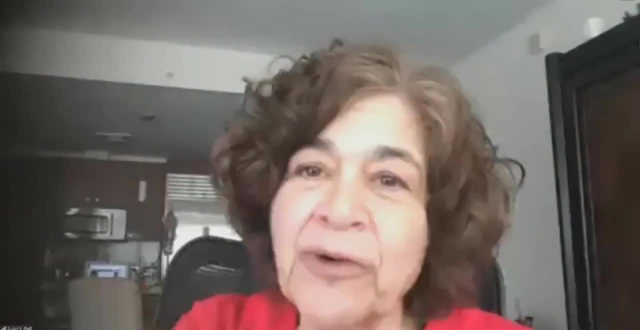 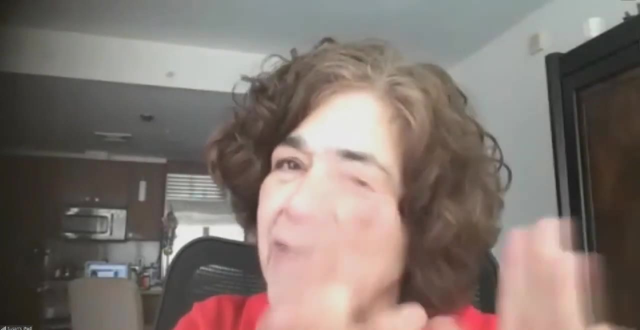 the of the actual commercial marketing. so there are a number of things and I'd be happy to talk about some of them because I know a few of them, but I think that they're that you have to look at those as well. so talk to your tech transfer folks at the universities and see how interested they are. 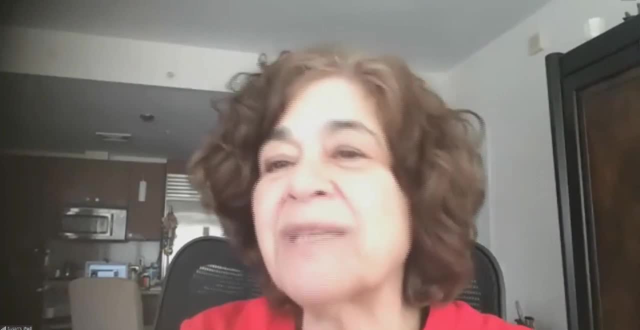 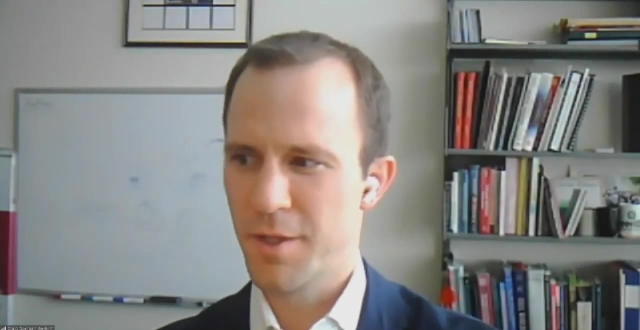 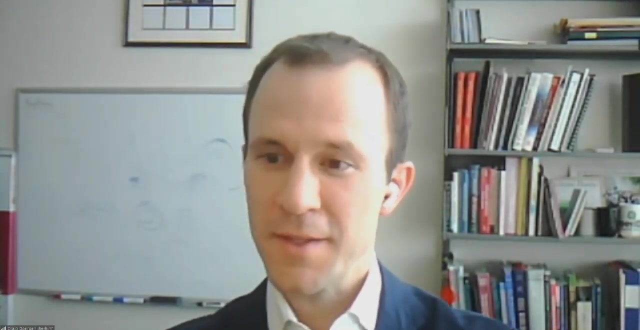 because they might be a really good place to make some of this happen. yeah, um, good question. you know I, I certainly know you you're kind of a small group, uh, and if I know, if I know you think I a small group uh, alright, well, that that would be interesting. I just I wouldn't really washing things. 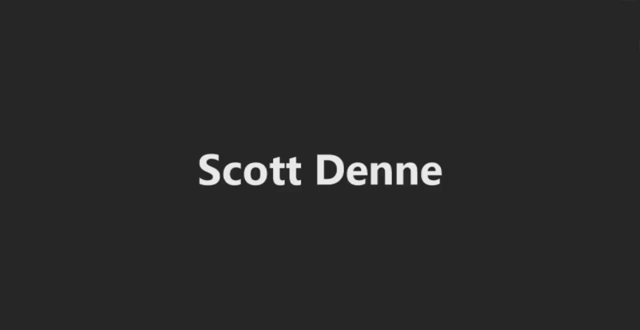 automatically, or being one of the leaders of the department that I know. so no, we don't. I, no, let's see, I don't think. I think it's just�무�ně unit. well, people are, we know we PhD work there. it's sexual rights. i mean, you know we do race M's F schools, but i think in some 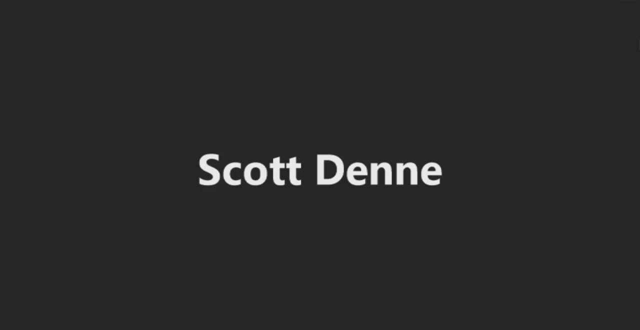 universities. there's certainly issues. there's partners. you know those businesses that are availability in children And I know devices have kind of gone down a different path. I know about the pediatric consortium. I guess from my perspective as part of the pediatric community I would view that as modestly successful, but not nearly the success that drugs have done in. 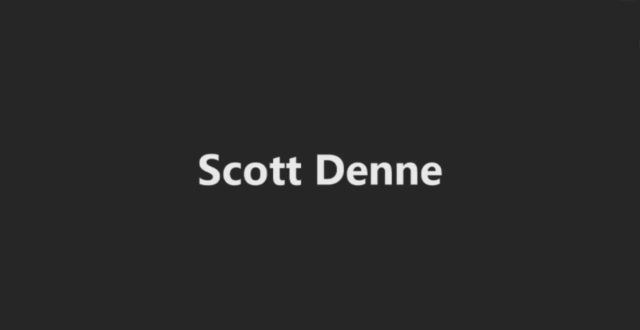 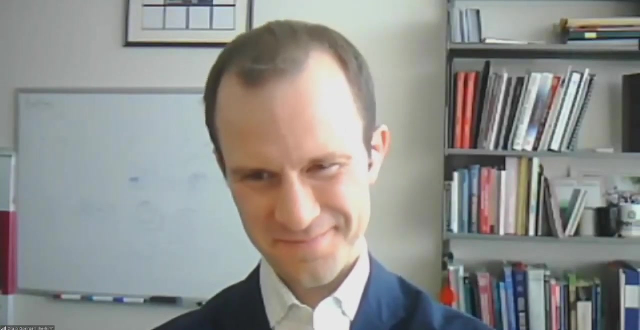 terms of availability for children. So I just wondered if people had any ideas about proper incentives and or mandates- And I know we have lots of industry people here, so mandates is always a dangerous word, but that might help sort of move this along. And again, I understand that. 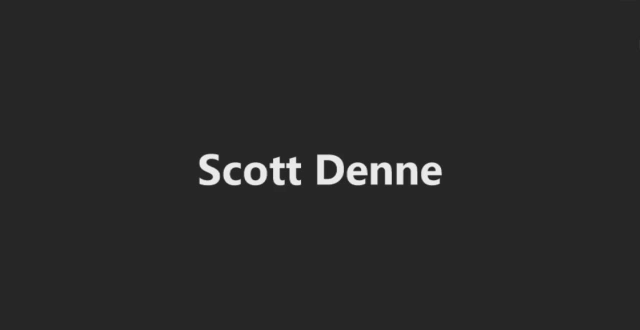 there's very different dynamics between drugs and devices for lots of complicated reasons, but it has been incredibly successful, And one of the things it's been really successful at is now, at least on the drug side, there is consideration of children right from the beginning, which I think makes a huge difference. 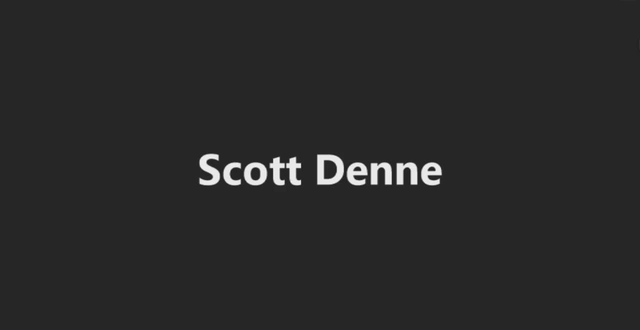 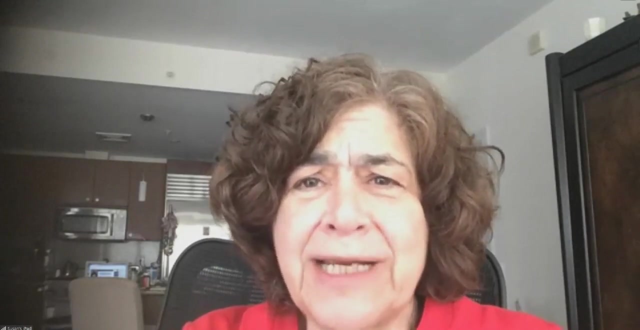 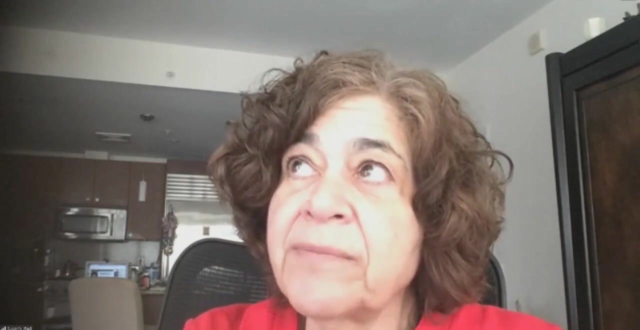 actually, And I think even just conceptually, if that could occur with devices in a consistent way, that could be helpful. I find myself jumping for one quick second and say one of the big differences and one of the reasons why FDA does require that people speak to pediatrics. 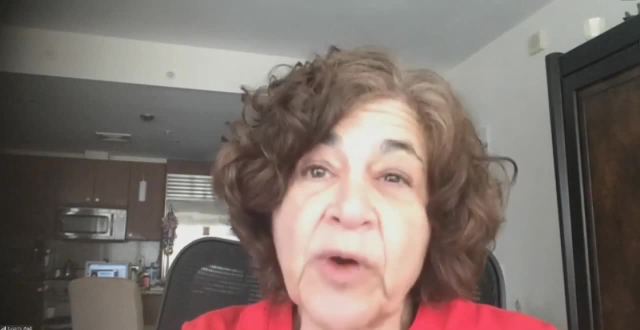 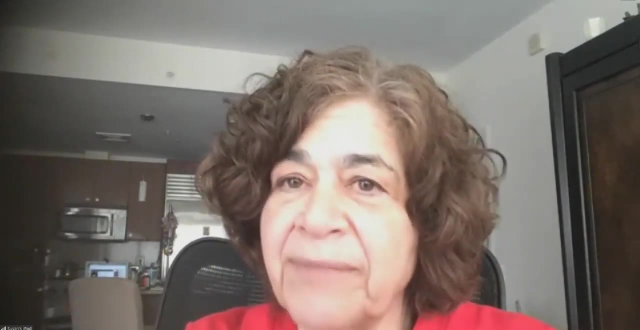 but there's a big difference between devices and drugs And we spoke about it at this panel early on. On the drug side, it's the same chemical, it's the same drug and you may have to make it an oral formulation, You may have to make it juicy and taste good, but that's it On the device side. 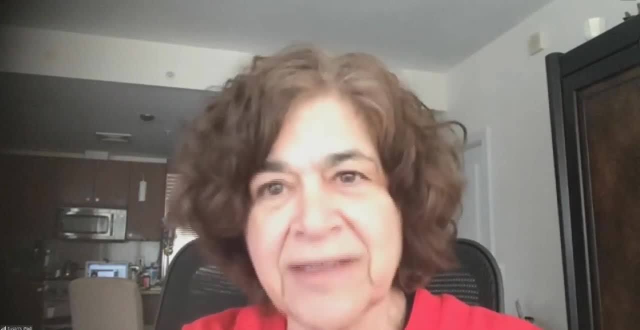 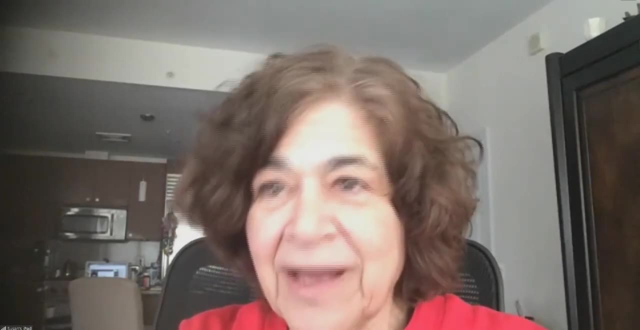 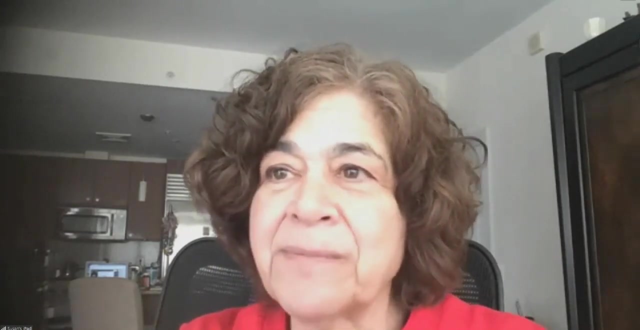 it's frequently a total redesign of the device. It's not the same device And that happens frequently. So mandating that a device for adults be designed for children is not the same mandate at all, And I'm taking that from the device side as well as as a pediatrician. 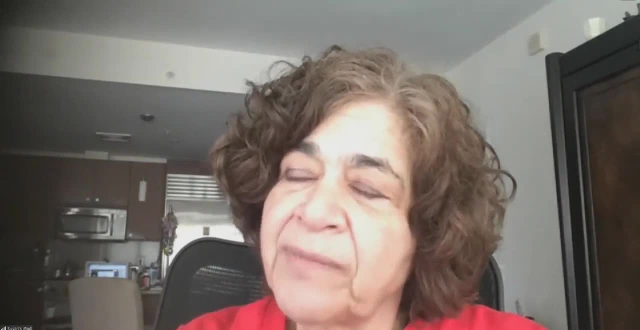 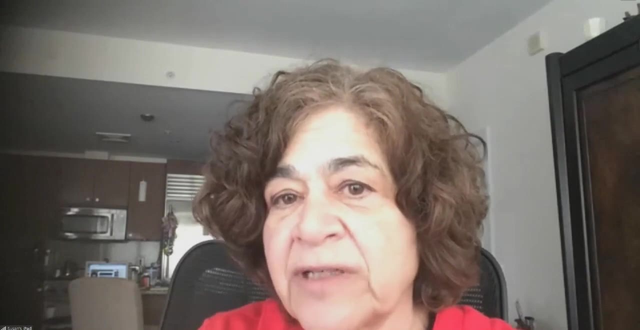 So I think we just need to. we need to. FDA does want and does require that people speak to whether or not a device can in fact be used in pediatrics, but I think we have to be carrying out a research plan as soon as we find a device in the mud market, in the public sector, every month. The reason I like it so much is because it maximizes access to the community, To the community, in particular, стран. I apologize because I don't know if that is enough for some of you guys, but it has also caused some of the values of Pre benettation options. careful around mandates, because this is not at all the same industry. The products are not at all of the same types. The change that would be needed is sometimes a totally different product, totally different materials, totally different design operation. So mandates don't really lend. 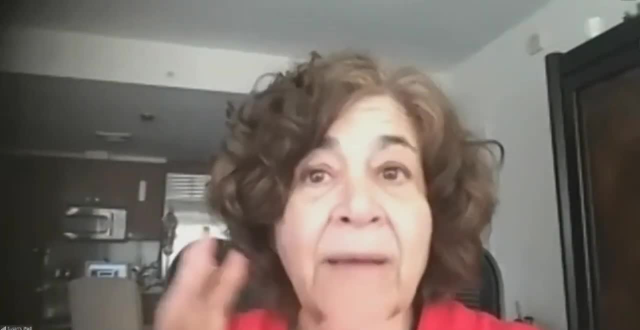 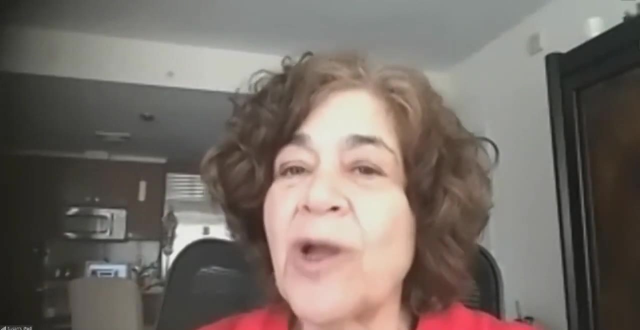 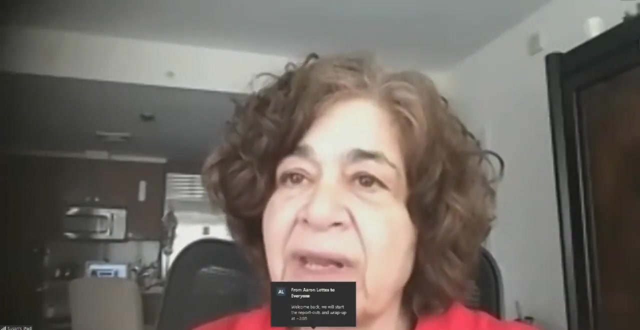 themselves to many areas of devices, But I think, making pediatrics front and center. and if you haven't seen the SHIP- Jeff talked about SHIP- go online and look up SHIP because that's an effort that's going on between FDA and industry and the academic community to facilitate the development. 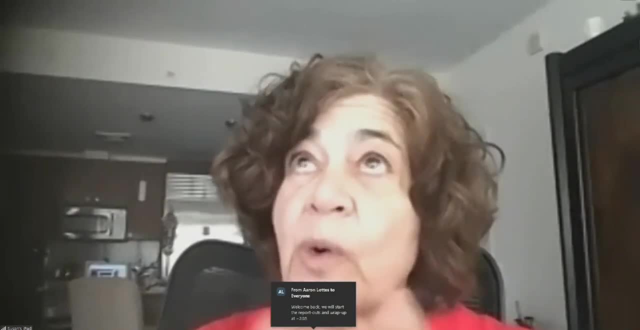 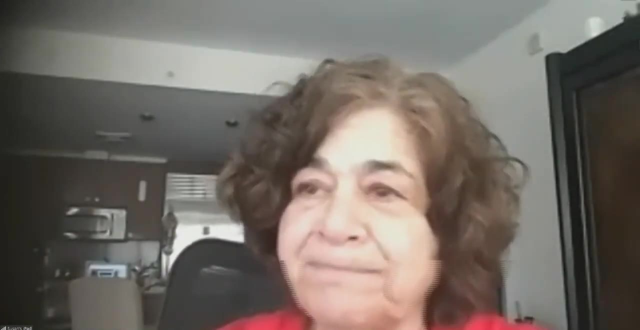 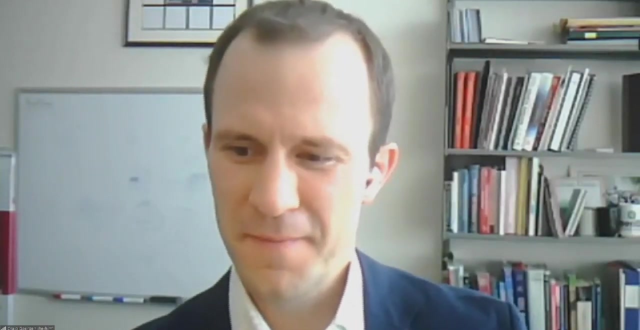 of more devices for children in a much more organized and much more visible and much more supported and collaborative way. Yeah, Any other comments from the panelists? I'll make one more comment, just piggybacking off of what Susan mentioned. I don't know if it's. 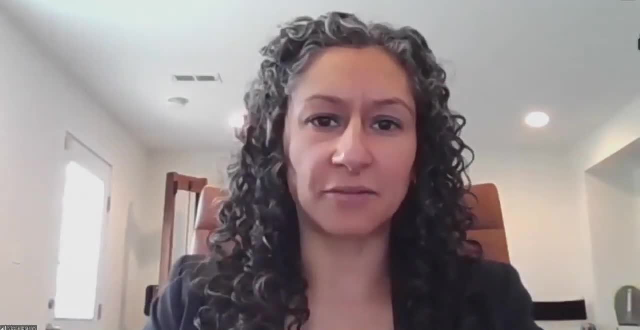 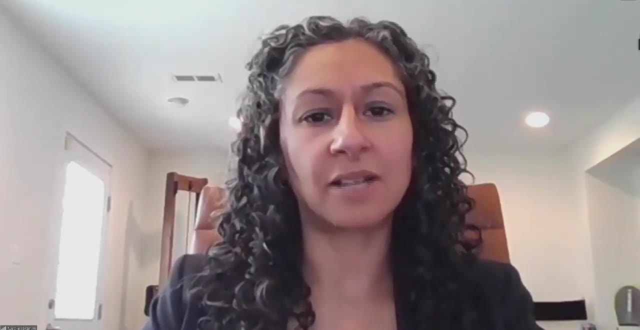 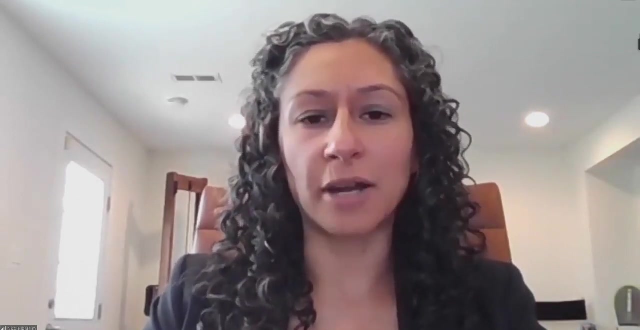 necessarily incentives or mandates, but I think one of the big differences between drugs and devices is one of the things that Dr Devlin mentioned, which is the flexibility in the regulations that we have in devices. There's room to allow for a lot of creativity, I think. 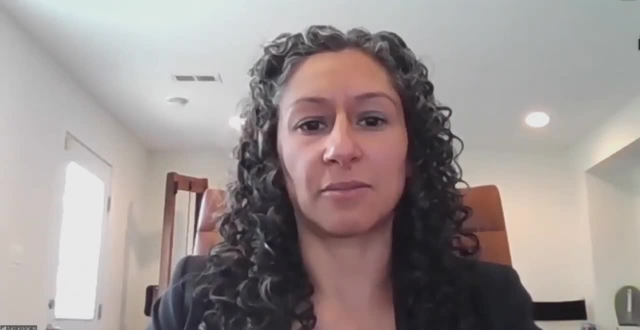 when it comes to, I think there's room to allow for a lot of creativity. but I think there's room to allow for a lot of creativity. but I think there's room to allow for a lot of creativity, I think, when it comes to. 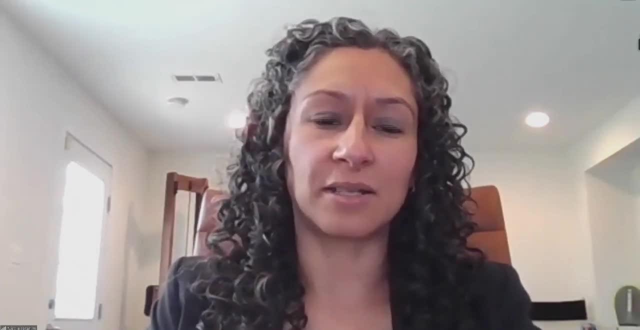 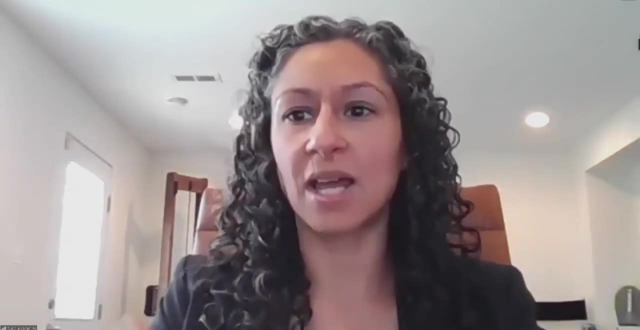 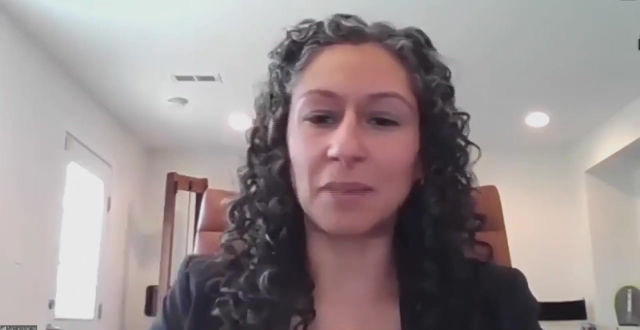 what evidence we would need for marketing, And I think those are the. That's the type of tool. So we have a different set of tools. I think in devices And I think that's where we, That's how. Those are the things that we use, as opposed to the mandates and the incentives on the device side. 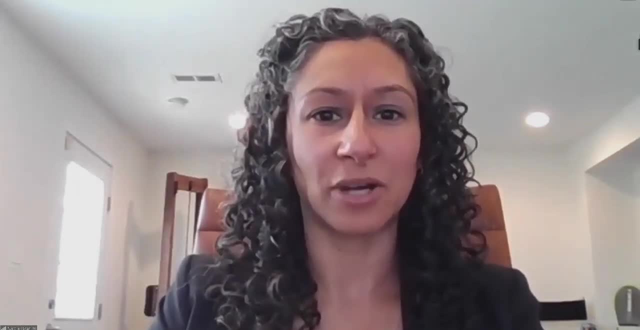 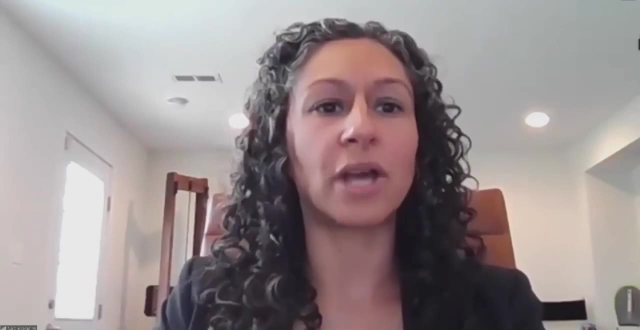 And, you know, maybe they haven't, We haven't been as effective or we haven't been utilizing them quite as well as we could be, But I think, and I'd like to think, that in the last couple of years we've started to utilize different. 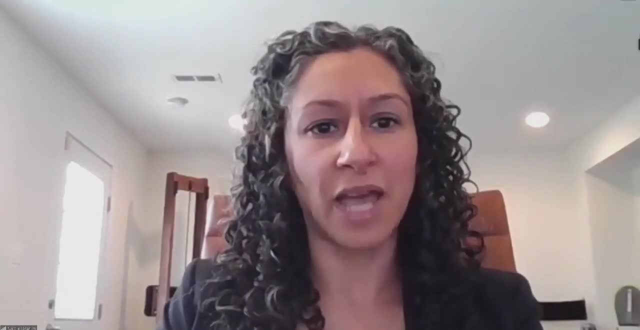 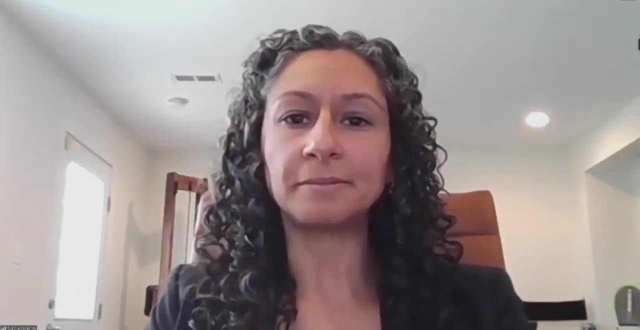 tools in different ways, using the flexibility that we have in our regulations to be able to push things and move things forward. for pediatric devices Agreed. That's a great way. to wrap up, I just want to thank the panelists again for their time and insights. 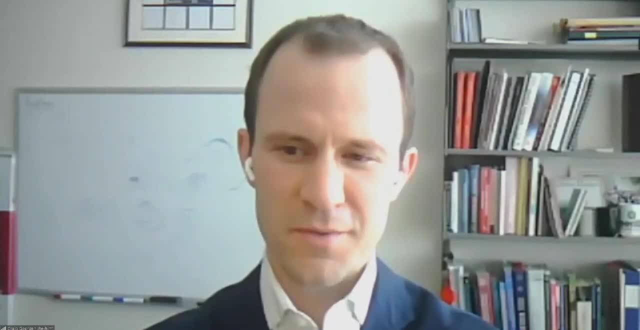 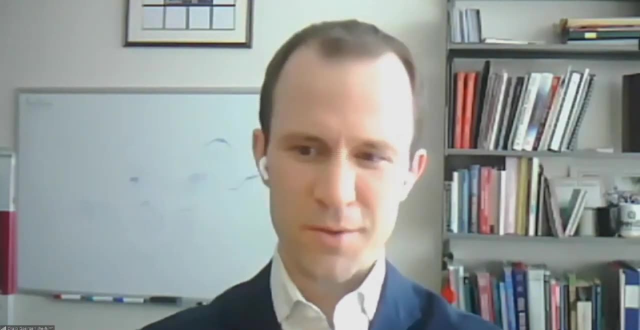 It was great to see all the different case studies And I really appreciate everybody in attendance for the discussion as well. It was wonderful questions And I think there's a lot of momentum for the of momentum for pediatric efforts, not only at Purdue here, but also across the state and through. 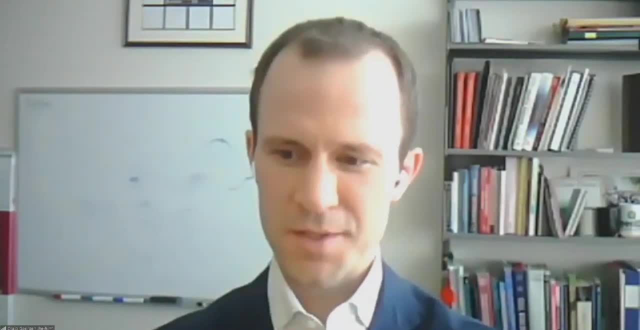 the CTSI mechanism, So we'll be following up. There's going to be a summary right after this. We've got just a few minutes for break and then Dr Lattice will be running a quick summary that will summarize all the breakout sessions. So stay tuned for that, and thank you again, panelists and 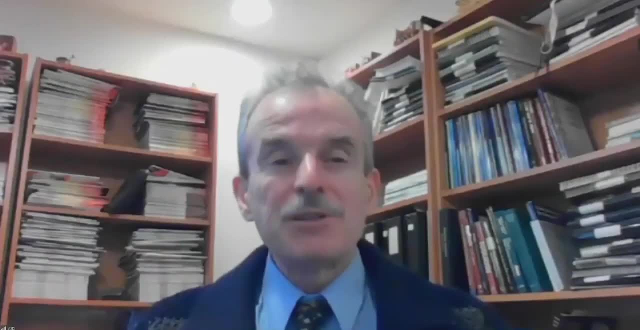 everybody that's participated, Thank you. Thank you, It's been a pleasure, Thank you.